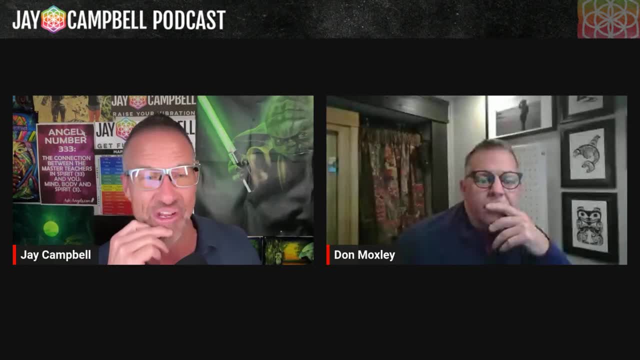 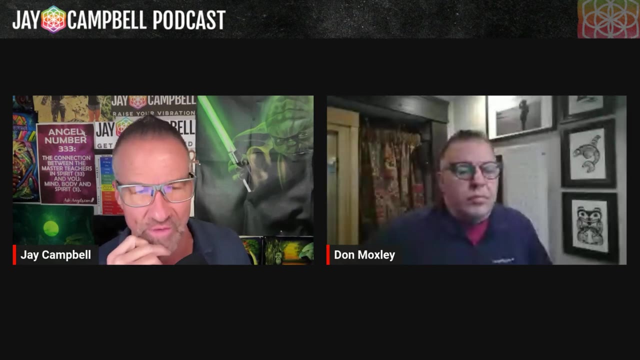 Science at Longevity Labs and also the developer of HRV Plus from Mode and Method. And also Don has an illustrious background. I would say just the sports performance and the college side of things, Don. actually we don't know each other formally but I know of you and have known of you from a lot of different. 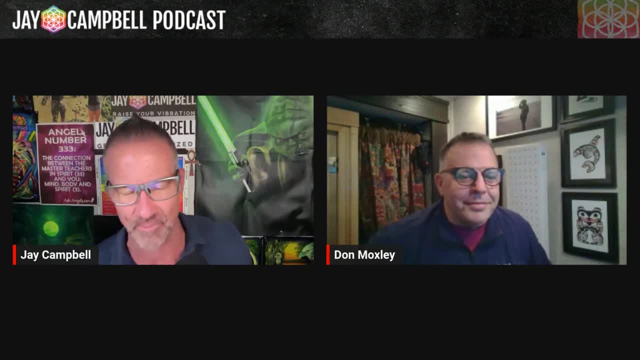 people. We have a lot of similar friends and colleagues Before we jump into it, because we had a bunch of different points we're going to talk about today. but why don't you just talk a little bit about traveling across the country in a fifth wheel? 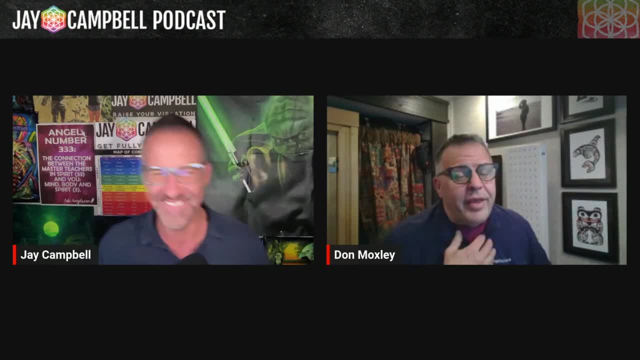 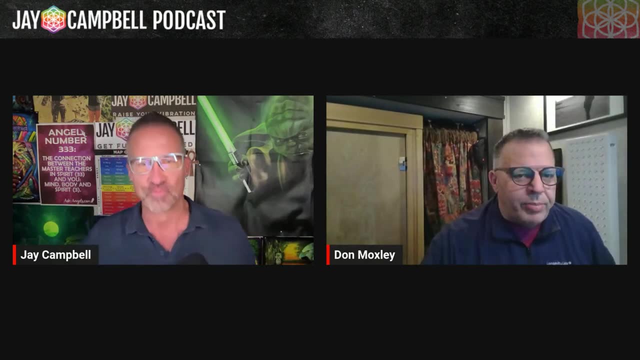 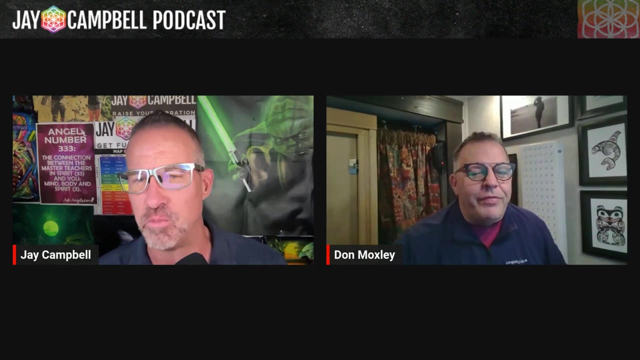 Well now listen, it is not a sacrifice. If you'll look over my right shoulder here, that's my sauna that I put in my fifth wheel. That's awesome. So we've got a red light therapy panel in my office. We've done it in a way that we're able 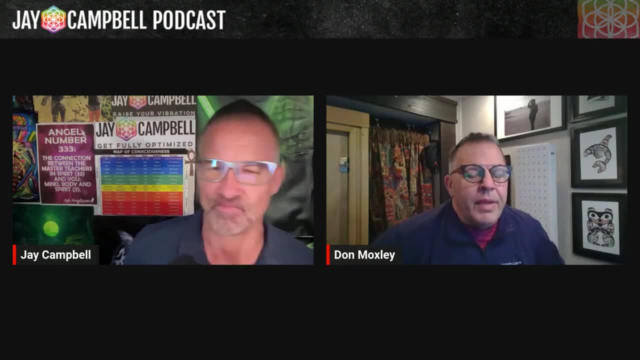 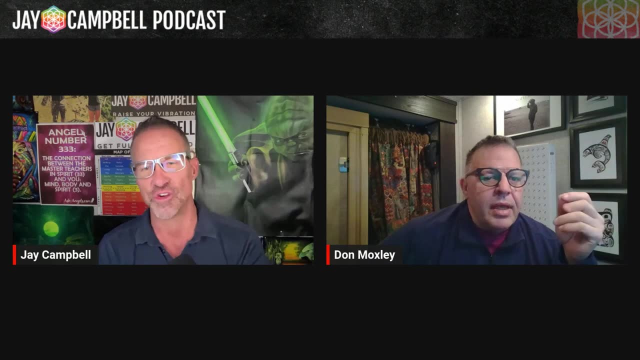 to. I've got a Peloton bike, I've got all my strength stuff. But I work for a company called Longevity Labs And you start talking about longevity and I think of life in three-thirds that you spend your first. 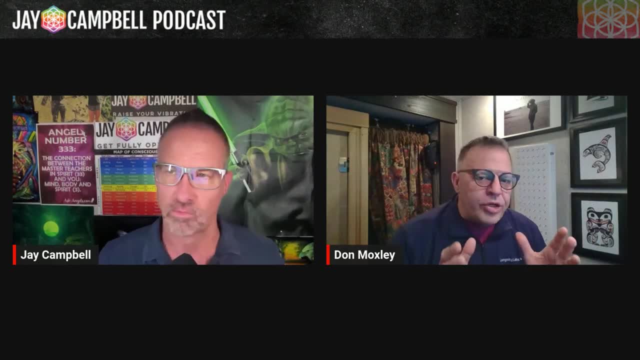 First third- learning- And then you spend your second third earning in service to others, meaning that you're working, you're raising a family, you're doing things like that. But then you have what's called the third third And my daughter. my wife and I have one daughter. 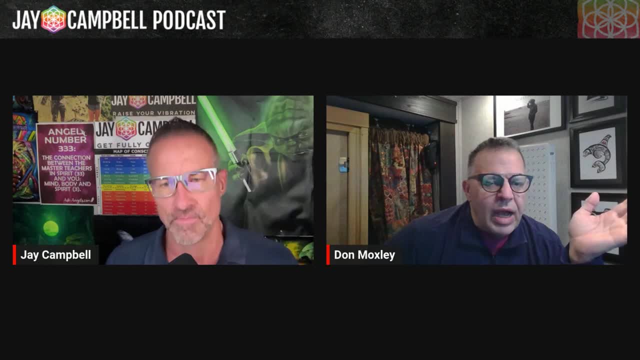 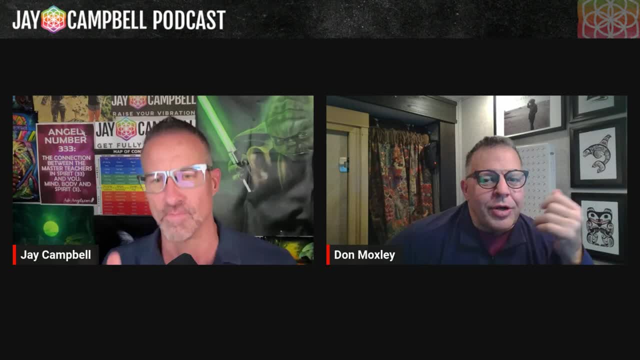 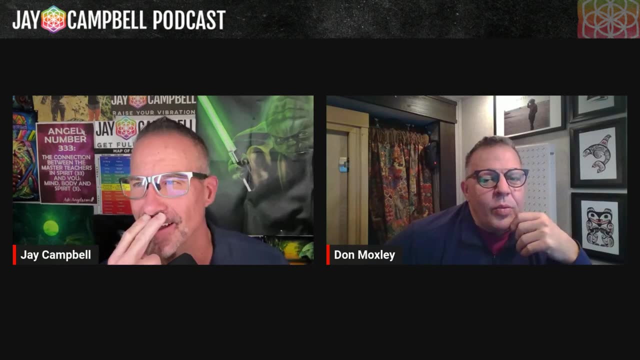 And I said she went and got a job at North Coaching at Northwestern And she's not coming back. I mean we're done. And we have always liked the mountains And I said I want to find a place where we can wake up in the morning and drink our coffee looking at mountains. So we thought about: 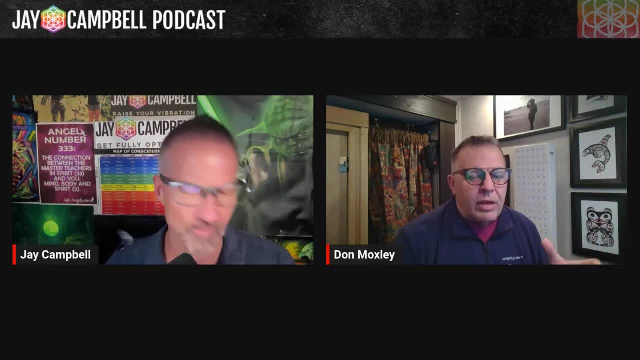 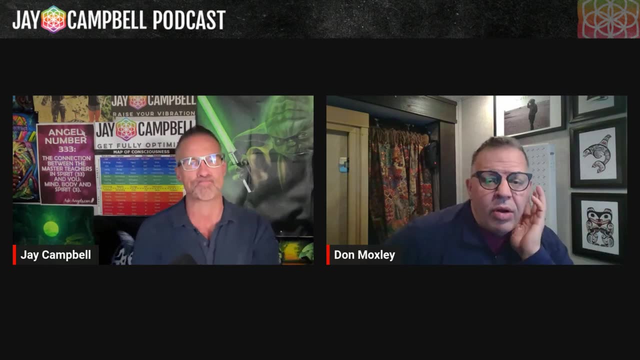 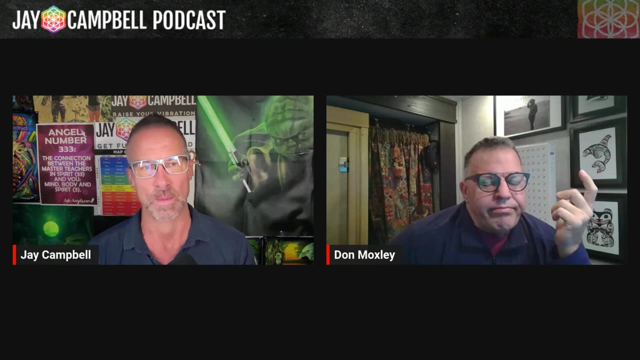 Colorado, And we spent a month and a half in Colorado last year, worked our way through Wyoming and Montana and all the way across Sure And back and forth across the country. We're now on our third trip back and forth, But we're waiting for the universe to give us our next home. 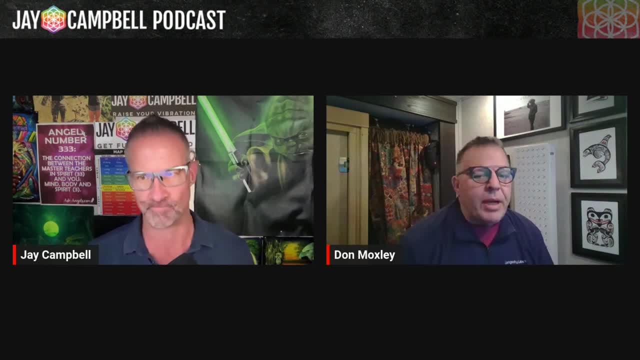 And we're taking it in. And we just spent six months in the Pacific Northwest, Oregon and Washington. We really like it there, But my kid's now coaching at Pitt So we decided to come back across So we can watch her work. You know it's not. you know you don't always get to go to work and 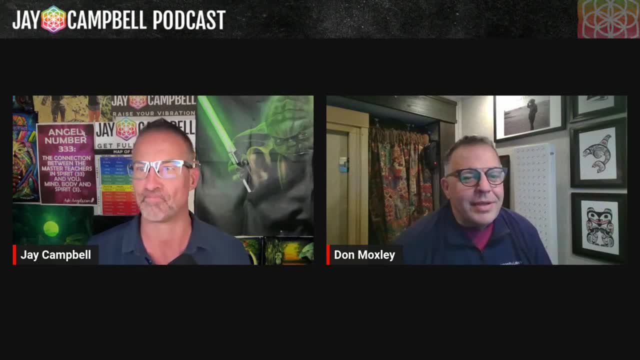 watch your kids work, right? Yeah, that's amazing, dude, And so yeah. so that's, that's our life And we're probably so we're back in Pitts. We'll be in Pittsburgh for a couple of months, Then I think we're going to go to New England. 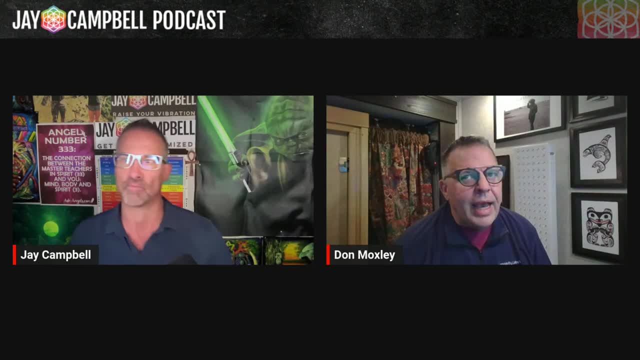 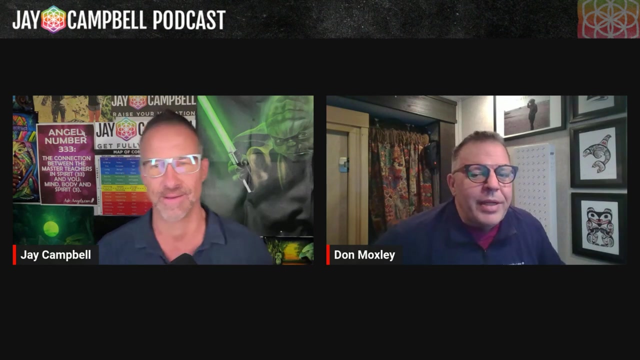 And if we get New England in, we will have 45 of the 48 states in. I think we'll be missing Kansas. but what will we miss? We'll be missing Kansas and possibly, like Tennessee, Kentucky, which I've been to- We just haven't stayed there in the rig- but of the lower 48, it's, it's been, it's been. 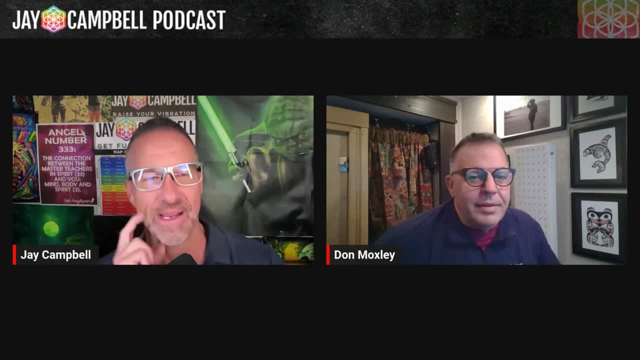 pretty cool And that's awesome, man. And you know we've got all your biohacking tools built into the rig. I love that, So so we. so we've got, like I said, red light. red light's a big. 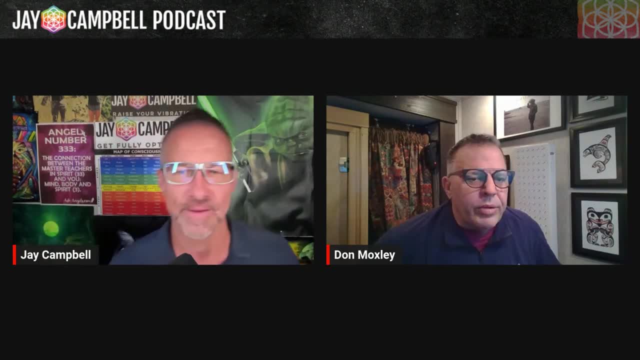 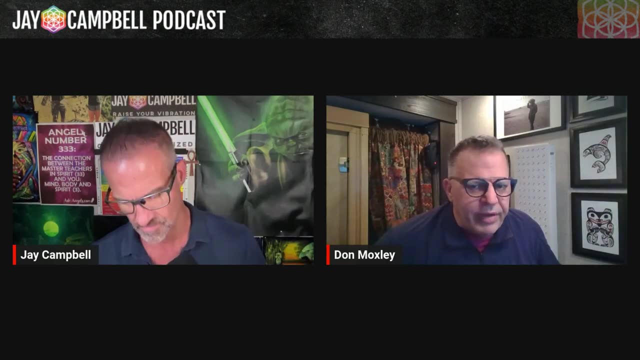 deal. You know, before we started recording, we were talking about light and heat and environments and so forth, And and I talked, I talked about my four big rocks of longevity and performance. You know, if you the the seven, 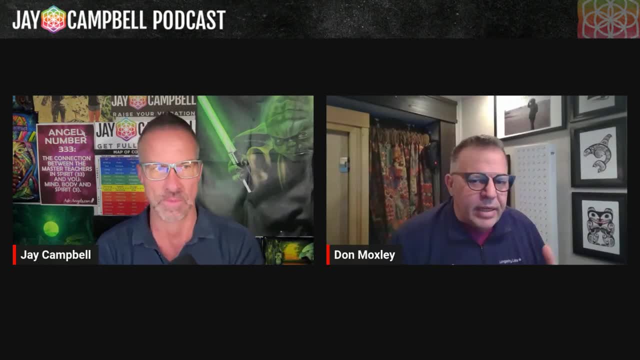 habits of highly effective people they talk about. there's a piece in there where they talk about putting rocks in the jar. that you know, you put the big rocks in, you got to get to gravel and around that and you get sand and water. but you got to get the big rocks in the jar first. 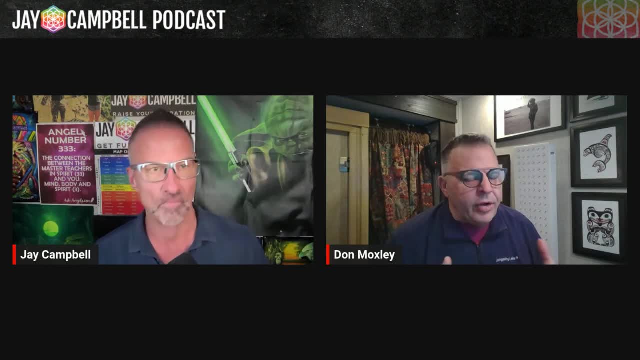 And in biohacking there can be a lot of sand and gravel. And if you fill your jar with sand and gravel before you go, you're going to get a lot of sand and gravel. And if you fill your jar before you get your big rocks in, you don't get the critical stuff. And and my four big rocks are: 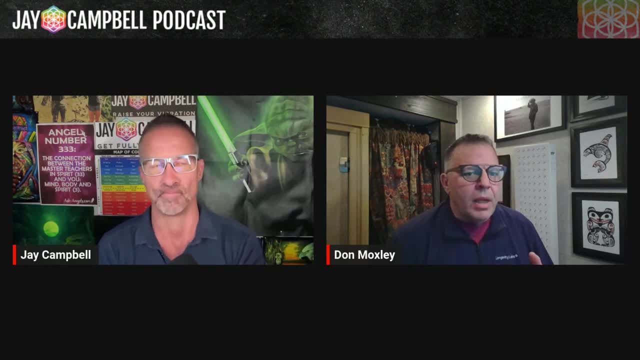 movement that you hack with exercise. uh, nutrient dense food that you hack with supplements. sleep, You don't. you don't hack sleep, You hack the sleep environment. Um but um, and then finally light. I think light is. light is as important a rock in the longevity and performance. 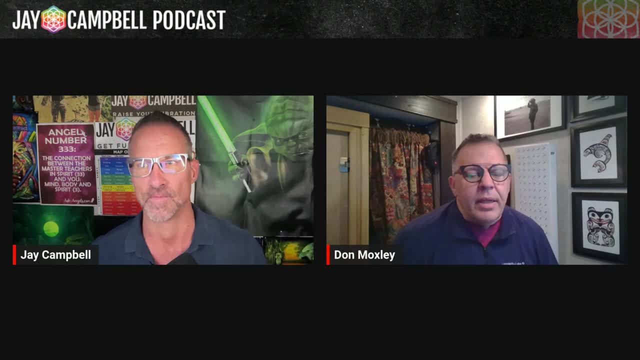 jar as anything. So, um, I started looking at light. you know, when I was a sports scientist at Ohio state- 15 through 18, we had a. we were working with the air force research lab out at Wright Patterson air force. 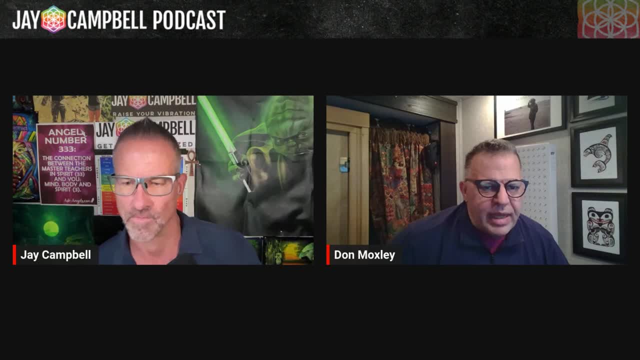 base And they brought us this thing called a Nova Thor table, which is this huge red, $160,000 red light table, And we and one of my, one of my national champions, um tour uh, an ACL wrestling in the Olympic trials. This would have been 17, um. 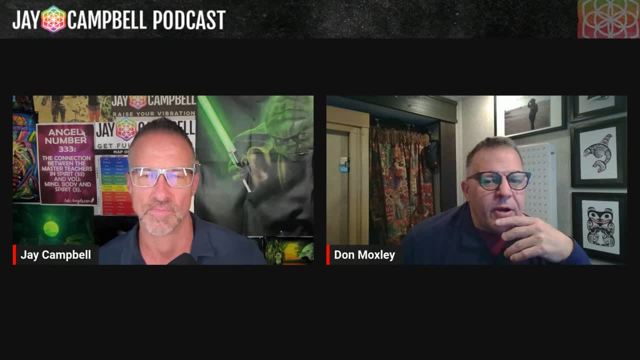 born ACL, And so we're trying to get this kid back for a senior year And I walk him into this, this red light table, and he goes in on crutches. I put him in there for 20 minutes, I take him out. 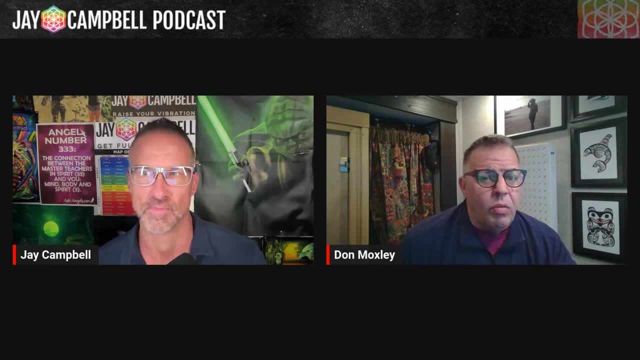 and he walks out with his crutches on his shoulder And I'm like Whoa what? what is going on here? And that's what got me looking at the quality of light. So I've invested in it a couple of times. I've got- I've got good friends down in Florida. They're over in Fort Lauderdale. 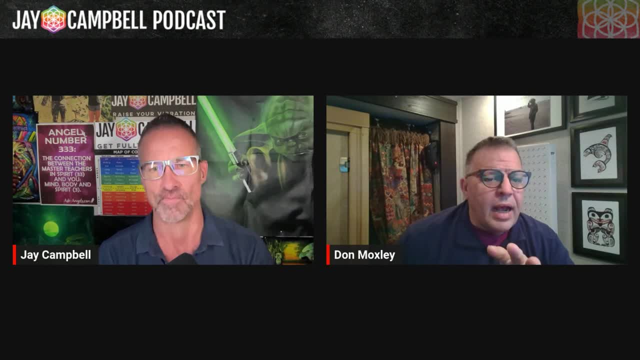 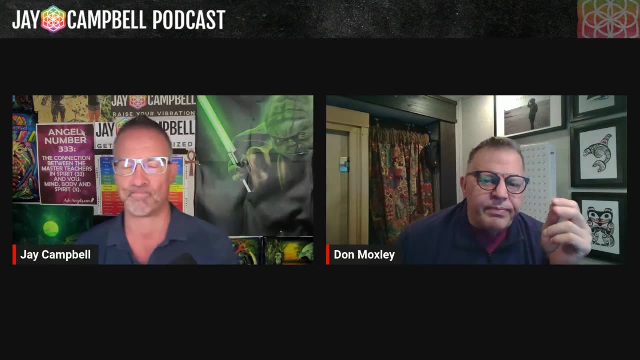 Uh, they've got a company called Therasage that I really like, Um, they do red light panels. I've got a red light panel hanging in here behind me, Um, but getting that getting lit. you know what, Jay, we don't die when we run out of time. 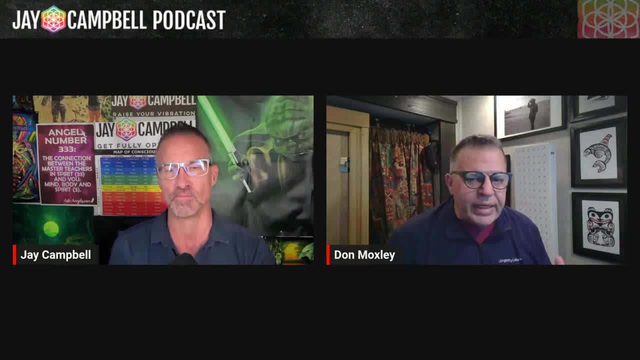 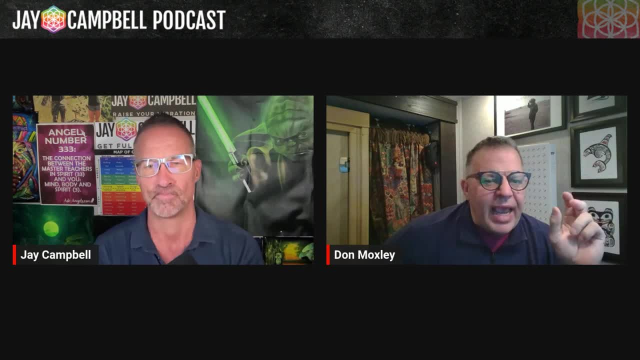 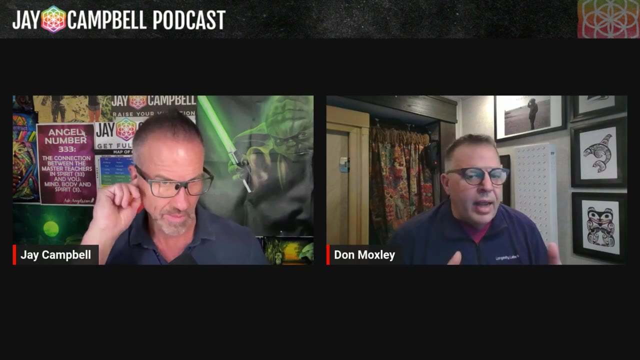 pay attention to this. Now, I don't. I don't think we have a handle on things like light therapy, cold therapy. I don't think we have a handle, Like we do, exercise and sauna. um, exercise and sauna. We can prescribe very effectively: Um and and and, but you know these other things. 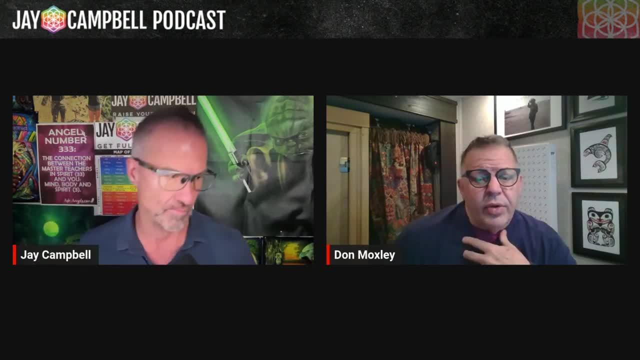 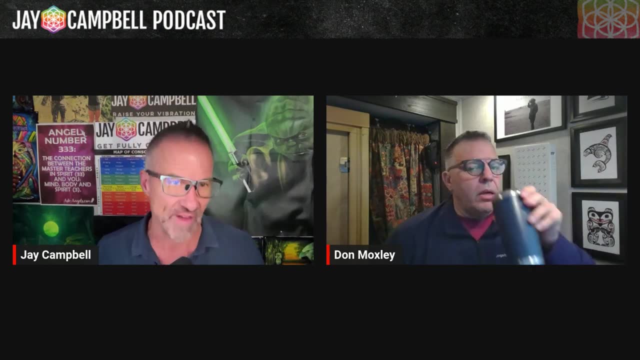 are emerging, We're starting to understand them, but I think light is a critical tool. Well, I'm a huge proponent of red light therapy. I mean, we just wrote a 9,000 word article on it. Uh, I use the perfect. 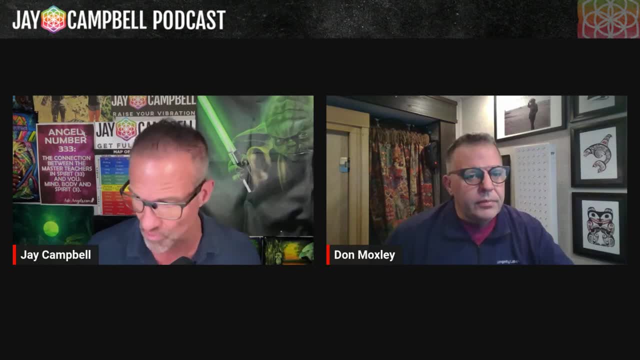 the trifecta pro four 50 bed. you know which is a $75,000 red light device every single day? Yeah, So is my wife. So is my daughter, who's uh 15, about to turn 16 years in performance, cheer. 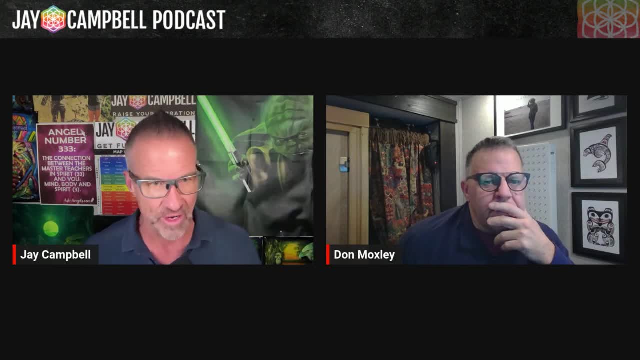 Uh and yeah, I mean, you know the photonic quality of your infrared light and red light at specific wavelengths. The problem is, Don, is that unfortunately- and I again, I wrote about this and also did a podcast when I interviewed- 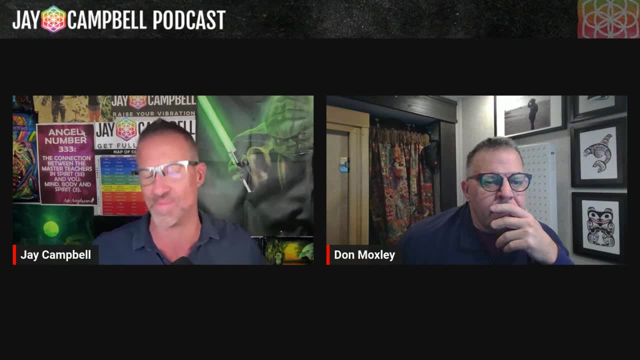 really the father of red light, Dr Carl Rothschild. you know who's been, the guy who's done all the research in the West 25 years, And of course it's his company that I am uh promoting now. uh, trifecta, but um. 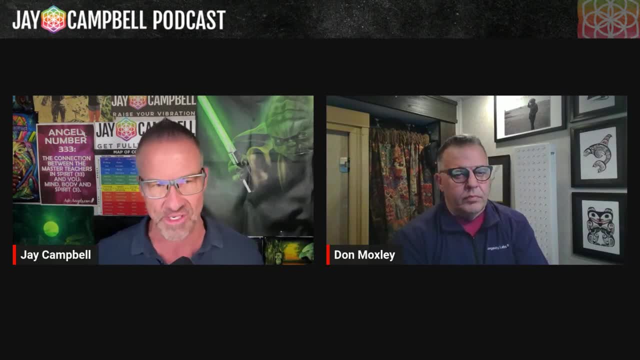 you're right What you said. I mean we don't understand it at the level that we understand other modalities and other things. And again, it's really just experiential. You like you can talk to 10 different people that manufacture red light technology devices and they'll all give you. 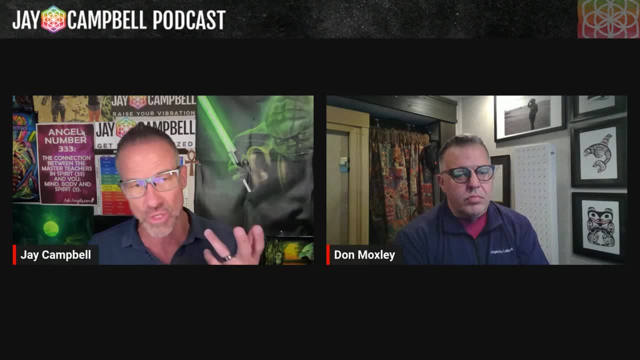 10 different answers. I'm like: what is the right therapeutic dosage? Now we do know that from an infrared light standpoint or near infrared light standpoint, that's the- those are the quality or the wavelengths on the frequency that will heal Right. So for people that have autoimmune diseases, 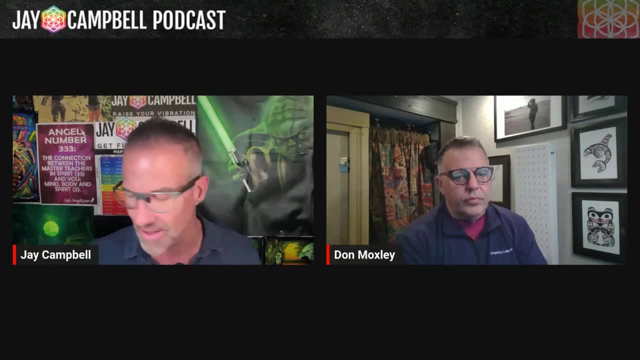 uh and obviously other forms of uh decay, uh advanced tissue regeneration and stuff like that, even uh neuro neurodegenerative disorders. that eats the near infrared light, where it's the red light frequency and wave light that uh, you know, ultimately improves cellular health. 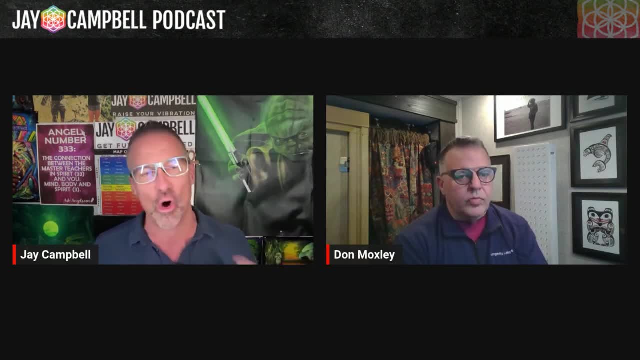 It creates fat loss, uh, enhances mitosis, It does you know all these different things. obviously optimizes mitochondria- You were just talking about that. but, um, I'm a huge, huge proponent of red light. In fact, all my friends that have. 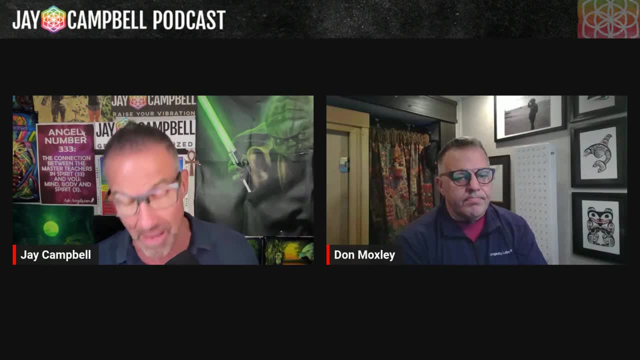 uh resources. I tell them you need to put a really high power, what I call high power, medical grade red light uh product in your home. And obviously you know, without getting into a competition thing, of some of there's you know, five, six, seven, eight, nine, you know. 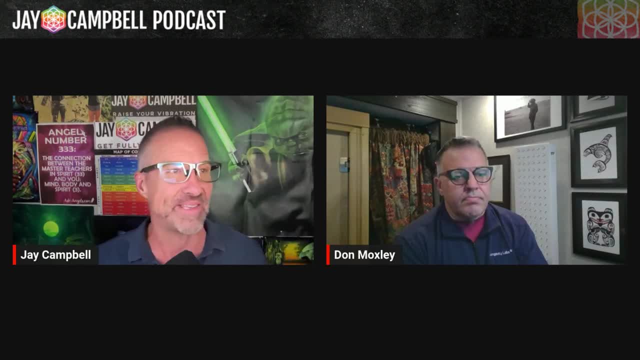 companies out there now that are all. problem is, though, is that, you know, five to seven years ago- And again I won't name names, but I could- uh, a lot of the red light companies- we're putting out products that were not. let's just put it at the level necessary to really 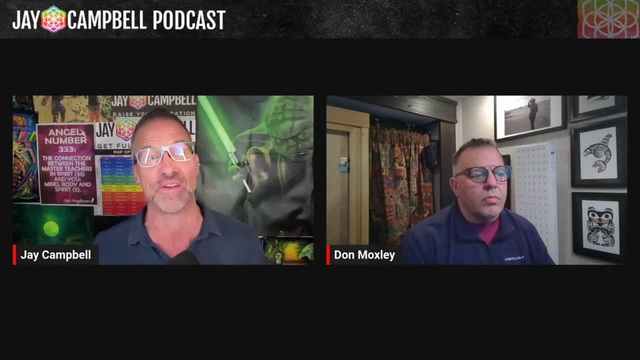 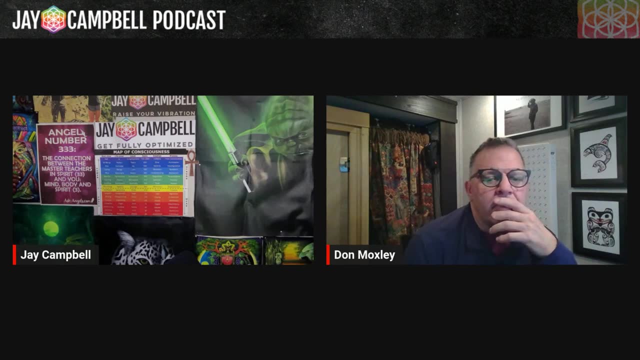 truly bathe yourselves in the light that is necessary to actually provide all these different effects and benefits. And again, you know either you probably already books. This is the newest one calls illuminated healing, and it's an amazing book And, as a lot of research, one of the things 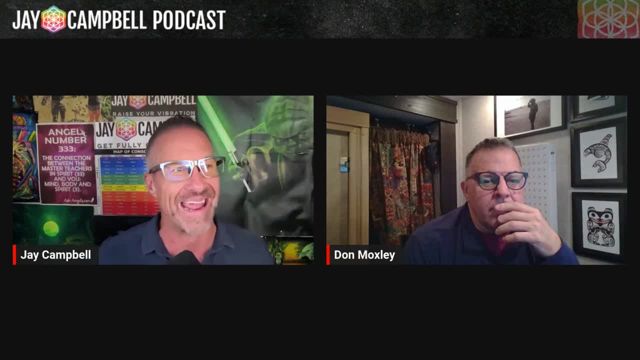 I didn't know about red light, Don was uh. it also enhances um the microbiome's ability to upregulate, uh. Acromantia mucilis, which, as you know, if you can, you know, cleanse the microbiome. and improve the strength of the microbiome, you're going to be pretty strongly protected, If not impervious. many of the diseases- right Cause, almost all disease- ideology originates in the gut. Yep, And a lot of people don't know that. Yep, But I'm down, I'm down. That's awesome. 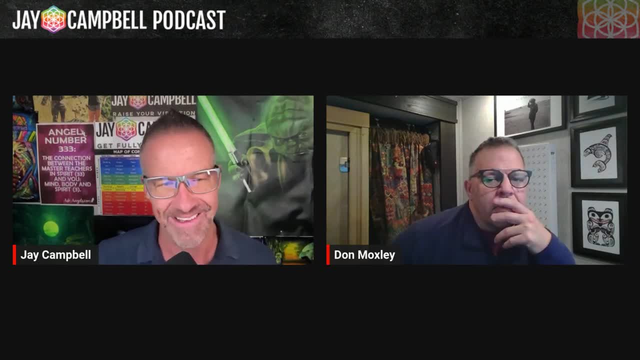 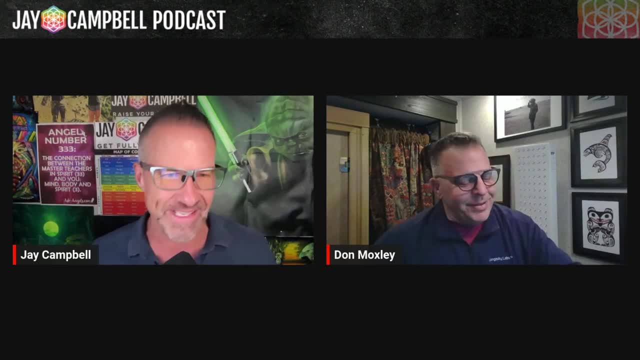 age of 25, doesn't even know who Stephen Covey is. Doesn't know what. the seven habits of highly effective people- True story. I met Stephen uh when I worked for Kelly blue book before I became whatever. I am now online gypsy Uh and, and he is an amazing human being but arguably one of 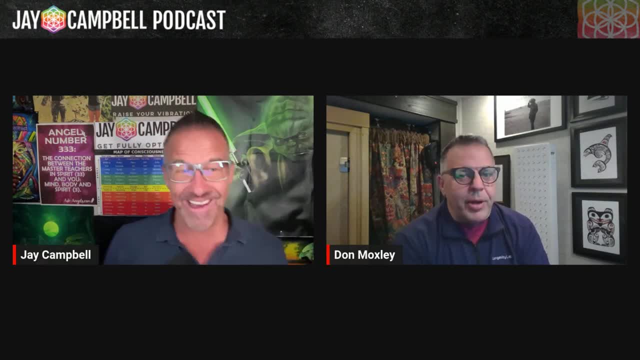 the best books ever written. I mean, if you're in business, you should read this book. If you don't know what Stephen Covey is, you should read it. I mean, I met him in 2000,. it was either 2005. 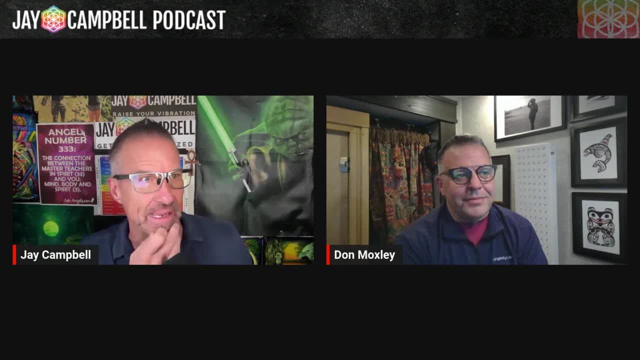 or 2004 and he died literally like eight or nine years later, but like he was still in his sixties, a very powerful speaker, Yeah, Like he had an aura and a presence about him. but that's so cool that you brought that up, Cause I was, like he just said, the seven habits of highly effective people. 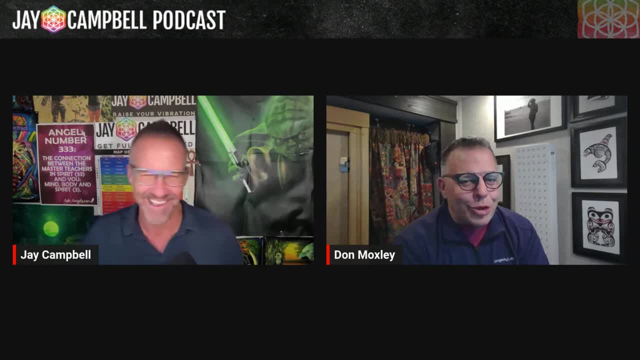 If I'm anything, I'm a pretty ferocious consumer of of written material, I, but I've now shifted over to listening more than reading directly. But, um, but I, and, and as if, if you, it's. 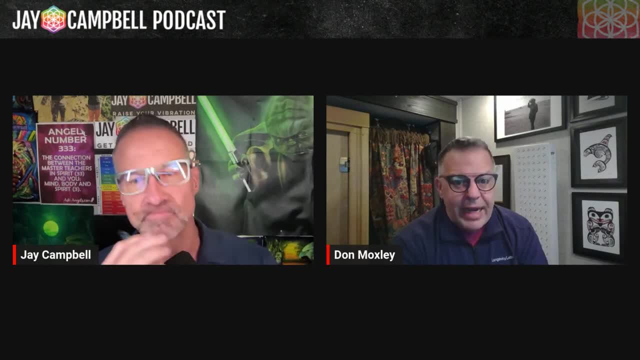 if you can just take one little thing, listen. I love seven habits There's. there's eight things in that book that can drive you. his next book, The eighth habit, is also is very good, Um, but yeah, it's, it's one of the, it's a guide, It's a success guide, Um, when it comes right down to. 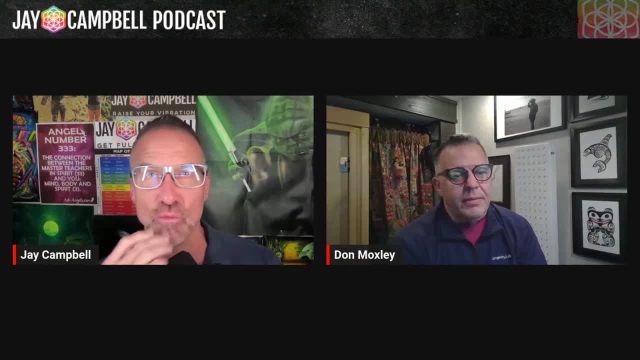 it. I mean what totally you just said? I love that reading, I mean the whole thirds thing, but reading Is essential because reading creates awareness, and then the awareness is usually coming from your experiential body of work, right? Well, so, whatever it is you do, whatever it is your trade, 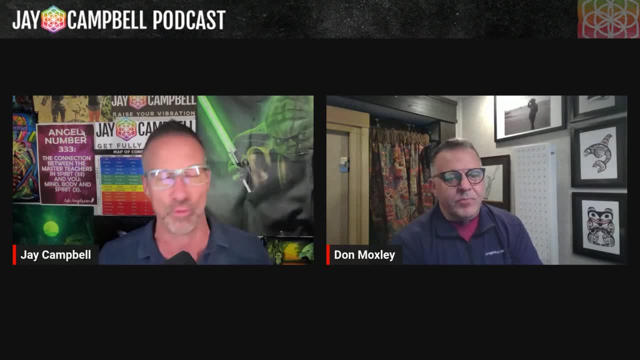 I mean even. it's like traveling right, Like traveling around the world, experiencing different people, different cultures, different- uh uh- languages. you know spiritual beliefs and inclinations. all that stuff creates awareness And it's like you know before we jump into. 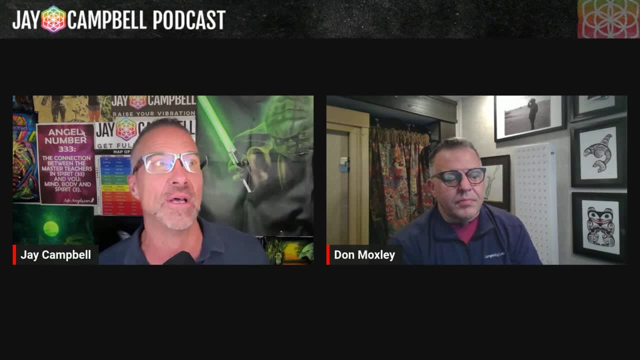 your topics, the saddest part of today, And I know you know this, um, because you've worked in the education realm. kids don't read and it's insane how bad it's gotten that even the schools are not even asking. 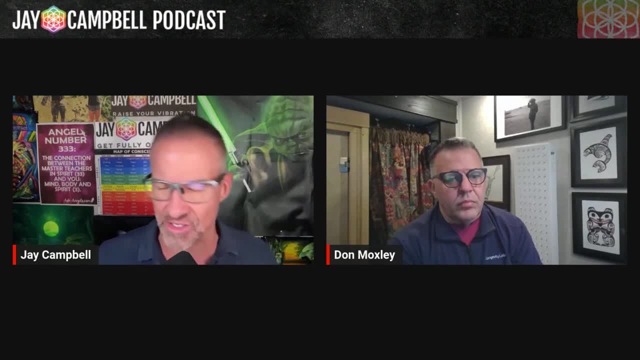 children, uh, depending on where you're at, you know, and I know there's private schools out there and homeschooling and all this stuff, but like the curriculum is degenerated to a point where they don't even read the classic literature pieces anymore. It's unreal Really. Yeah, It's a. 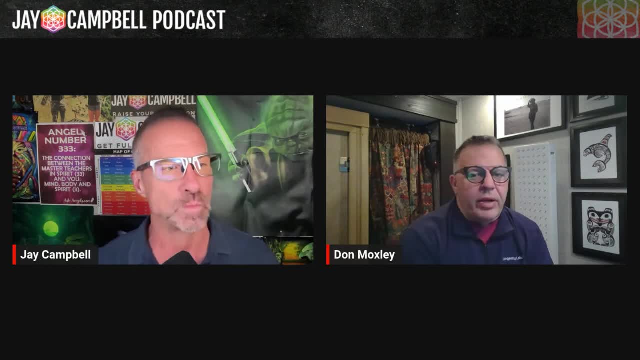 challenge And and listen. I I don't, I don't depend on the schools to raise my kid, That's for sure. That was, that was on my wife and I, and luckily I'm married to an educator, Um, and who was. 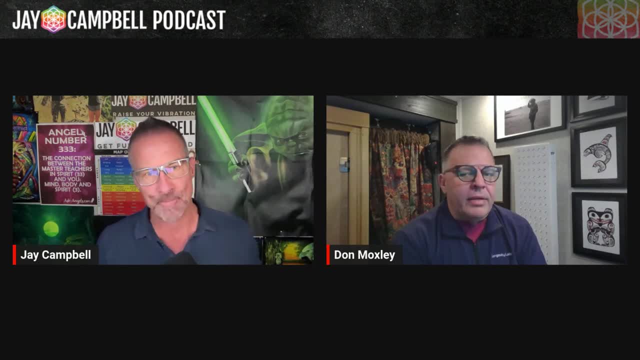 who was very good at what she did, Um, and our daughter benefited from that. She grew up at a house with two teachers, Um, and, and she's a pretty sharp kid now. but that that's all part of it, And she's a pretty, but I don't depend on the school for that. Now I tell you, we made a 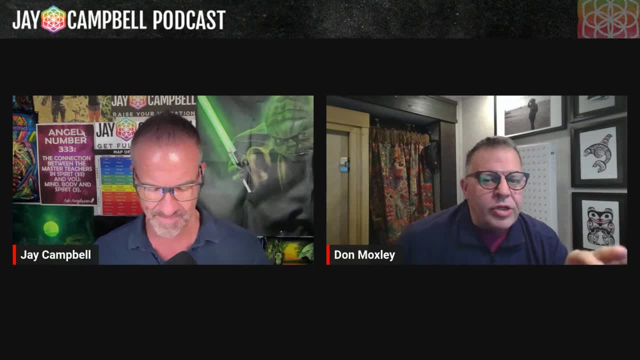 decision When she was born, that we changed, we moved. we at least live in downtown Columbus, a little little part of Columbus called German village, which was a great place to live when you're single. when you're when you're single or married- young married couple- um restaurants. 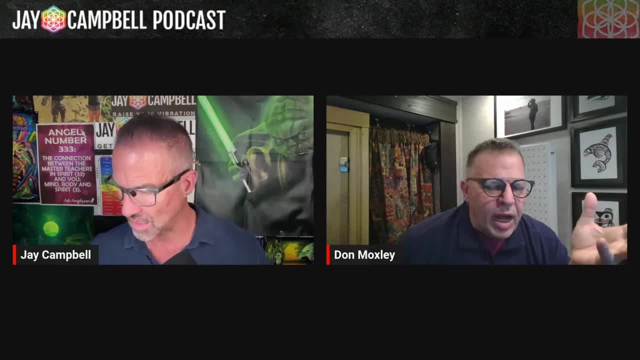 are good, The nightclubs, I mean just the whole downtown life. But as soon as our daughter was born, I said: nah, I'm not raising a kid here And I don't, I'm not sending a kid to set, uh. 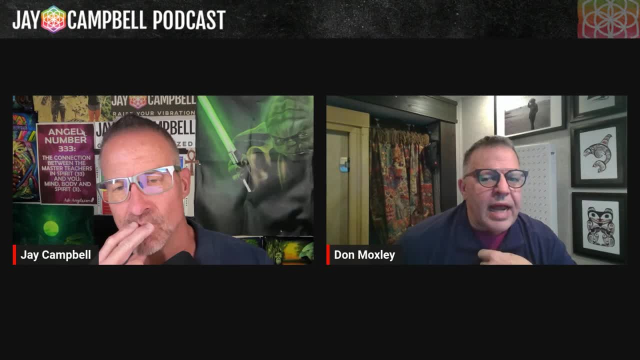 inner city schools And luckily I had the resources that I was able to sell a house and move into another village. And I was able to sell a house and move into another village And I was able to raise my kid in a community that supported our beliefs And and and those I think I mean. 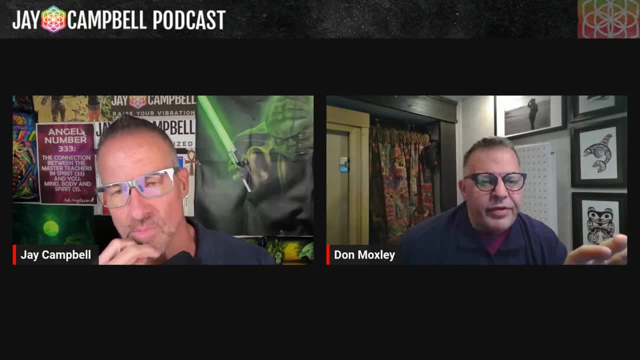 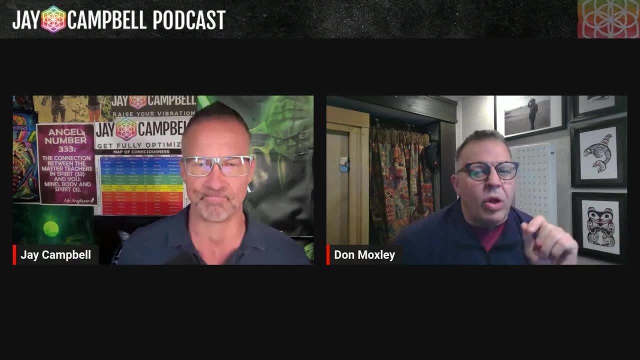 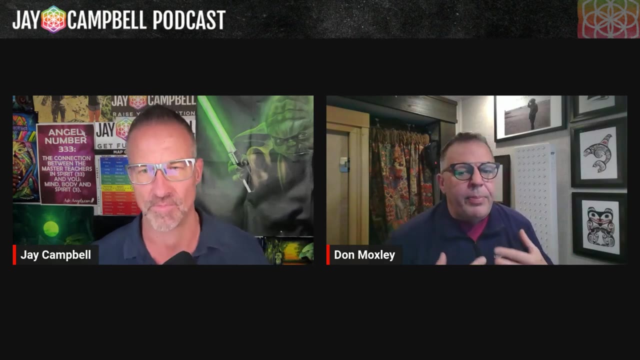 she's a very good writer, She's a. you know the Granville schools did a very good job of that, Um. so you know that's that. those are parenting decisions that you have to make along the way, And, and, Jay, you know not to go too far off topic. Part of the challenge is: is that people 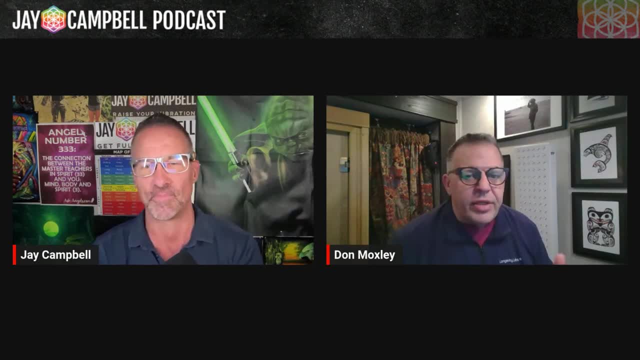 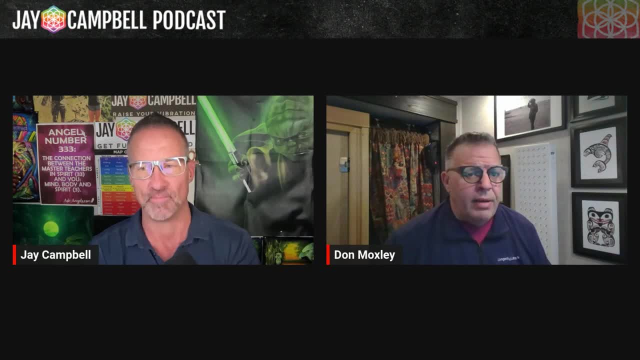 that that, that's that. that's the wrong attitude. Um, you know, I, I, I have a. I feel I have a huge responsibility, the same way my parents provided me. Now listen, I grew up in. 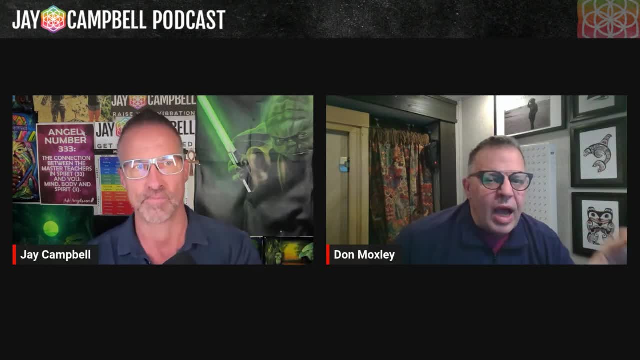 a small country school, but I had two parents that taught us that we were limitless. Um, we can do anything we want to do, And, and that's a, that's a, that's something I wanted my kid to learn, Um, so you know, it's that, it's that responsibility, Listen. 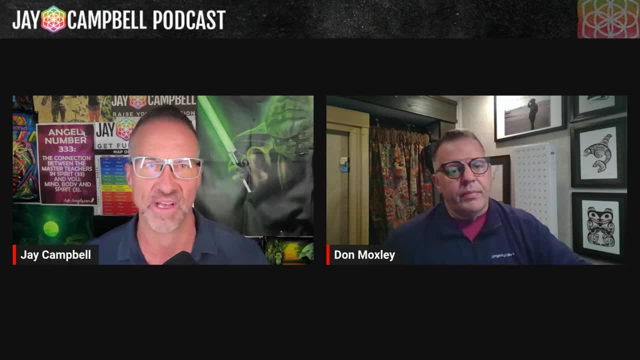 we made them, we're going to raise them And you got a responsibility there. A hundred percent, I, I, I, I couldn't, I, I, I agree a hundred percent. I mean I don't know how I could even disagree with any of that. I mean it's definitely the parent's responsibility. 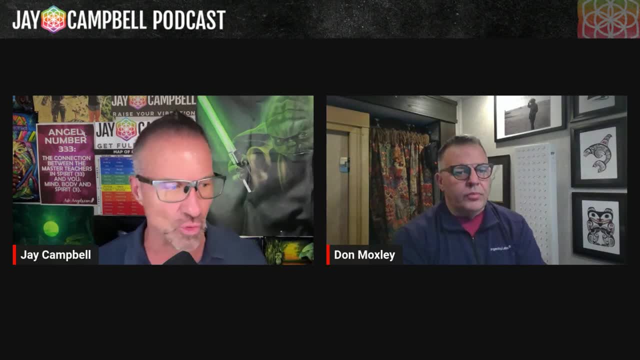 to make sure that your children are educated outside of school. Um it just I don't know It just it's mind blowing to see the difference in just 20 years in the school system as far as the curriculum and the way things go and stuff like that. Now it seems like they really just 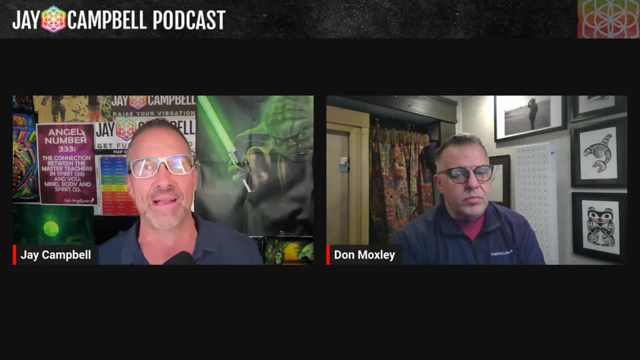 overburden them with like busy stuff and that the kids really are not getting. you know the what I would call the experiential body of of work that you and I got Cause again and again. things are different, right, Because when you and I grew up we didn't have technology. 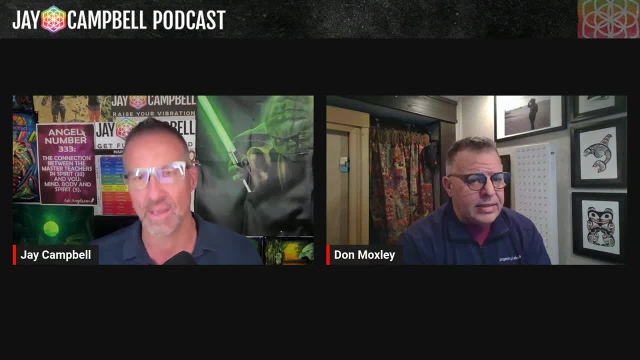 So we didn't have, we had very little standardized testing. Yes, Um, and and I think- and now listen, we can do another entire podcast on this- but, um, but it's, it's the the role of standardized. 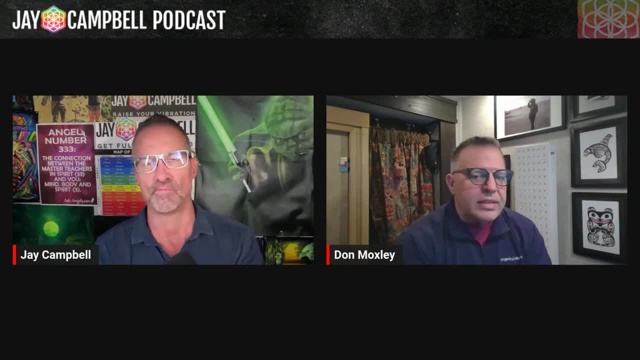 testing My wife. my wife was a science teacher, social studies and science teacher And one of the things that just frustrated her to no end that by the time they took the standardized tests for science, that was the eighth standardized test Those kids had taken in the last month of school. 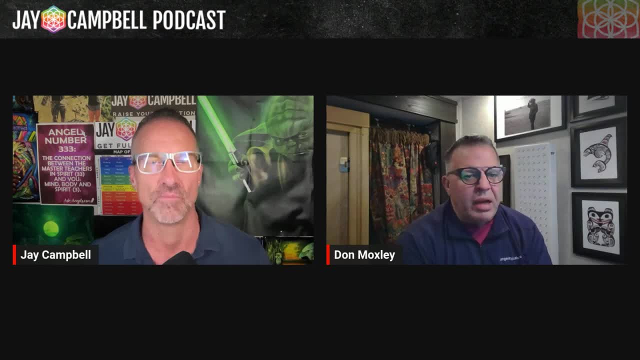 Yeah, She said yeah, she realized they were checked out. you know they were done, Um, and then the school wanted to base her pay on the performance of the. these kids tests And and it just the the. we're in a situation where technology's changed everything. Okay, Our kid, you know. 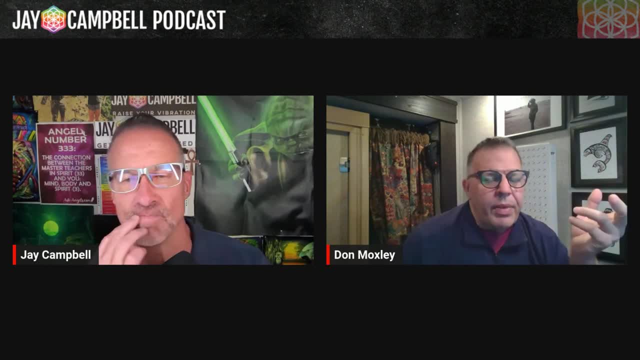 I watch my kid walk through life. You know my kid's one of those kids that grew up. you know she. she had a cell phone relatively early. We were very we paid a lot of attention to it And the re one of the big reasons we did is is Jacqueline was a very good athlete. She. 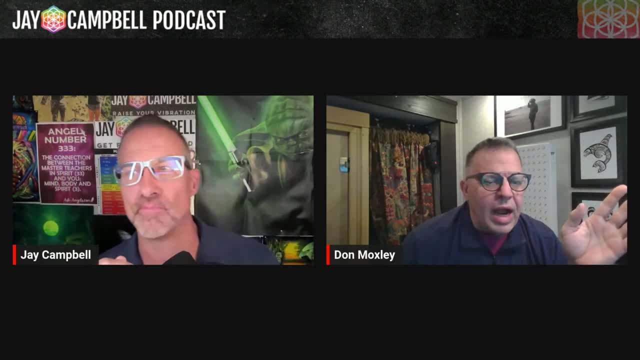 was on travel teams- We were all over the country with both hockey and lacrosse- and social is how she connected to all these kids And now she has these incredibly vigorous, uh, relationships with all these little kids, with these kids that she co, that she played. 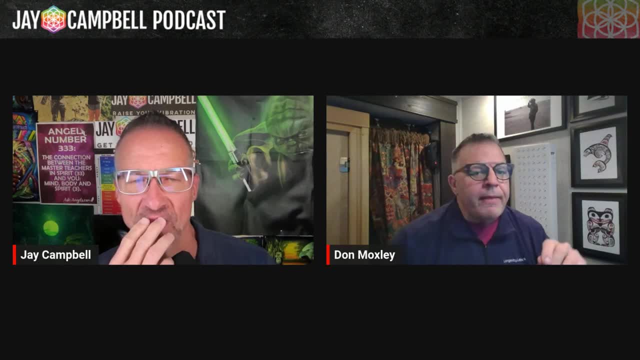 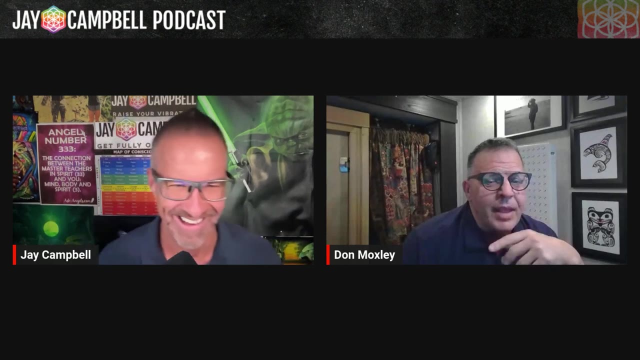 and coached with all these years And it's beautiful to watch. That's the other thing that happened. She came to me for help with a math problem one night And I looked at it and I'm like Jacqueline I: I don't know how to solve this. Um, well, she. she whips out her phone. 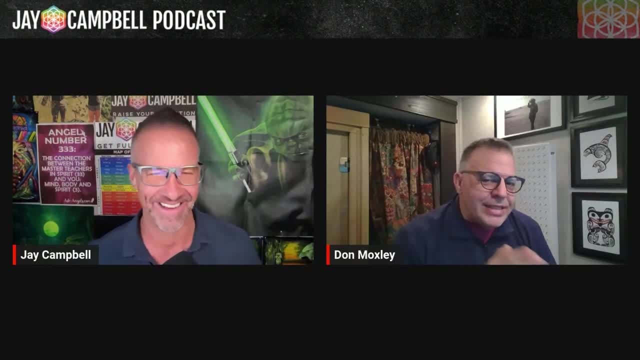 She takes a picture of the question She's asking me, she texts it to a friend of hers. Her friend sends back. here's the way it works. And I'm watching this whole thing. I'm like, Oh my God, this is so powerful, Insane, Yeah, Um, so you know, it's, it's. 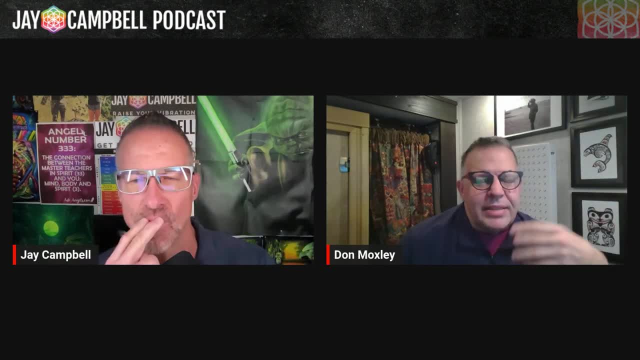 you know she, I don't, I don't think she's a tick. you know she has tick, tock and instead and those things like that, but I don't think she's, she's, I don't think she's hooked on it. 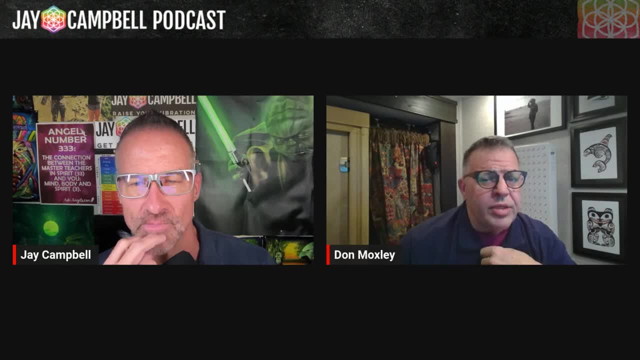 I don't think she doesn't define herself by by any stretch of the imagination. Um, so you know you, you gotta pay attention to it. There's no, you have to. I mean, that's just time we live in. 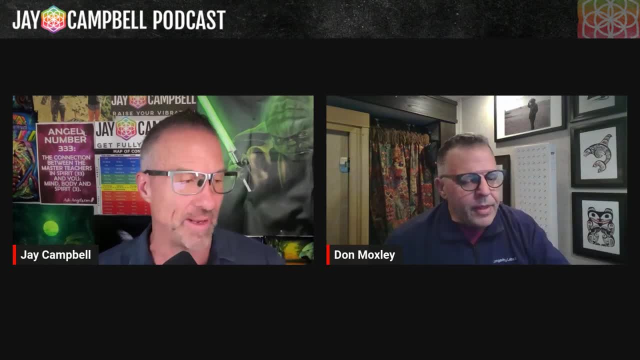 It's interesting- And I appreciate that we're going this way and that it's not just the talking points, because this is a good, free, flowing conversation. but it's interesting because there is a there's great benefit, as you just demonstrated, in technology. 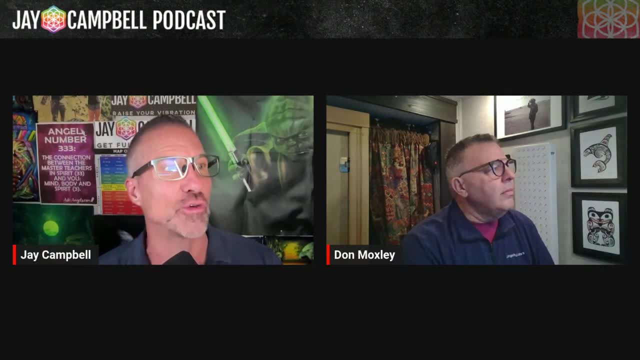 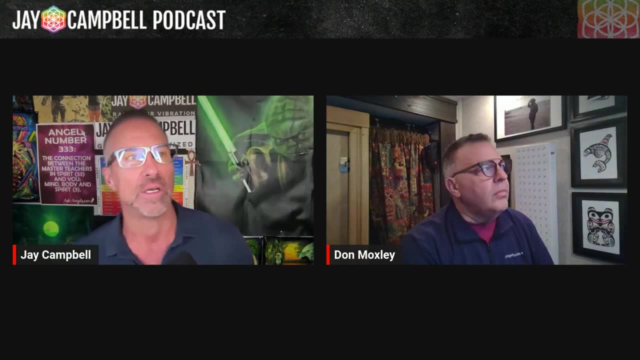 but you have to use technology creatively and not consumptively. And that's the issue is that most people consume, consume, consume, consume, consume. right, They go from Netflix to the internet, To video games, to porn, whatever it is. It's again, it's just this constant consumption that 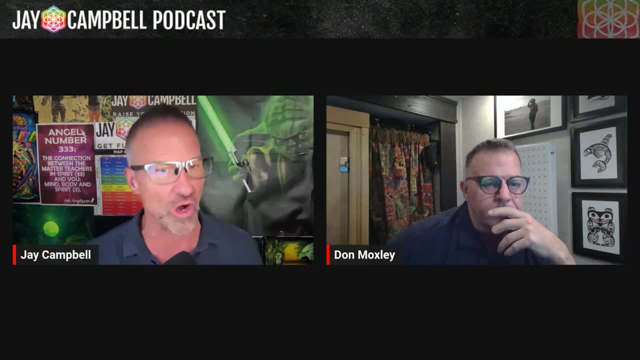 they're not creating. But if you use this amazing technology, like your daughter and her friend did, to create and to you know, think and and and build exactly And to build that, it becomes an amazing conduit And obviously it's an asset. but again it it comes back to what you originally. 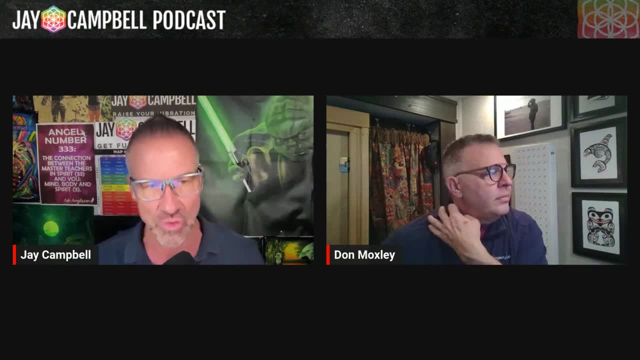 said, Like we as parents, have to limit the usage and obviously instruct the judicious usage of the technology. And you're right, bro. I mean, like how many people literally just look at their kids as a part of, you know, an addition to their house? 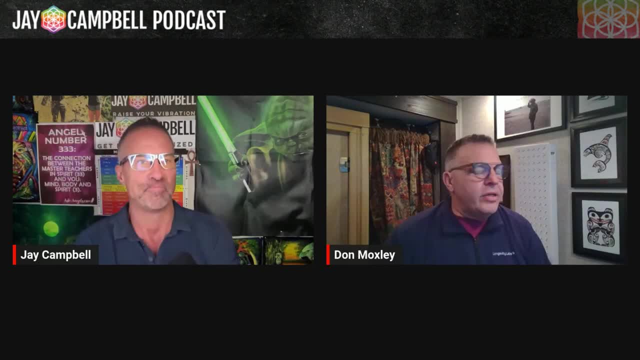 Well, I'll tell you, I have you ever um. there's a great author out there just to throw another book in the mix. That's what I do. It's called the coddling of the American mind. The author is Jonathan Haidt. Um one of the other books he wrote that I love is called the righteous mind. 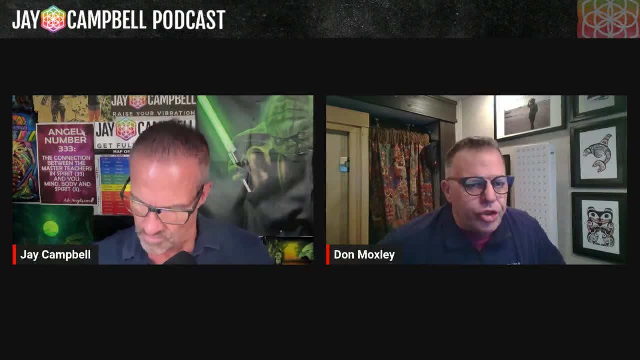 Why good people disagree about politics or religion. to two great books. Um, but the coddling of the American mind is a great book. Um, but the coddling of the American mind is a great book? Um. it talks about what's going on in education, in schools. you know that we're starting to see. 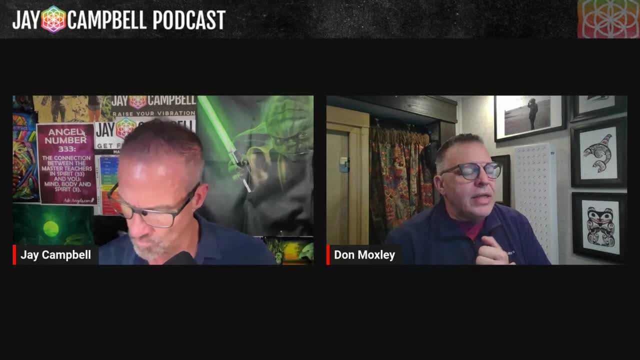 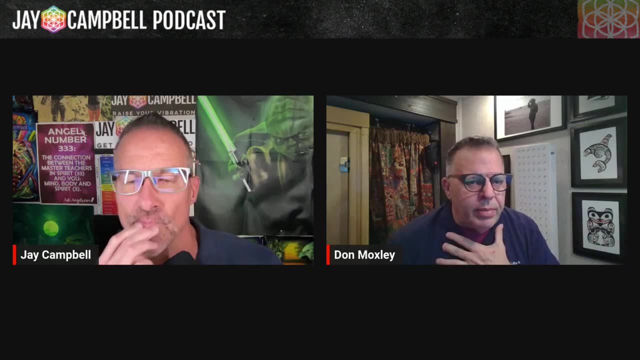 some pushback. There's certainly a pendulum that runs with this, but, um, if you're raising a kid and you're trying to understand technology and the difference between you know. listen, I turned 62 on my next birthday. I got all the way through my undergraduate without computers. 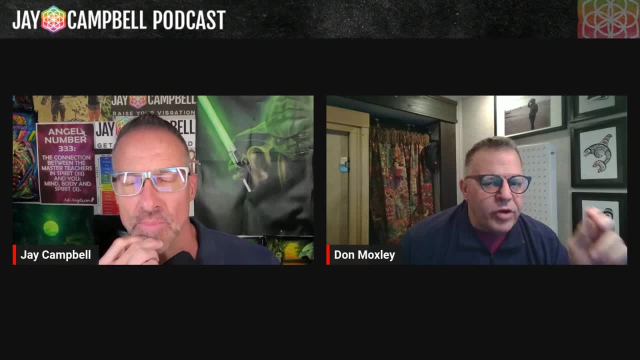 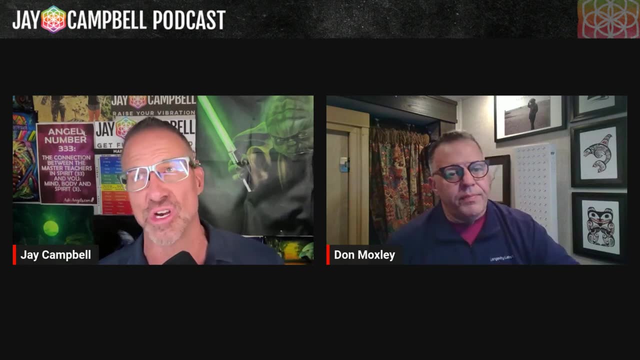 without using a personal computer. Yeah, I used my first personal computer in grad school and shortly thereafter, So we're similar. I my senior year. I'm 10 years younger than you- now really nine- but I same thing, Like my senior year of college: a green screen WordPress. 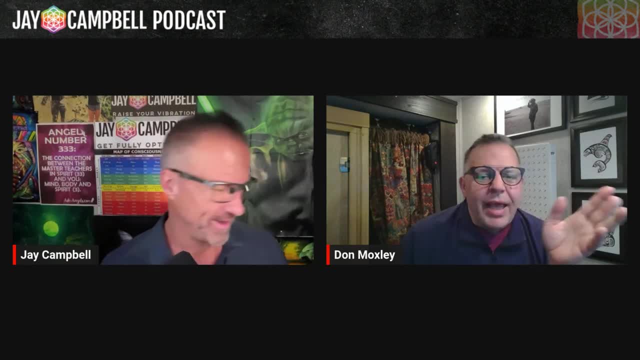 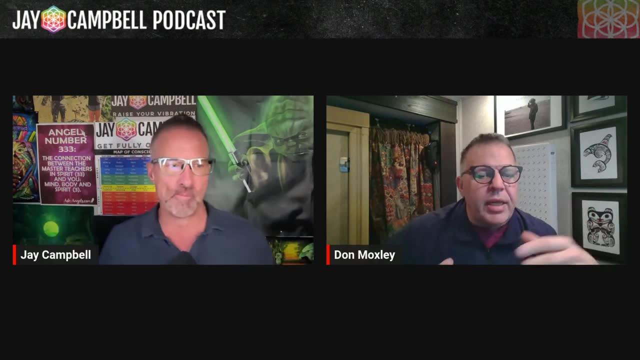 or processor came out. That was, yeah, it was. And listen, now look at us. Okay, We're sitting here communicating across this technology, which it's beautiful, the way it's worked this way, the way it's worked out, when it's used correctly. It's beautiful, Um. 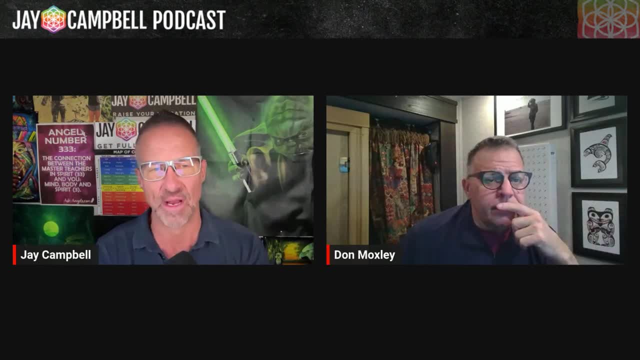 but it certainly has changed the game. It has And we all have to adapt. I mean, it's crazy because, like, no matter where you go, my wife and I were. we were people watchers, obviously, but the other day we were. I forget where we were, but it was like a place that had. 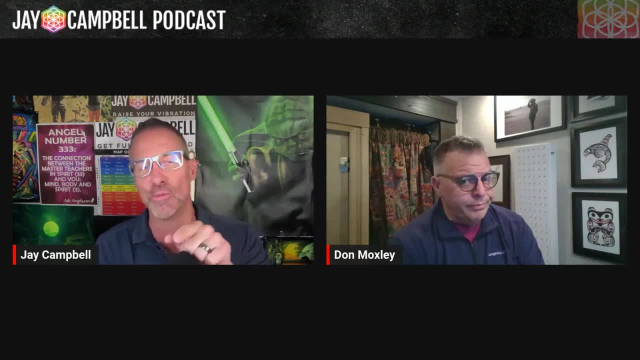 mostly seniors and you know boomers. and you're not a boomer yet, bro, You're still Gen X, but, like the reality, I'm the last year of the boomer. I'm the last year, Okay, cool. But these 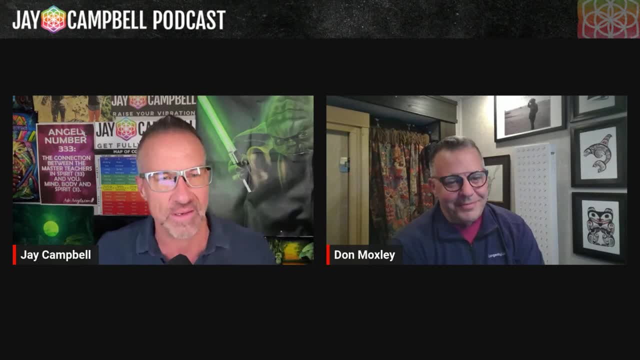 were people in their seventies And, um, they were all on screens Like now that literally every single one of them was like this: Yeah, And my wife and I just looked at each other and didn't say it is contaminated. So all of society, I mean everyone- is addicted to quote, unquote, to the dopamine fix. 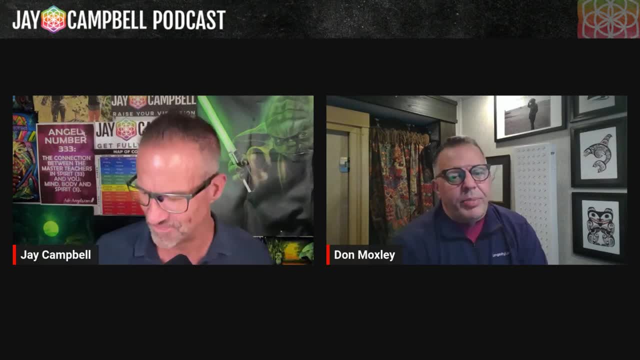 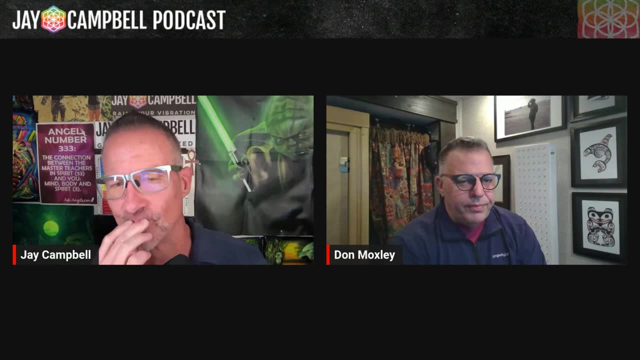 Yeah, I think, listen, I don't want to condemn, I don't. I, you know, I don't want to be that, you know that that that person, but, um, it can be very, very beneficial. Yeah, Can be, Yeah, Um, and I think this is the challenge that 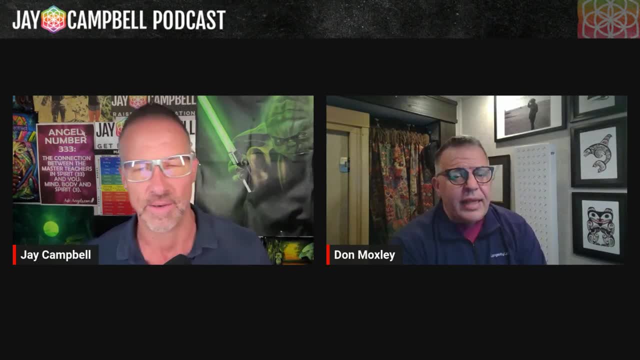 you know that when we have to recognize that the role of the role of artificial intelligence in social connections, in social networking, you have to be very careful about um if if you're getting the majority of your news from social media, you're probably in trouble. 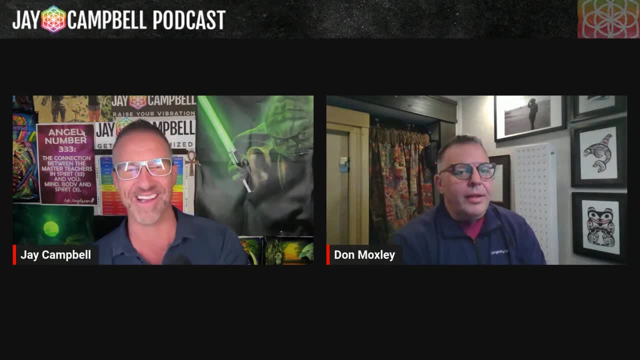 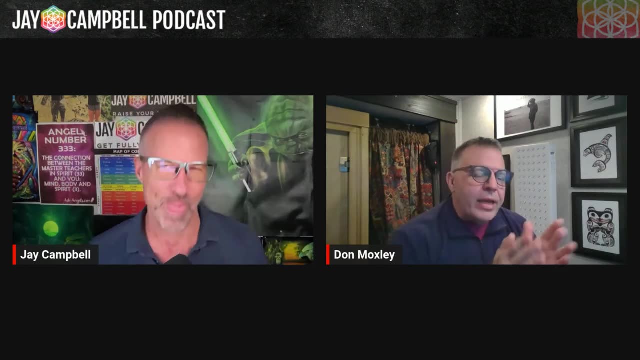 Yeah, Um, you've, you're definitely in trouble, Yeah, And well, as you listen, I, I, I have social feeds that I pay attention to, but I know where they come from and I'm not concerned about, I'm not concerned of of. 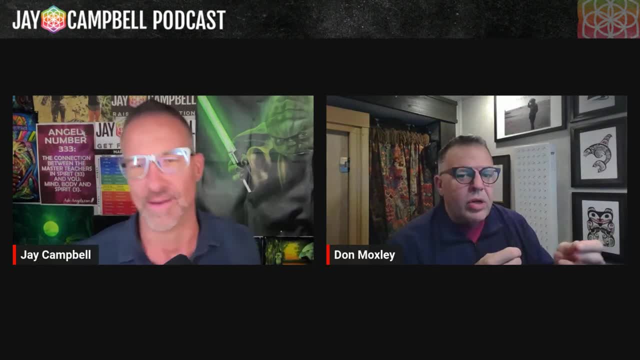 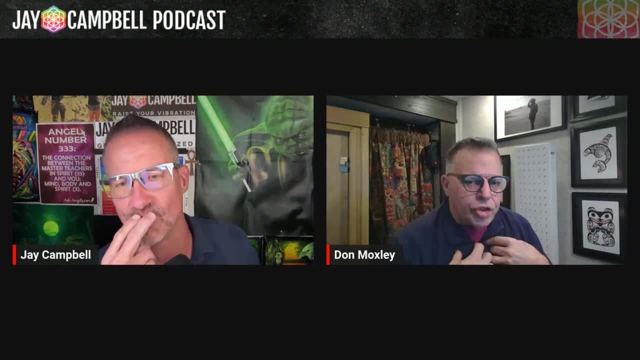 nefarious. uh, whether it's political or or or corporate, I'm I. I pay attention to those feeds. I'm a, I'm a judicious consumer. Yeah, I got it As as I am with my written material, as. 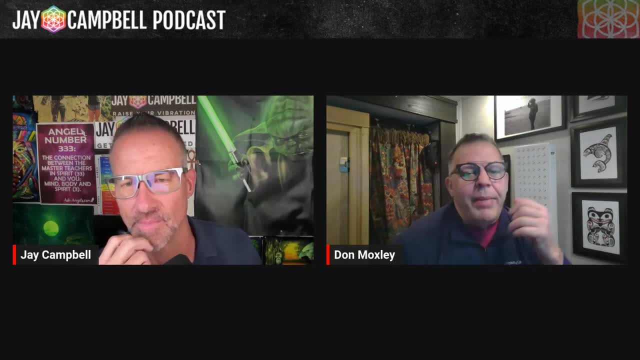 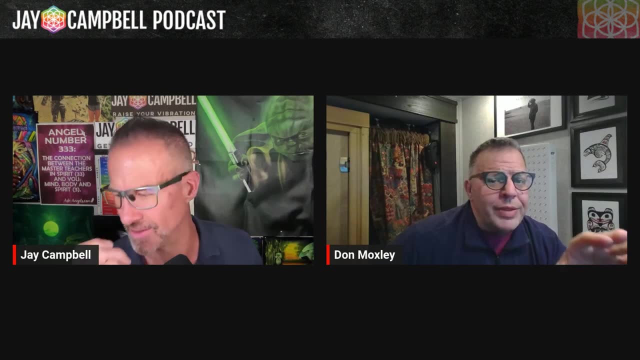 well, I mean, you know, you know, or, or a movie, you know, man, have you seen boys in the boat yet? No, I haven't, but I actually heard about it. The book first of all. the book is ridiculously good. Okay, I mean, I read the book in 15 when. 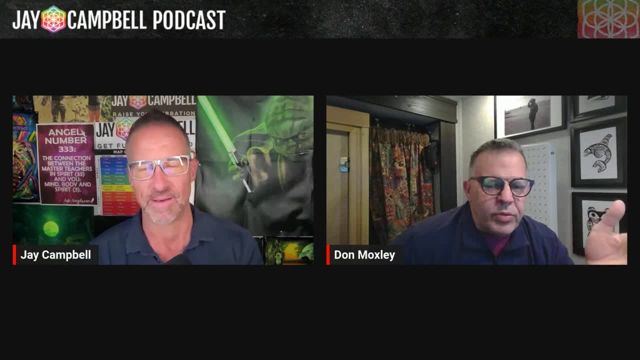 it came out when we were out in Washington. we went and saw, you know it was. we were in Washington, we were in Seattle and we went and saw the movie release out there. The movie's great. Okay, The book is 10 times better. Um, but, but I'm, I'm going back to 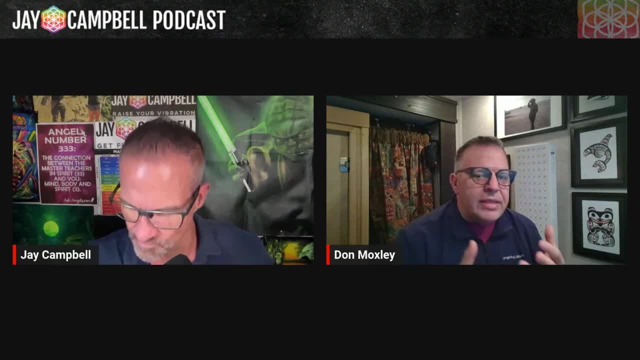 to authentic What is, is the information that we're getting, Is it authentic or is it curated? Is it manipulated? Um so, and I, and again, I'm not a, I'm not a huge conspiracy theorist, I- 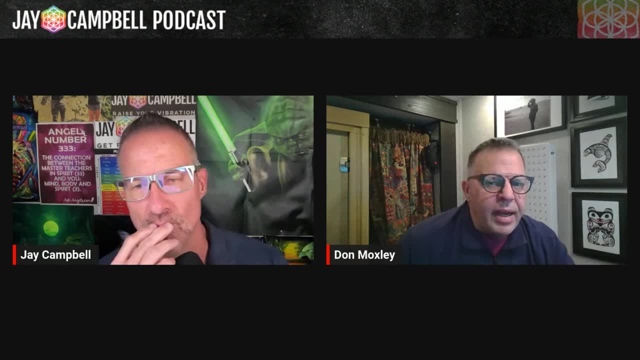 I tend not to go down those, those rabbit holes, but I'm also a very judicious consumer of information, Uh, and I always take a step back and say: wait a minute, does that make sense? I mean, let's follow this back. I mean, you know, people throw. 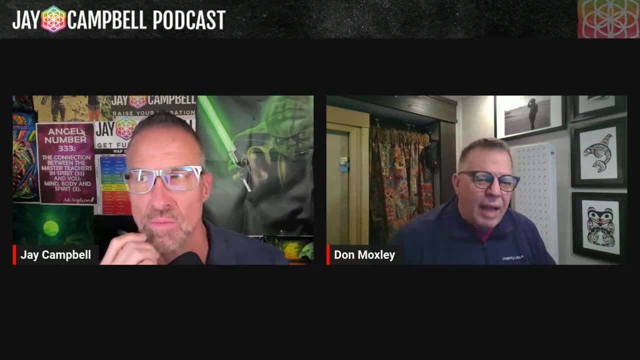 things out politically one side or the other, And I and I'm like, wait, stop from it, Think about what you just set, Think about all the things that have had to happen for that, for that. And I'm like, do you really think all those things happen? And when you stop and think, it makes a. 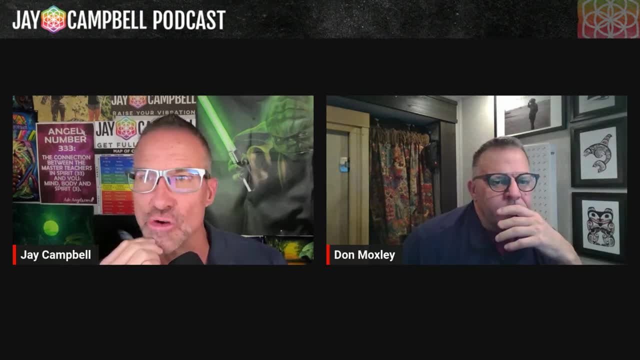 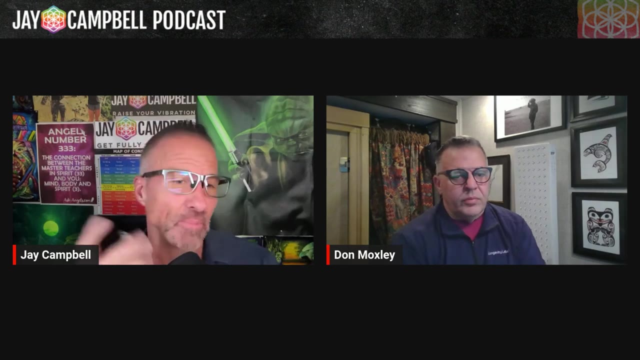 difference, The the you that you just said it best: you're a judicious consumer of information, So you're an educated, intelligent, critical thinking consumer of information. The average person is it, And unfortunately, that's the problem was. what you just said is that the media is so manipulated. it but, but we all 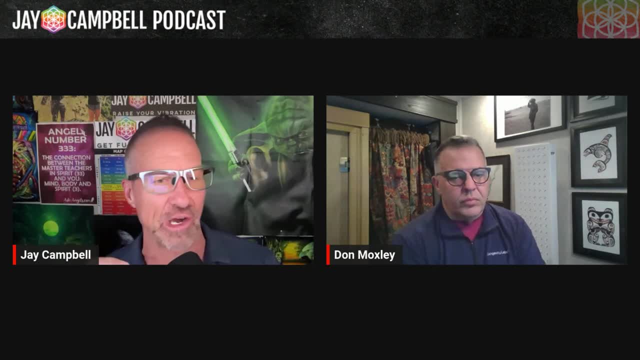 can fall prey to this. You know, like I, I know my wife sent me a link like three nights ago or two nights ago, you know cause. there was a tornado that went through Panama city. What happened on? and she sent me something off of Instagram. you know, to Instagram, which I mean, dude. 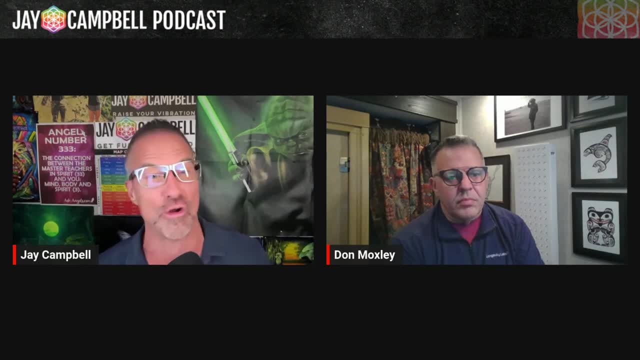 like at the level that I create. every day. I'm barely on social media. I might you know people say, Oh, you're on there. I'm like, no, those are my teams. But the but. the reality is. 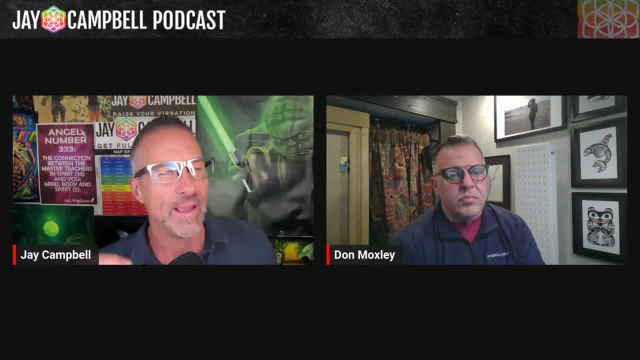 is that when I do go on, it's like if my wife sends me something or my daughter, And so I click on this link and it's like this fear porn, easily modified, you know, Photoshopped- tornado on the beach in quote: unquote. 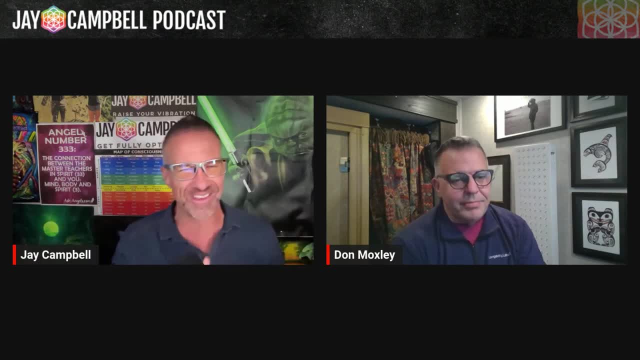 Panama city, And I had already seen the real footage and I literally sent this back to my wife and I'm like, what does it matter with you? This is fake, Right. But so the point is is to get back to what you were saying- is that, like, a lot of it is curated and edited and modulated. 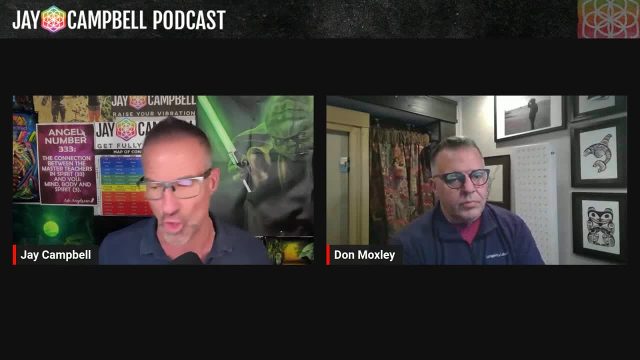 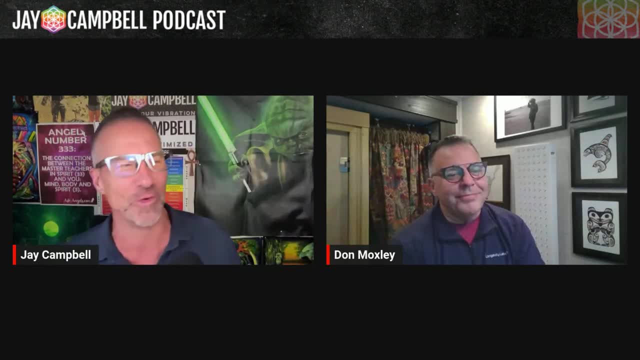 you just just consume, you're going to be misled and diluted And dude, it happens to the best of everybody, Absolutely, And it they've learned to tap into your fear circuits which are which are legitimate circuits, And, and, and you have to recognize that you know. 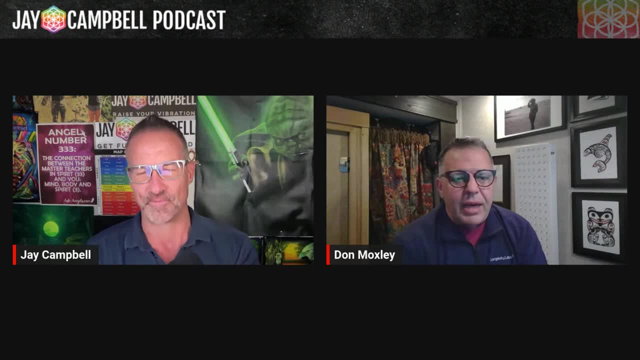 we're going full circle right now because you know we're here to talk about HRV plus and HRV- things like that- which is a measurement, is a measurement of fear. exactly this is one of the things that go into that and that's why it's. 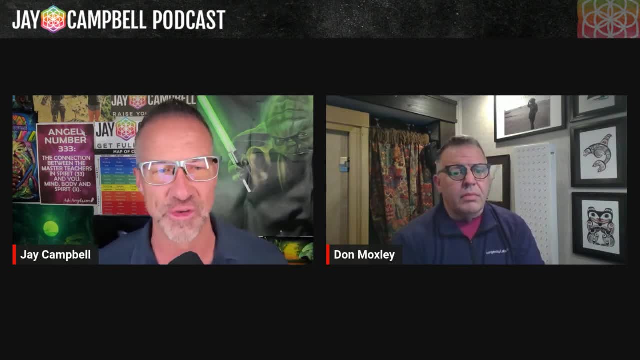 such an important thing to pay attention to. yeah, dude, that's a great point, so we'll transition, but i did. it's funny you say that because, getting back to literally what you just said about the point about how they track us, like you know, when you, when you shop right and you're shopping online, 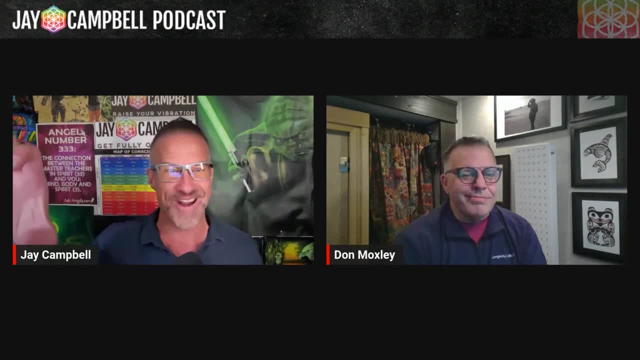 for whatever it is. you shop and then all of a sudden you go on your first social. there's the right. you're like, wait a minute, like how do they? that started happening five or six years ago. but again, how many people- you and i, because this is our life- but like how many people truly are even. 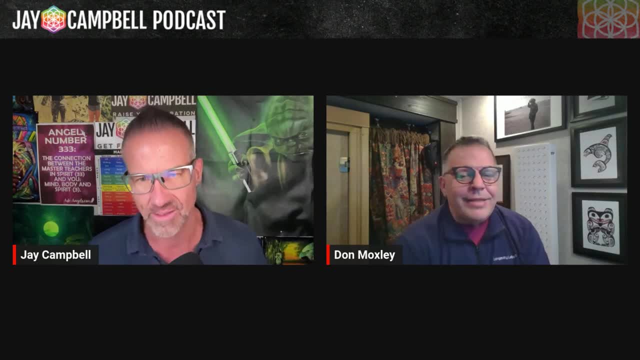 aware that that's influencing their decision. now i gotta tell you that doesn't bother me, because i'd rather get ads for things i want rather than tampons, of course, of course, um, you know so, you know. so there, there is some value there, um, but i, i i'm with you on that. you have to recognize that. 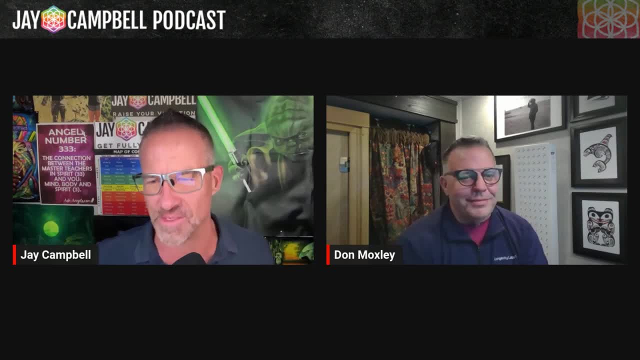 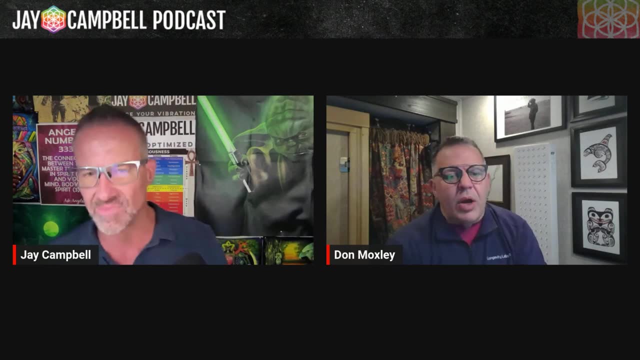 it's going on all right, so, uh, so getting into this a great great segues, but uh, talking point number one is: how did you get interested in heart rate variability? you know okay, so it was interesting. so i, i'm i've been trained as an exercise physiologist, for i i finished up my graduate. 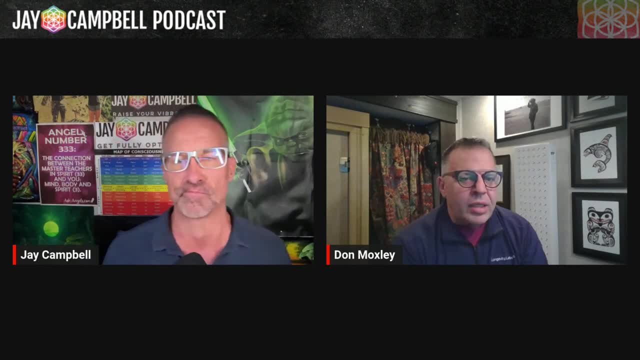 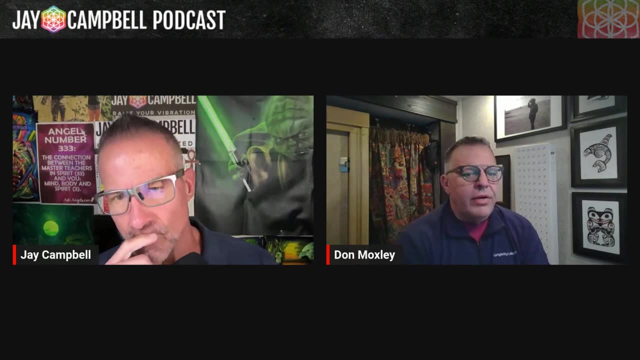 work in 86. um, it was a adjunct university professor by 89 and i've been, you know, i've been teaching the exercise sciences for for that long. yeah, um, now, along the way i had the opportunity to go work for polar, the heart rate monitor company. sure, 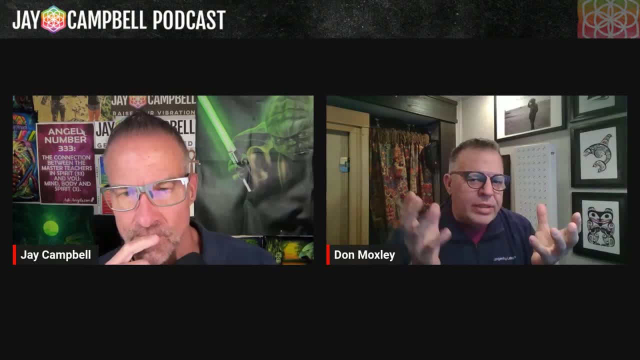 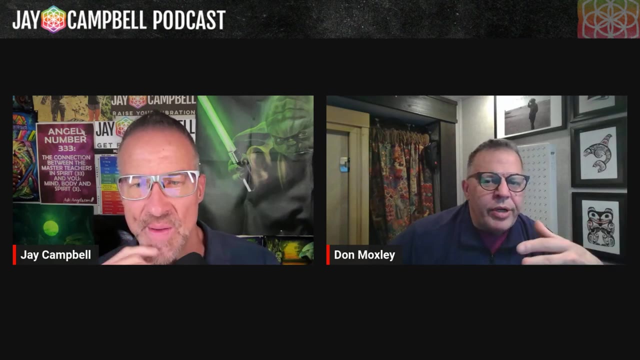 um, so i've always had a foot in academics, but i've always, i've always kept another foot in high performance and or tech. i love, i love tech. um, so, working for polar and, and one of the challenges- and you know this, jay- when you, when you're doing exercise, prescription intensity is 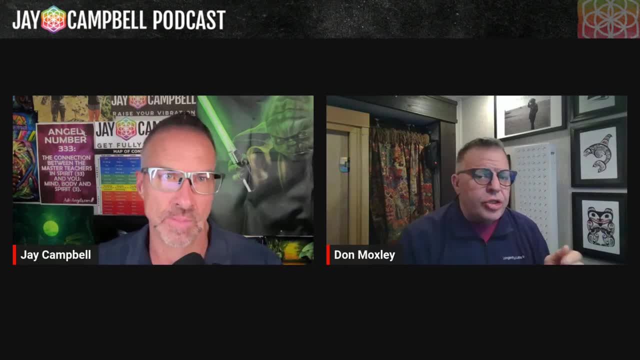 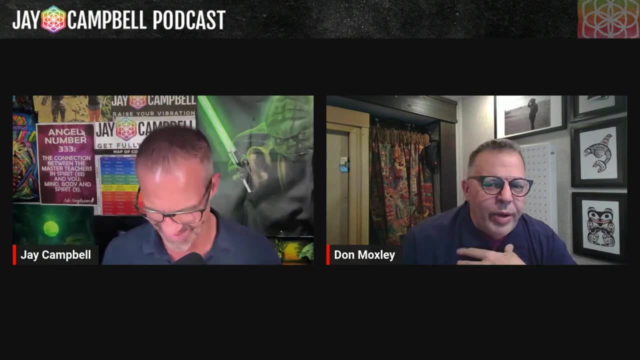 important and back when we were teaching this, we were teaching: 220 minus your age, calculate 85, yada, yada, yada. um, that's that's what we were teaching. in fact, we were teaching people to measure your heart rate by taking two figures and put them on your carotid. and all of a sudden, i've got this device. 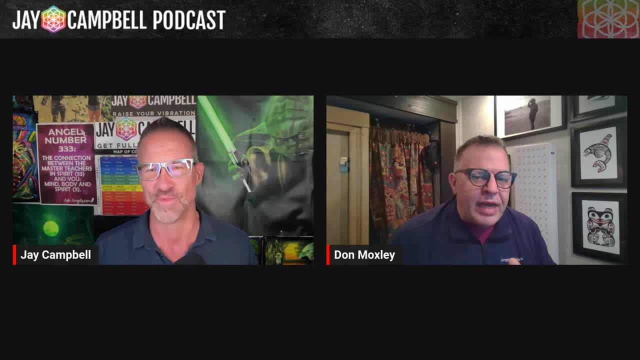 that i put a strap on and i have 90 accuracy. but not only do i have what my heart rate is, now i wind up with a with a representation of the entire workout. i've got these buckets of intensity that i can go back and evaluate. was this a good workout or was this a bad workout? or was this a? 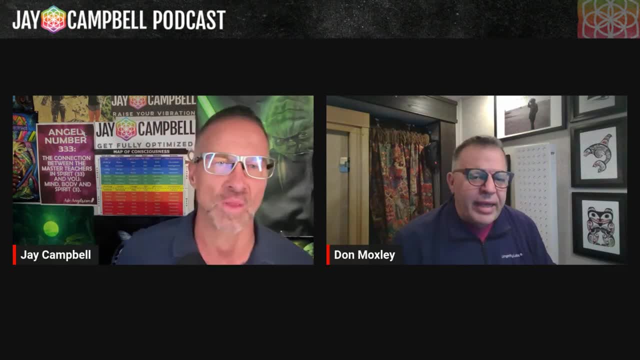 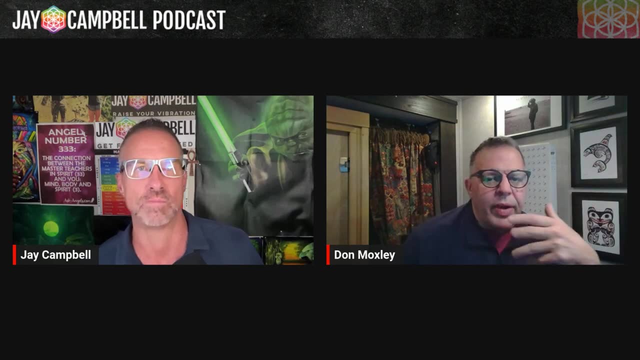 good workout or not, and how do i modify and so so. and this is consumer technology. you know these are, these are devices that you're buying for less than four hundred dollars, three hundred dollar range for the good ones. right well, now that is all in your phone. you know the the bad of the bad of the phone. 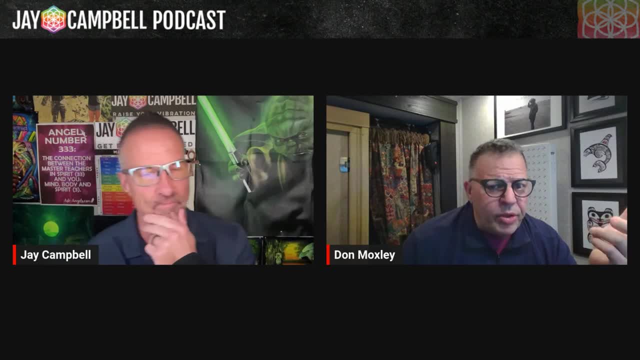 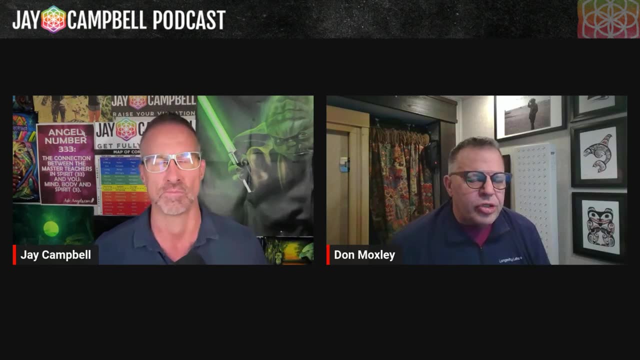 we've talked about. the good of the phone is that that's a, that's a computer in your pocket. that can be amazing. so, and while i was working for polar, i see they have these features that they're launching. it's called own zone, own decks, own something, and these were based on this concept of heart rate variability and 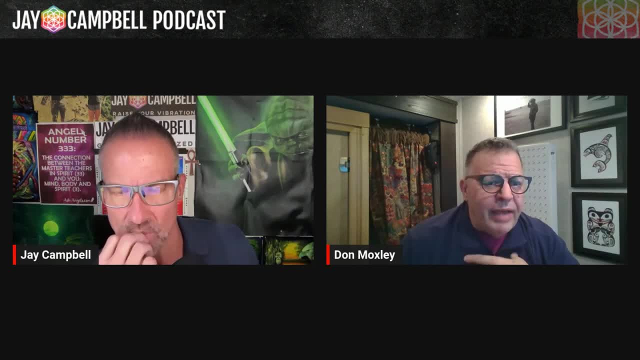 and i had. still, i had never heard this term. i'm, you know, i have a master's degree. i'm, i'm, you know, i'm legitimately writing curriculum reading, doing these things all the time, and i've never heard of this term. so i start to dig into this. i'm like, okay, this is interesting. and again, polar is a. 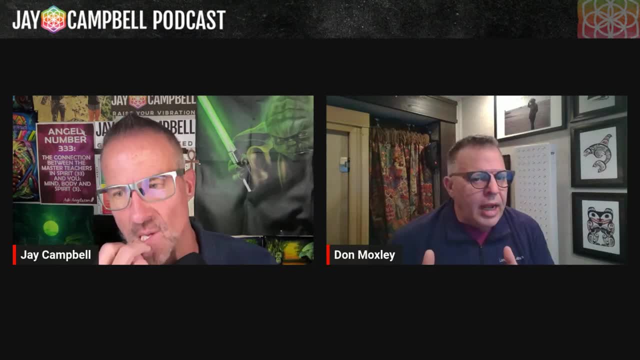 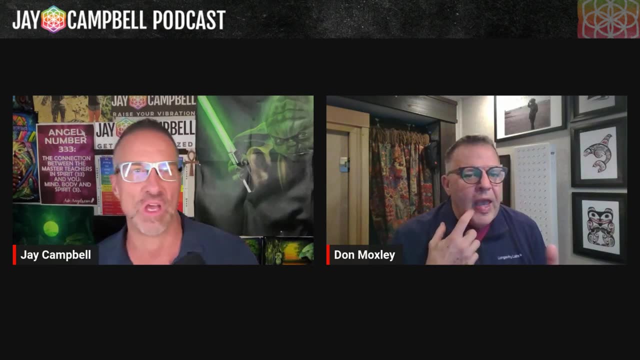 finnish company hrv is very much a russian uh variable. the russians really figured this out in in the early 60s with their, with their cosmonaut program, yeah, and their and the sins took it and in and put it in technology. um, so i'm all of a sudden to do exercise prescription. i'm not locked into 220 minus your. 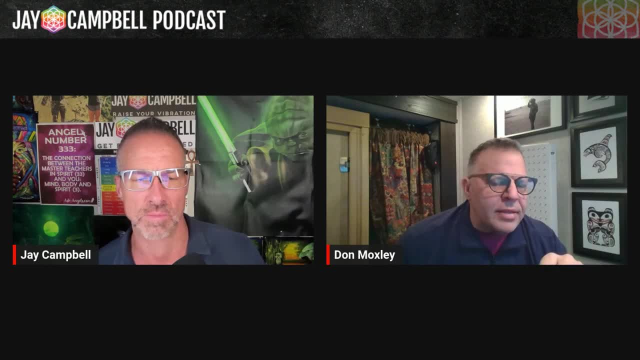 age times 85 and 70- i'm now able to look at. they had the ability to look at exercise intensity from the bottom up. they had this little test that you did. you sat for a minute, you stood for a minute, you walked for a minute, you ran for a minute and it was looking at the 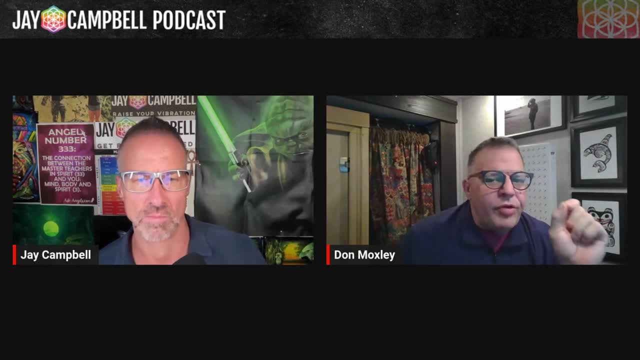 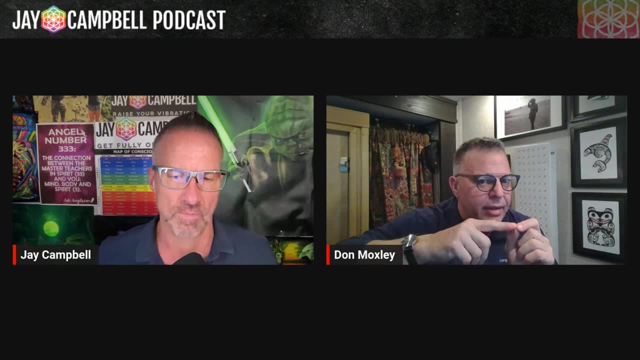 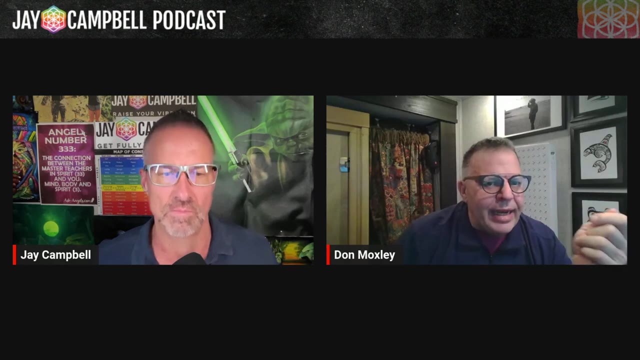 change in hrv with each of those stages. it gave you the bottom of the zone where we were calculating the top. it was giving me the bottom and the bottoms where the value's at knowing that point is huge. go on for a few more years. you learn about lactate testing. you look at lactate and 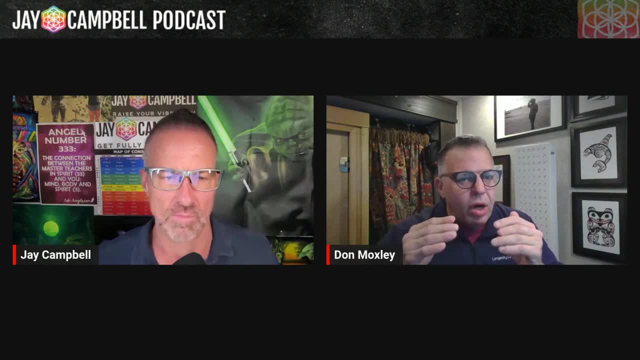 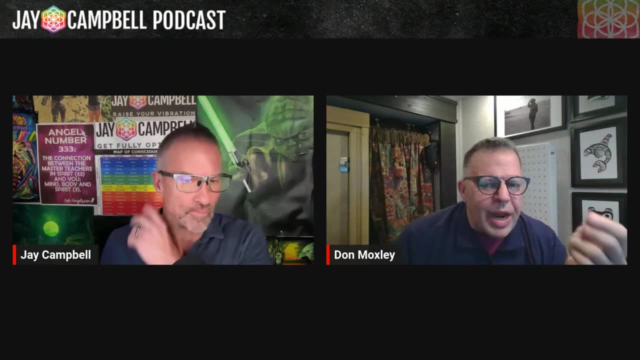 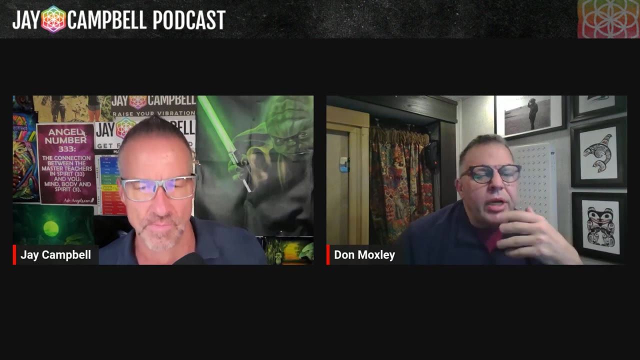 its impact and that shift between zones three and four of a five zone system, you know, and it's like: okay, this is so. so tech is what's driving this hrv thing, the, the availability of good consumer tech. well, you, we go on a few more years and 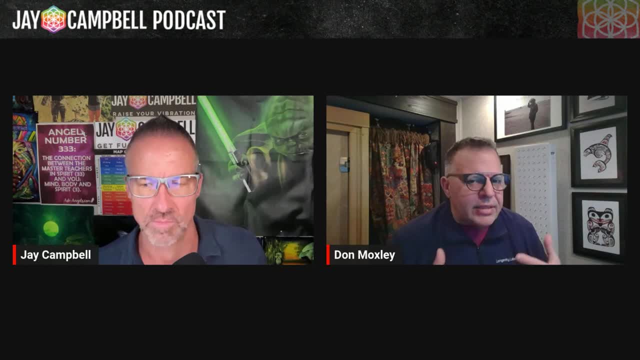 and jay. i had a lab that i people would come to me i would do testing, i would do this work and i got to the point i had a- actually had a police officer. i had a nine o'clock appointment with with a police officer to do testing. he comes in and i just got to where i was collecting. 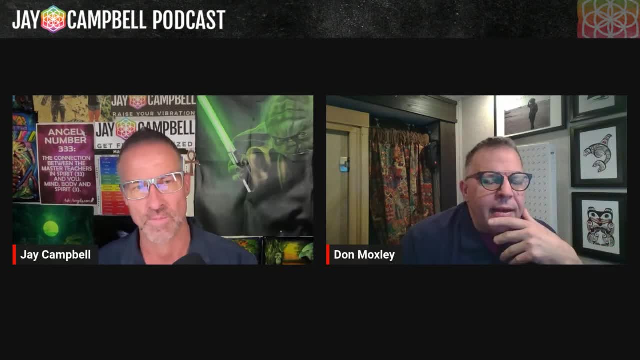 resting hrvs before i tested everybody and um why i was doing that. i'm not exactly sure. i just knew at some point. and this guy comes in and is: is resting um rmssd or is this classic hrv score that most people use is in the is below 20? yeah, and i'm usually not comfortable doing a test on. 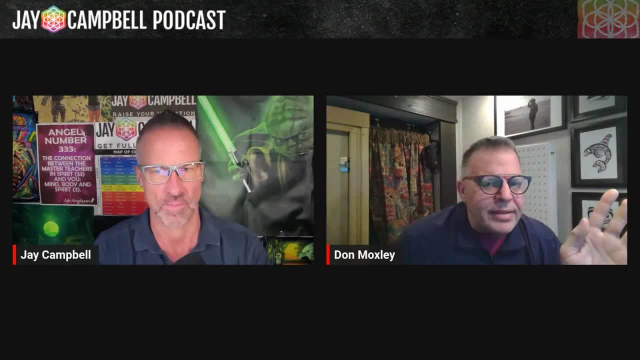 someone, unless it's 35 or above. didn't know why at the time, but that's just where my that's where the science met the art, right. um. so i said to him. i said: so what? what? i said? what did you do yesterday? tell me about how you slept last night. and he looks at me, he goes: how do you know that? 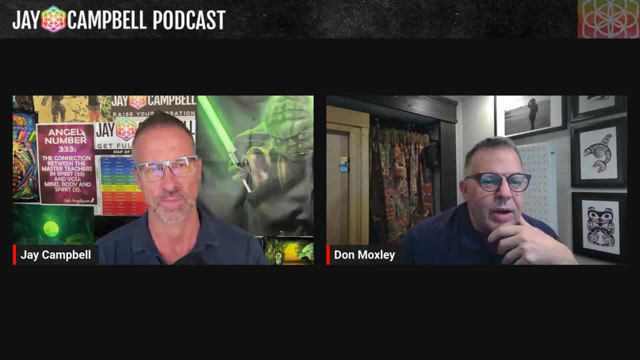 i said: well, just tell me. he says: well, i didn't sleep last night, i just got off work. i worked midnights and i came over here and i'm like okay. i said i'm glad i know. and again, when you're, when you're working in a lab, you don't know what this person's been through the last hour, day, week, month. 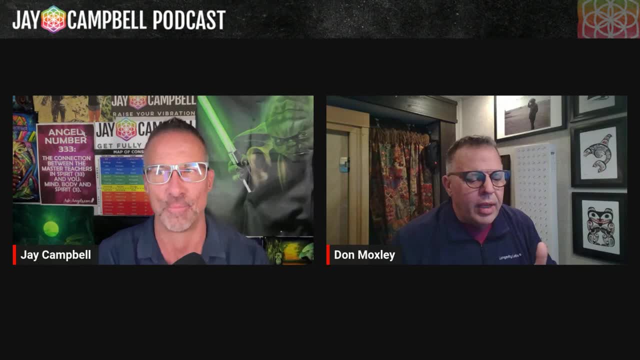 you don't know what they're bringing in. you just have this person sitting in front of you. if you think you can take anyone and throw them on a piece of testing equipment, not knowing background, you're kidding yourself. you're, you're again. you're that formulaic person. 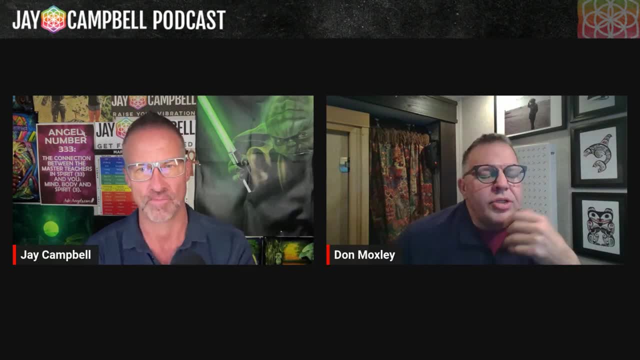 you're not the person who really dives into this, yes, so so that was the first time i'm like: okay, this is. and this guy, listen, his fitness test, his employment depended on his fitness test, sure, and i said we shouldn't do this stuff. you should, you should go home, come back, get a good 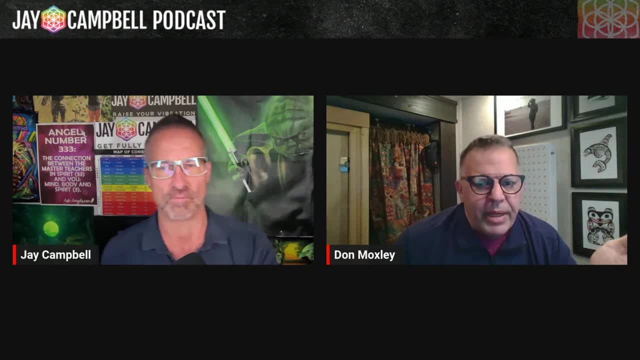 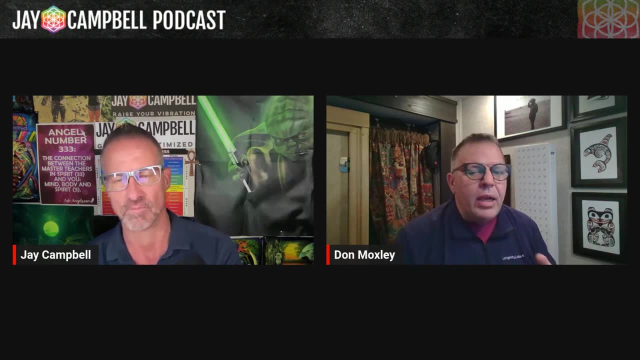 night's sleep and let me. when he came back, his resting hrms sd was in the mid 60s, so we went i was able to get was valid at that point. okay, so we then move along. so the hrv- measuring: hrv was something that i that just became part of what i did. i had a little facility in that little town. 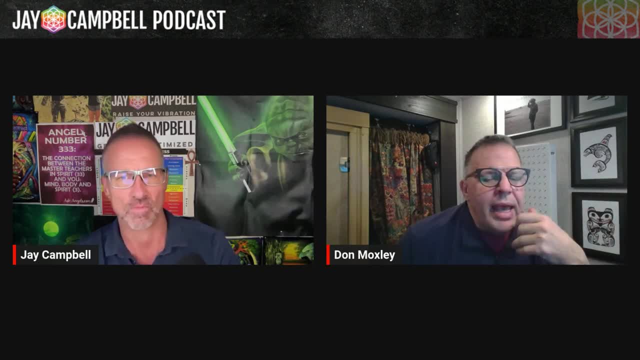 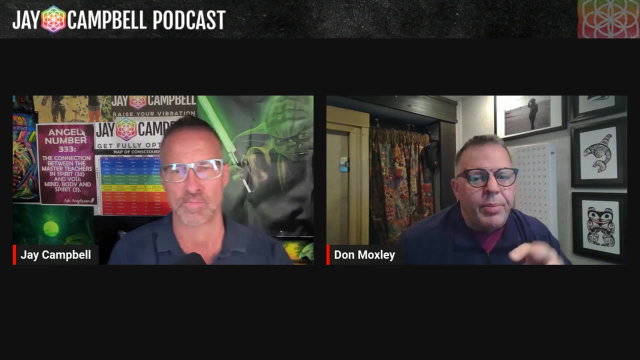 that i, that i grew up in and that i lived in granville and um the, the wrestling coach from ohio state. i'm an ohio state wrestling alum. i was on the team 80 through 85 and the current coach had come over um. he wanted to do exercise testing. he was riding a bike and he was riding a bike and 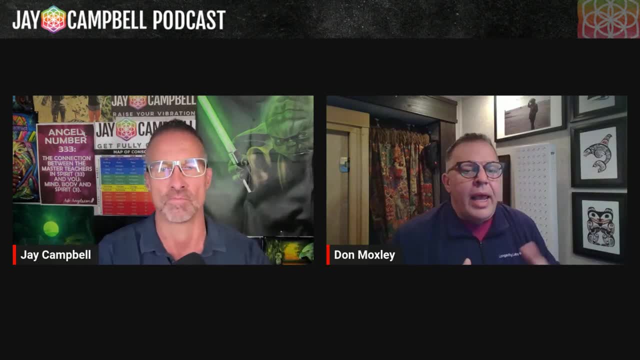 bikes and wanted to get better. and it came over. i did the whole routine and he loved it, you know, i mean he really bought into it. well, two years after that he calls me. he says i've got an athlete that's struggling that i want you to test, and i said, well, i said i can't, i can't do that for free. 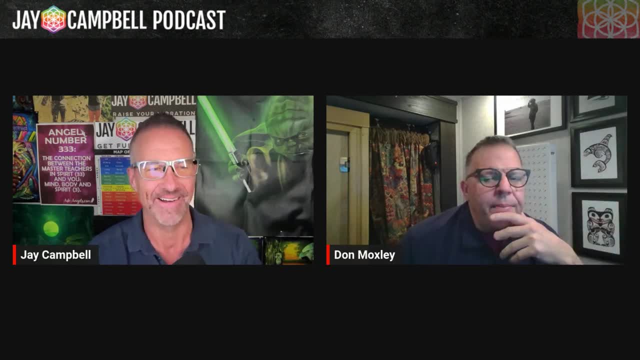 we've got to do this and he's like: no problem, bring him in um. so this kid comes over and this kid's a very talented wrestler and this was 2015. so, and to put the and to put it in perspective, ohio state at the time. 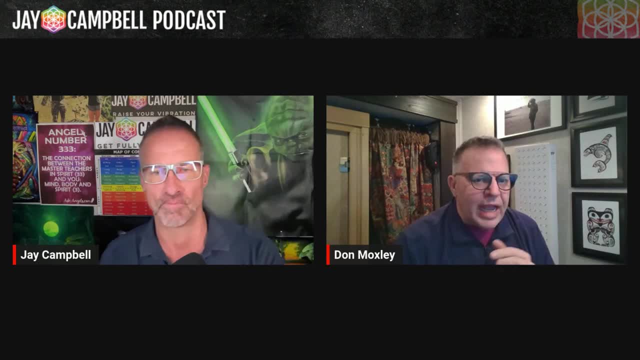 had a wrestler who had won three national titles and was coming back to win his fourth and to date there's only ever been five guys that have done that. so at the time there had only been three. before that. um but um, and we had these three freshmen that were very talented, wanted 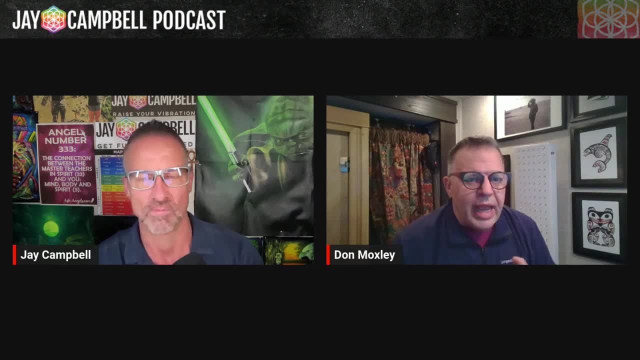 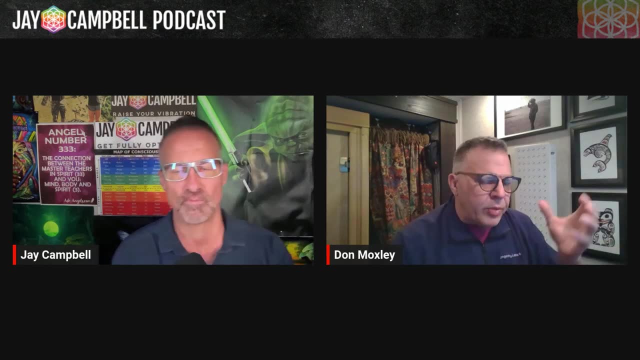 going on to win an olympic gold medal. all three of them were national champions um. all three of were four-time all-americans um. so we had them as freshmen. we had this, we had logan who was coming back, but to win a national title in wrestling, you really. 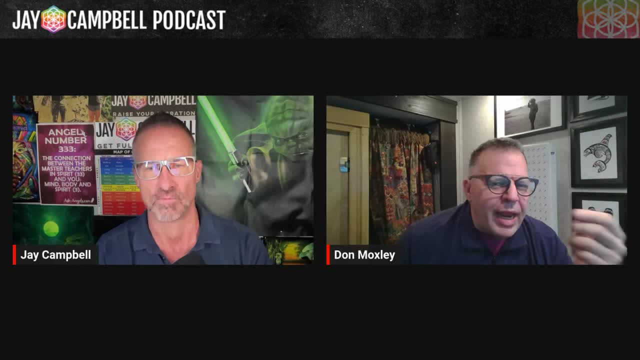 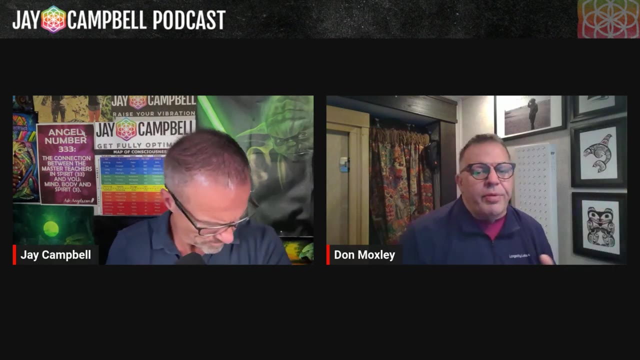 need five, six or seven point scores. you got to score 80 to 90 points back then, and you need four or five guys to do that. well, one of his wrestlers was this very talented wrestler from pennsylvania- uh, two or three times state champ in pennsylvania, which is really hard to do, and this kid was just 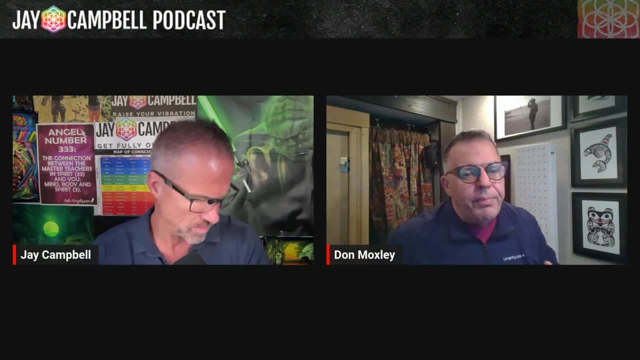 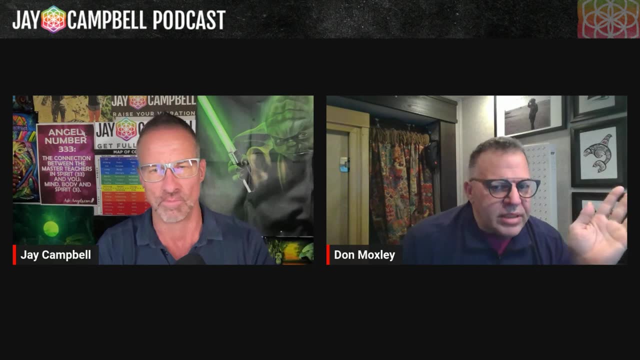 underperforming coach brings him over, i wire him up his resting rmssd. first thing on a sunday morning, after having not wrestled since friday night, was 15 milliseconds, wow um, which is roughly equivalent to the score that if. if we're sitting in a room and a bear walks through the door, that's what our rmssd drops to. that that's. 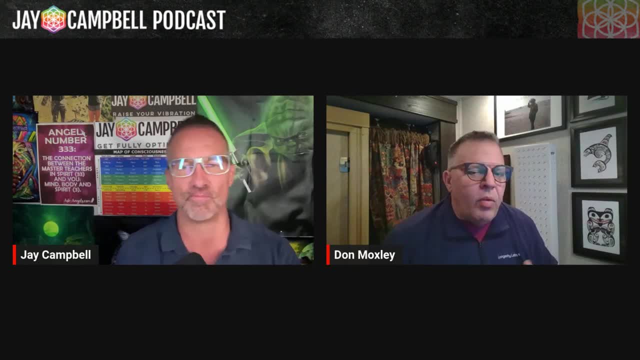 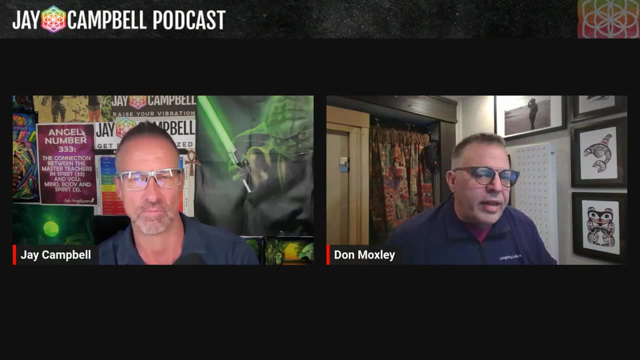 full stress, right, so i have this kid go lay down. while he's laying down in my facility, his hrb climbs up to about 100 milliseconds, takes about five minutes to do it, and then, when he stands up, as soon as he stands up, it drops back down to 10. 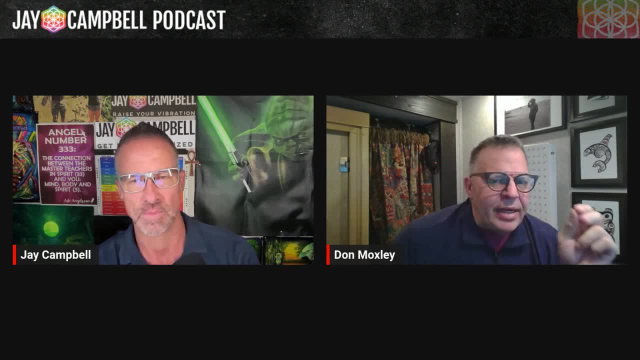 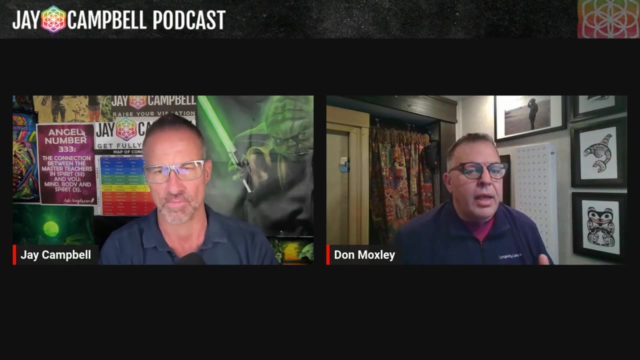 well, i'm like just the act of standing for this kid the body recognizes as a stress state. so i go ahead and finish the finish, the, the testing and his, his capacity was half of what it should be. the he was classic overtrained athlete. and i said to the coach: i said listen, i 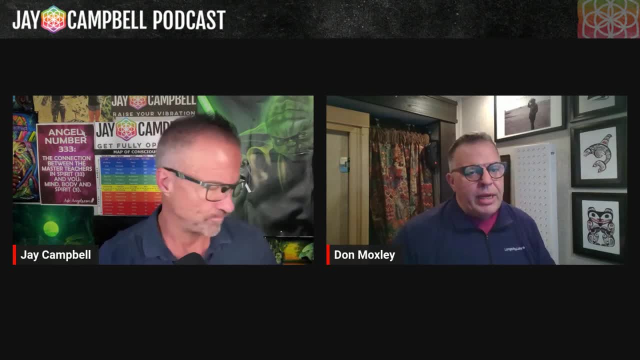 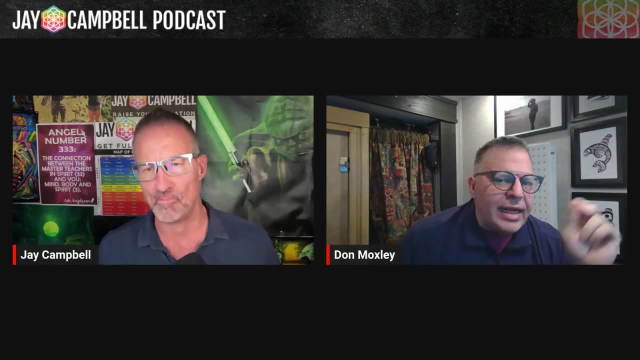 said i- i used the term overtraining back then. i don't use that term anymore and we can talk about. i said he's. i said this kid is maladapting to your training, he's not adapting, he's maladapting. and he said: what do we do? i said you have to training for what he's ready for. how do you do? 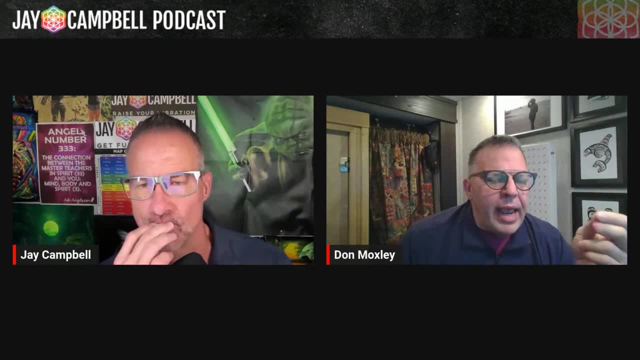 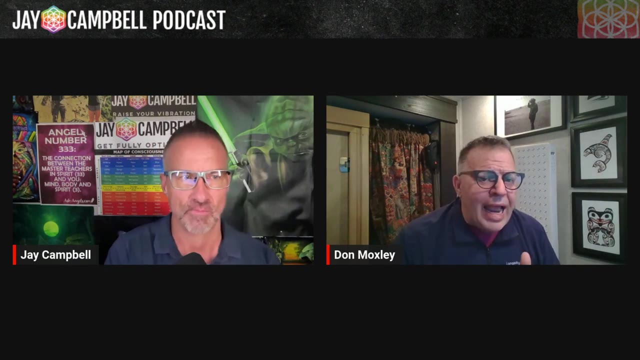 that i said we need to measure his hrv every morning and then we will go ahead and design his training so, literally, for close to three weeks we would measure in the morning and i i never released him to wrestle live for two weeks. i never released him to wrestle live for two weeks. 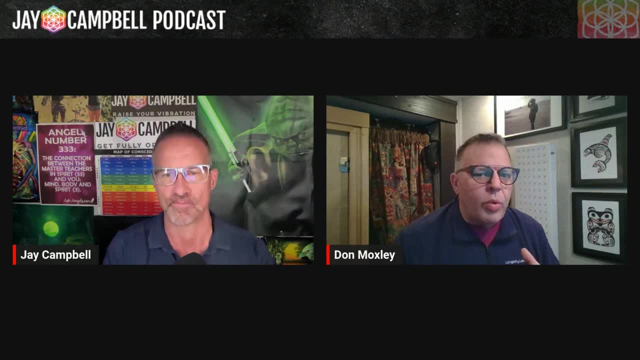 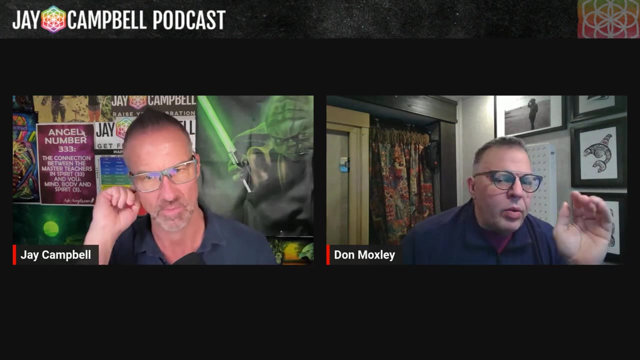 okay, because he just did not have the ability to do it without creating a huge stress response. yeah, so we finally backed this down and i'll tell you what. i'll send you a video that i did on this that you can put in the show notes. it's on youtube, um so, literally as we started to to titrate his 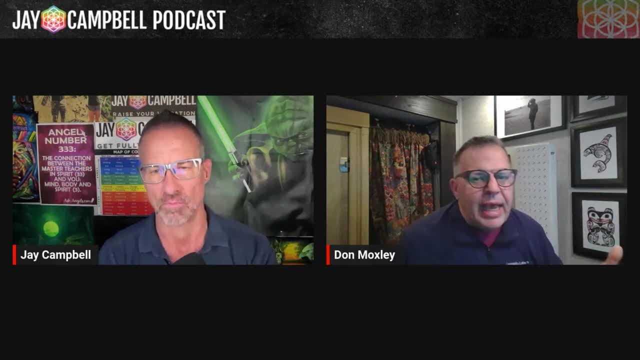 work. you saw hrv improve. we got him into big tens. we got through big tens, but the big deal was he finished hrv and he was able to do it for two weeks and he was able to do it for two weeks. and then the big ten. and if you know anything about wrestling, big tens is where wrestling is at um. 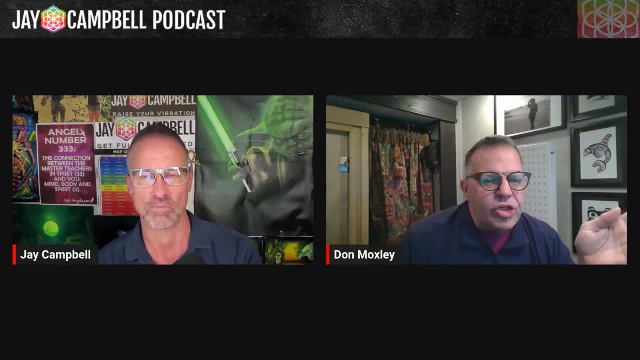 and we got him through. he finished eighth, qualified for nationals, but he had to score 12 points twice in order to get through that tournament, which for him he was winning matches- two to one, three to two, stuff like that. he was not scoring points. um we. so he scored and i'm thinking, okay, we're making. 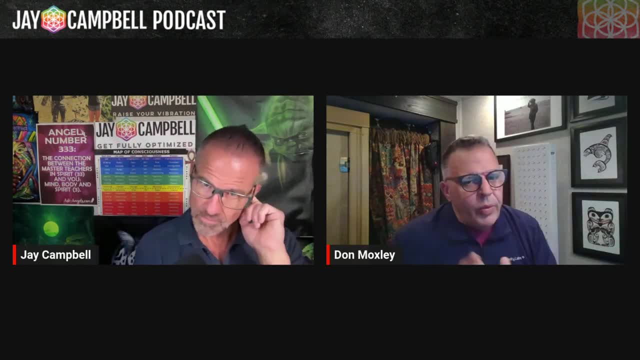 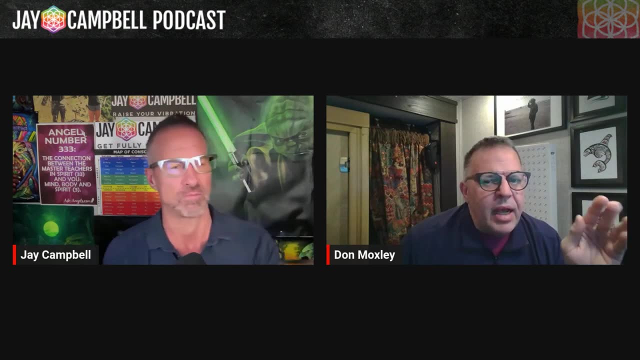 progress here between nationals and big tens we continue. i flow in some other, but i was able to send this kid to nationals with a resting rmssd of 75 millisecond. well, he winds up being fifth in the country um one score for the and the team wins the national title. now let me 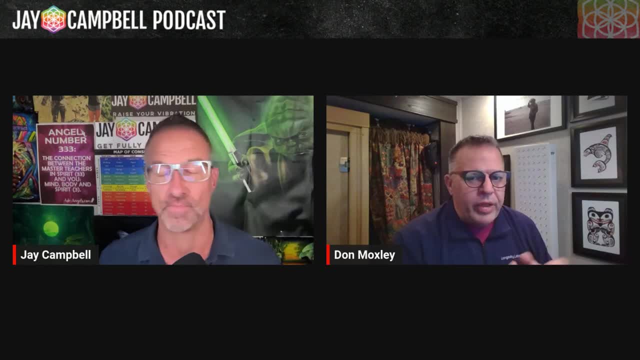 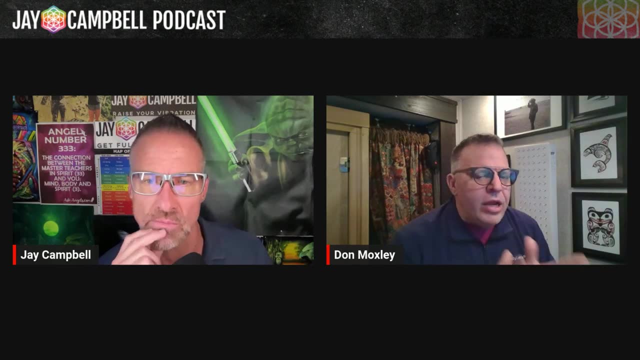 put this in perspective: when i first went into that wrestling room, when the coach brought me into that room, i knew the coaches. they knew who i was, but they didn't know what i knew. um, they knew how to train guys for nationals. they knew how to train guys hard. they were good with a whip. 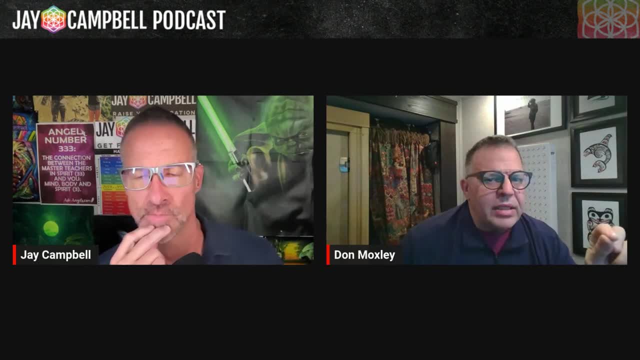 and when i would step in and say, no, this guy's not wrestling live, he's drilling. and i did that day after day after day. they thought i'd lost my mind. um, you can, you can't, you can't go to nationals, just drill it. you know, it just doesn't happen. and but you also can't train this kid, the. 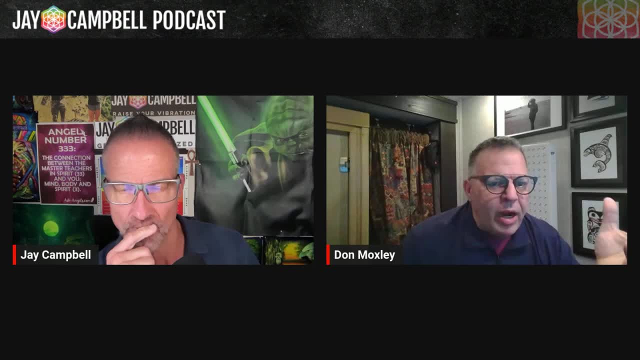 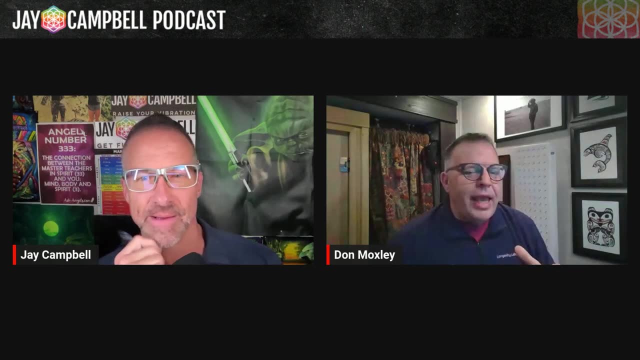 way he had been trained. um, so he makes all american and all of a sudden, the coaches look at me. they're like, okay, what is this voodoo that you have? yeah, um, and, and this started the process- they bring me on staff as a sports scientist and we start a program of measuring hrv- uh, one of my. 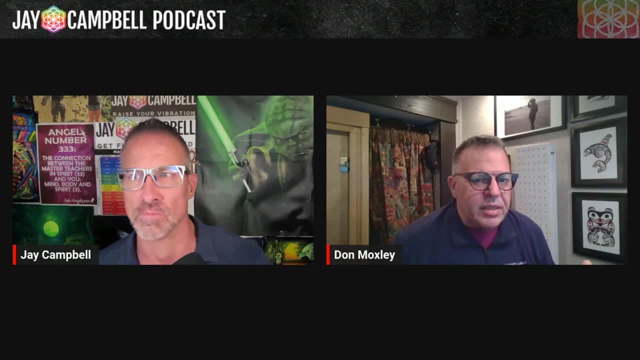 alumnus and a former teammate, uh, bought me a first beat system and we start doing 24 and 48 hour studies on the entire team. um, but i can only do one guy at a time. but we learned a lot and we moved the needle. we continued to improve, um, but then the year after that the us air force uh. 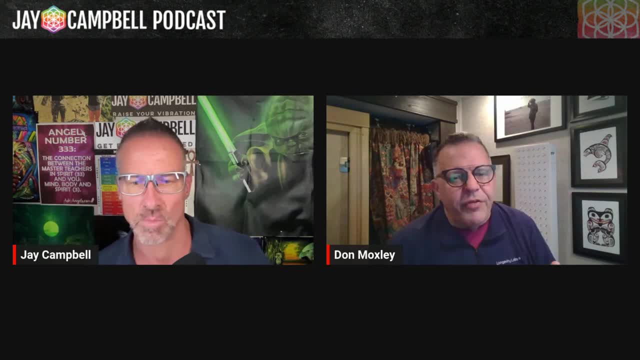 research, uh, the um- i'll think about the name- the air force research lab, where all the elite warrior data is done. this is where they look at navy seals and army delta force and all these elite warriors. they had come to ohio state to work with their athletic department in using wearable technology to 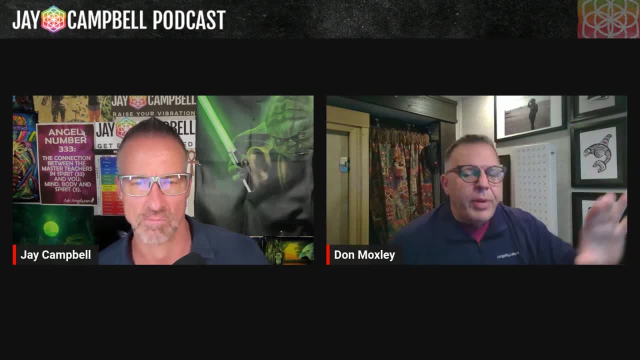 help predict uh athlete performance. and they'd been working with football and they heard about my program. so i went from where i could measure one guy a day and they say: what do you need? i need capacity. well, they hand me uh 16 omega wave systems. um, so i go from wearing one guy a day to 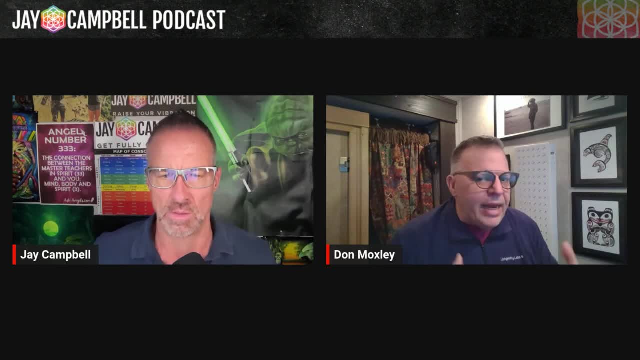 where i'm measuring 16 guys a day. um, our data continues to climb and jay. by the time i finished in 18, we went to national, so we qualified 10 guys for nationals in the 18 season- first time in school history that we qualified the whole starting lineup. we had eight all americans, the 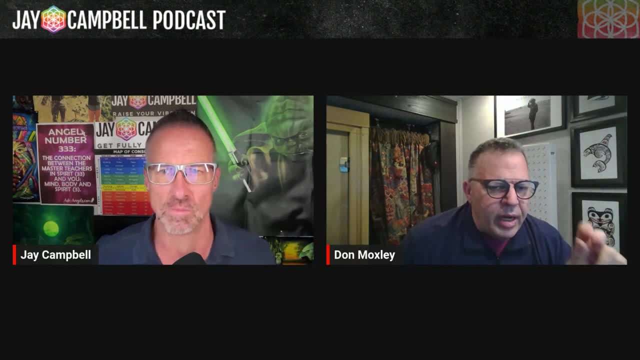 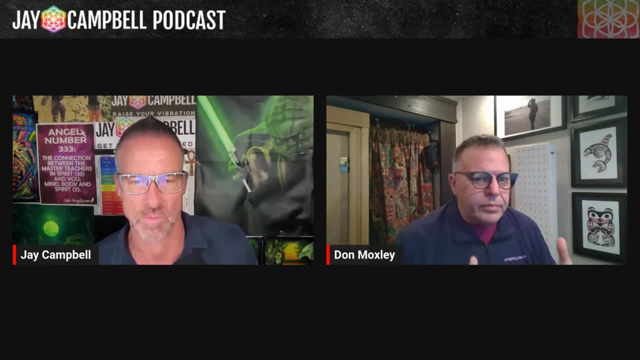 most in school history, the two guys that did not make all america's. i predicted the first day of the tournament now. i did everything i could to get these kids ready. i got eight of them there. two of them we didn't get there, but i got to where. if you listen, if 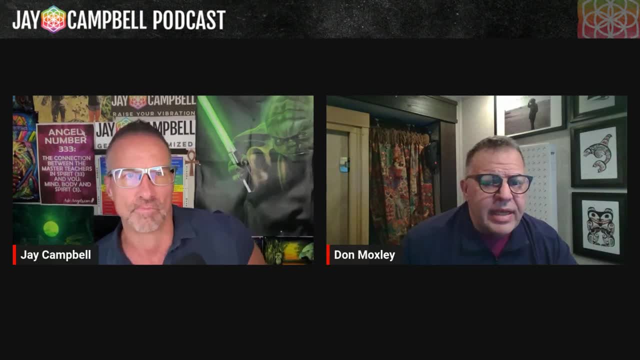 you're hrv. if you're a college wrestler and your hrv is not greater than 70 milliseconds, you will not make all american. my olympic gold medalist had 125 milliseconds. my national champion. why an olympic uh? bronze medalist was 100 milliseconds. my national champion. who did? 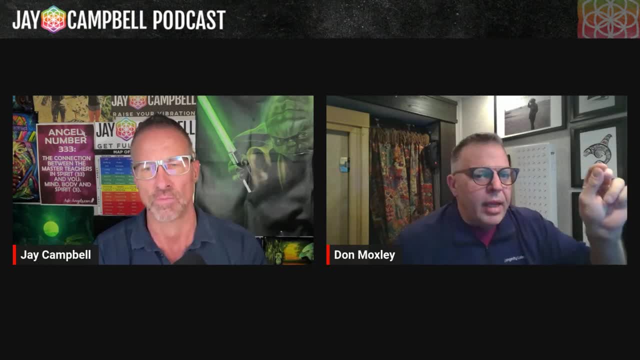 not have olympic experience. 96 milliseconds. literally, it was a linear relationship between hrv and performance. so we learned. what we learned is that we can train hard, we, we. there's a lot of people that can train you hard. okay, the question is, are you putting the the time in that that? 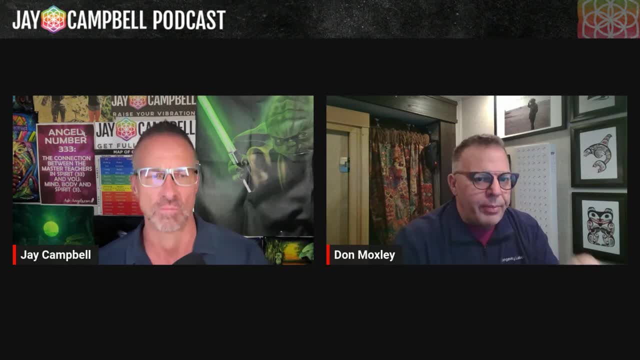 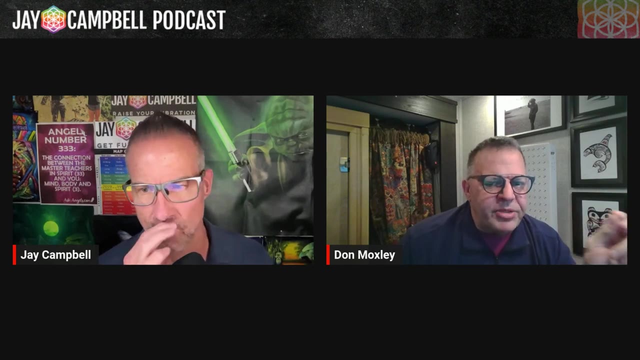 training yields recovery and growth and super compensation. and and again, going back to my the, the, the kenny, the kid i was telling you about first that we first started working with, one of the first things i had to do with him was teach him why it's important to sleep in a bed by. 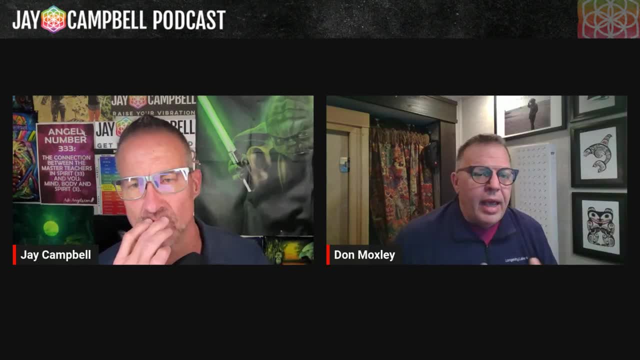 himself. now his girlfriend was bent out of shape, okay, and i said, kenny, i'm not saying don't have relations with your girlfriend, i'm not saying any of that. i'm saying finish your business up and either you go get back in your bed or she goes and gets in her bed. but i want you sleeping. 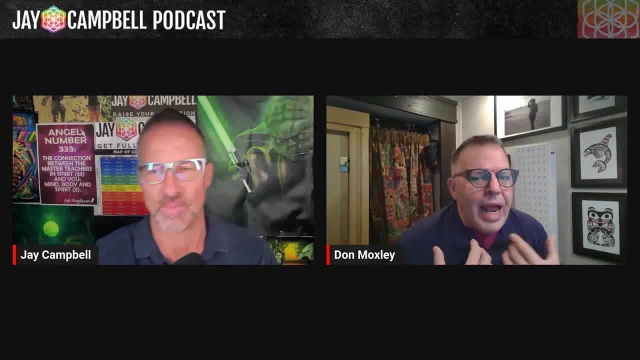 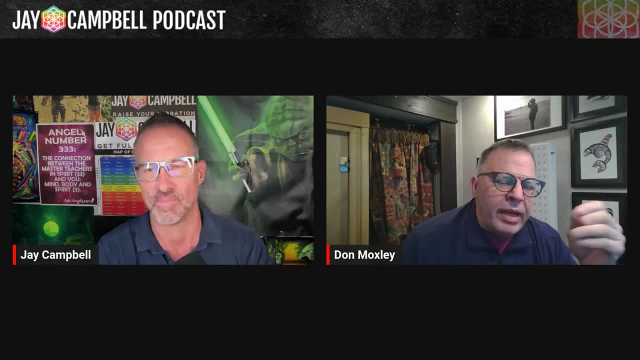 by yourself and i want you to turn your room into a cave. we were driving recovery um girlfriend was happy with me when he made all american um but um, you know, and and people could see it as we went. so this is how i learned about hrv. now the next step was kind of 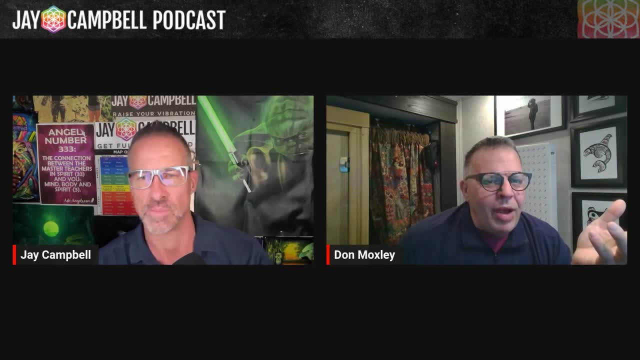 ironic- this is how i wound up working down in florida- that while i'm at ohio state i've got people contacting me from all over the country- pro, pro, strength coaches, people like that- and they're like: what do you know about thc and hrv? and i said i don't know anything about hrv. 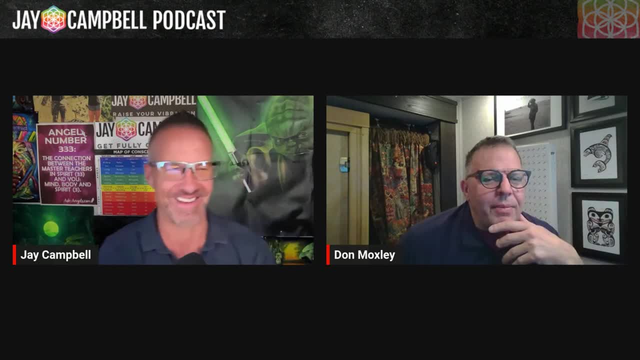 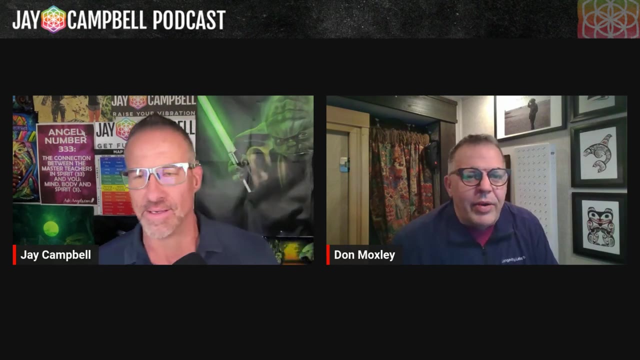 about it. my guys are ncaa athletes and um. well, finally, a good friend of mine that i worked with at a tech company in in um in new mexico calls me. he goes: you want to work in cannabis? and i go: yes, i want to understand this. he's so he. so he hires me to be the medical director. well, the director. 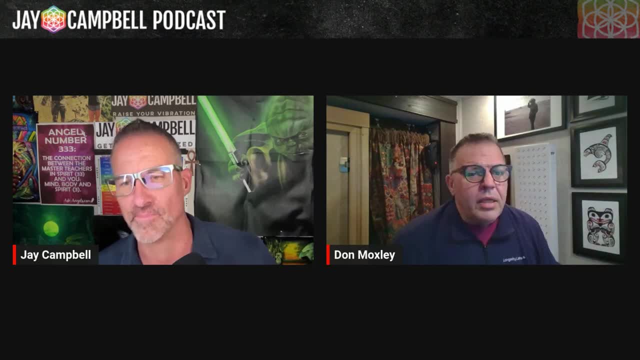 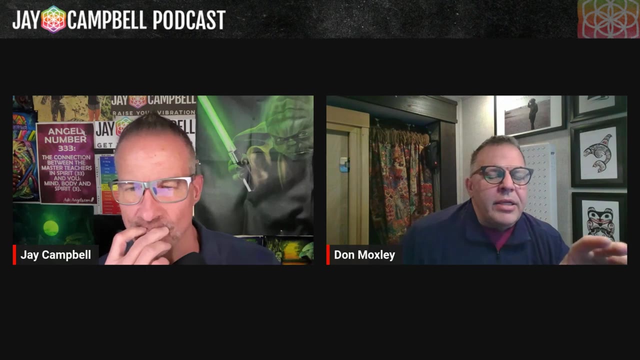 of applied science for a, a cannabis company in florida. so you, i don't know if you've seen the grow healthy stores, though we opened that company and my job was to go down and build a medical brand in cannabis, which meant i needed to understand cannabis. yeah, and and and, jay, i don't know if you've- if you've crossed this veil. 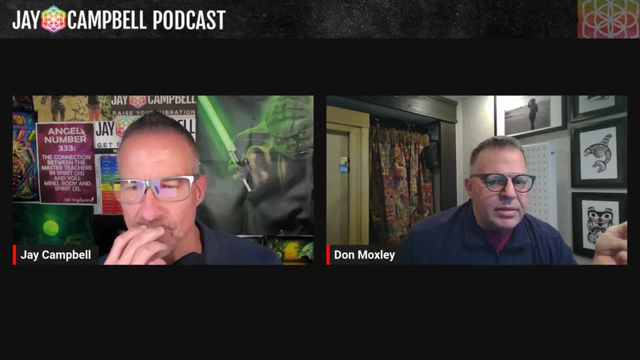 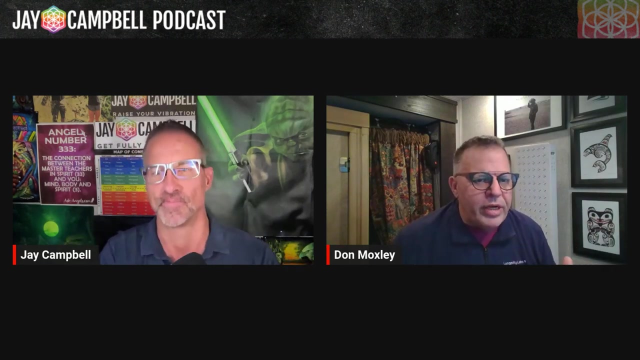 but when you move into the cannabis business, the amount of information that is available is overwhelming. i mean, there is so much good science. anyone who says cannabis does not have research has not bothered to open their eyes. yeah, um, the research is, is is tremendous. there are volumes and volumes of volumes of great research. 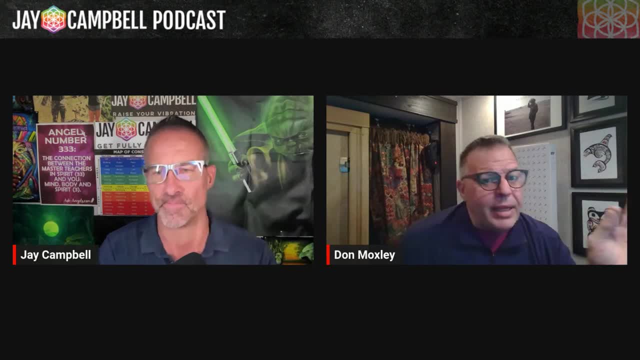 on cannabis. you've got to understand. it's not about thc, right? okay, beginning end of story. and and what was funny, i'm down in palm beach at the breakers at a medical conference and and it's this florida pain management conference. and um, this, this jamaican medical assistant walks over. 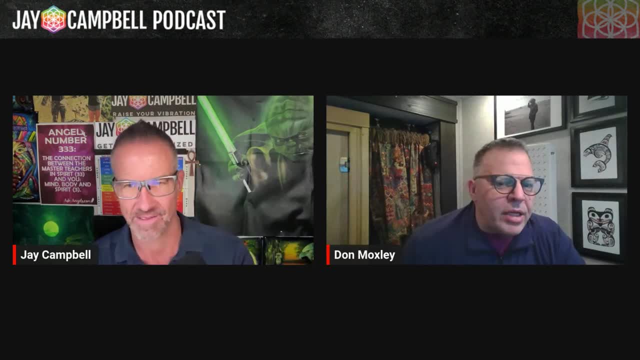 to me and she says: you know, we used to grow this in our backyard, yeah, and? and i said, and i said: really, tell me more about this. she says my father would take it and he would soak it in our finest rum. and i'm like: oh, that's. 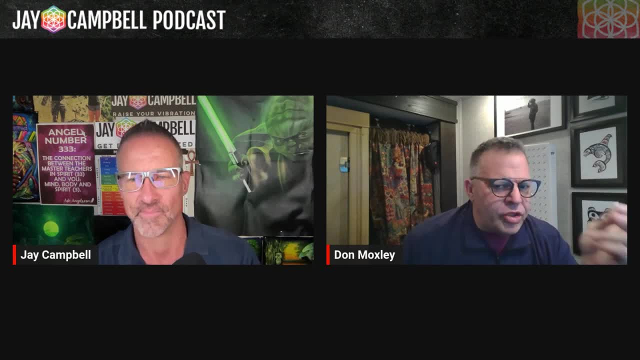 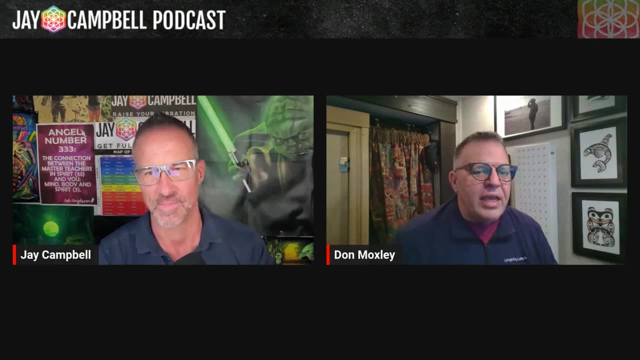 interesting, and not just rum, not just junk rum, his finest rum, right. and he said, when i would have a minstrel cram, they would give me a shot of this in my orange juice and it would take care of it. my father would come home and he would rub this on his knees, and he would rub this on his knees and 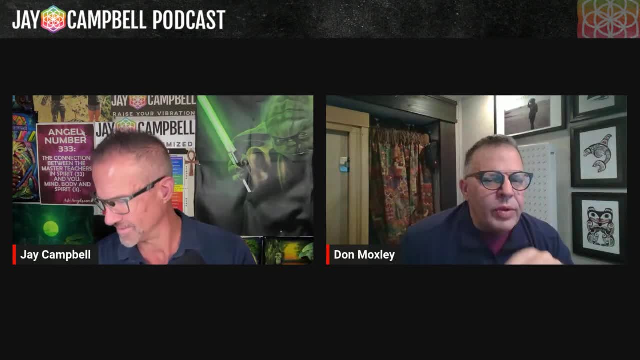 after he worked in the fields and it would relieve his pain and i thought, okay, there's something. i really want to understand this. so there's a way to extract terpenes and cannabinoids from cannabis is called ethanol-based extraction. that's what. that's what they were doing with the. 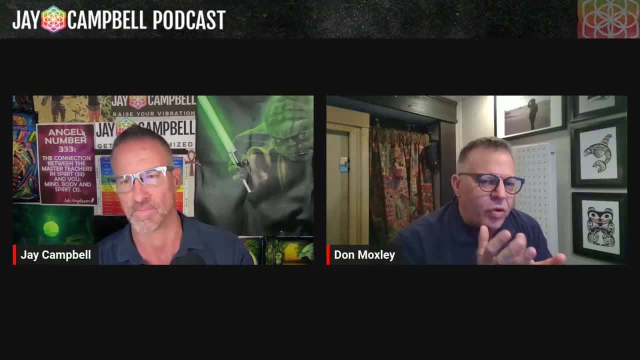 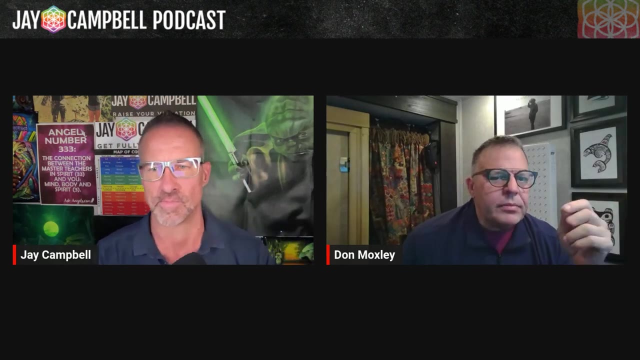 alcohol, it keeps the acid form of the molecule intact. so so thc stayed thca, cbd stayed cbda, and anyone who is in who has looked at cannabis has seen this thing called cbd. yeah, cbd was essentially junk. it was essentially a, a disposal product from the cannabis industry. 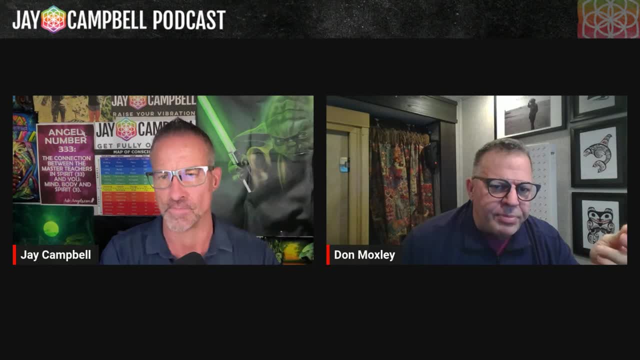 but along the way, some folks working with epilepsy figured out that cbd helped my kid have less epileptic seizures. so all of a sudden, cbd starts to get some value. well, you look at this long enough and when you look at it you're like, oh my god, i'm gonna die, i'm gonna die. 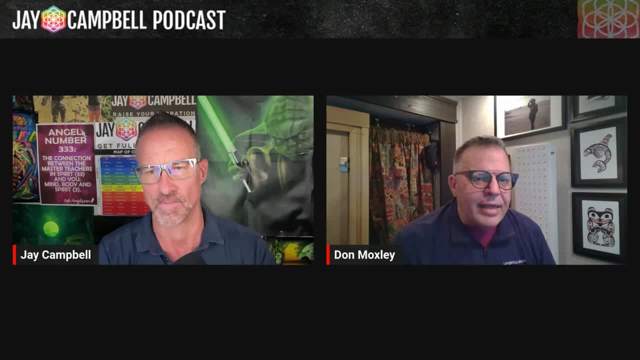 but you find it's not the cbd, it's the cbda, it's the acid form of, it's the original form. this hangs on a bunch of different, on a bunch of different receptors. so when you start to dig into cannabis and understand it, you start to see: okay, there is. 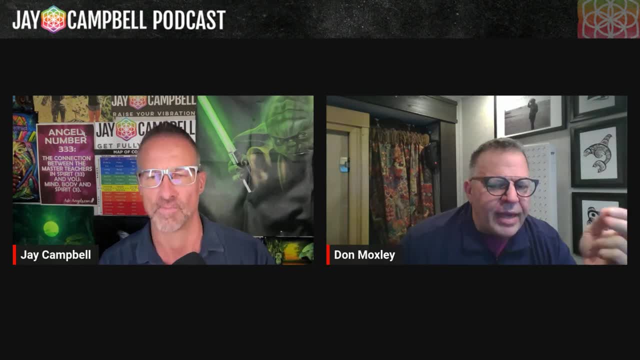 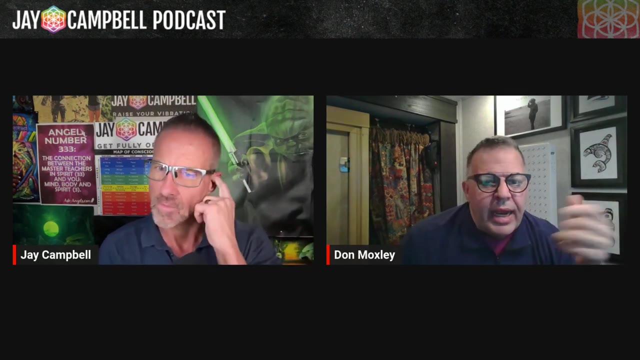 a pain relieving effect, there is an inflammatory relieving effect. the number one thing that drives poor hrv is inflammation. right, that's what drive and, and we all know the inflammation issues that we deal with, um, so, so that's, that's kind of the long story, and then, and then i get one of the guys i worked. 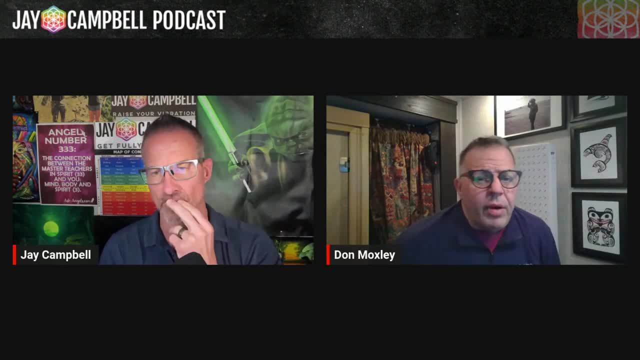 with down there in florida calls me one day and says: what are you doing? so i'm looking for a project? he says: well, i'm working with this company called longevity. flagship product that we launched, uh back in 20, was a product called spermidine life. yeah, spermidine's a molecule in the autophagy. 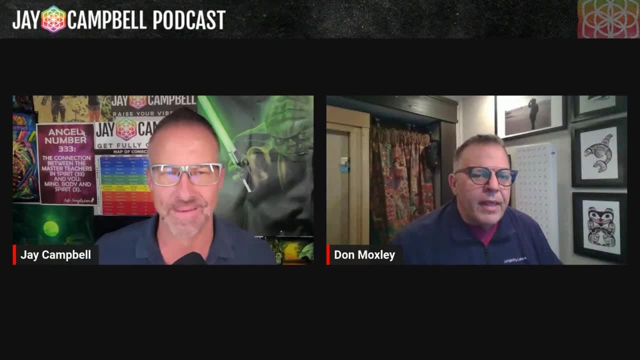 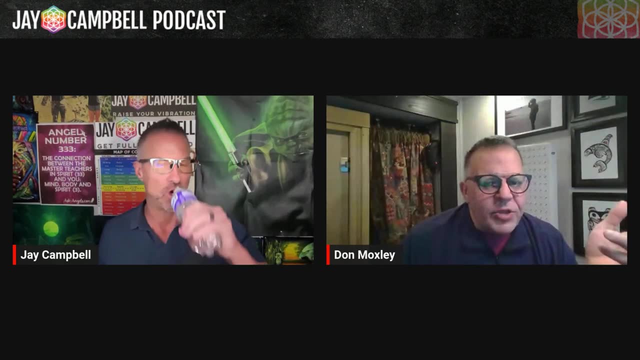 pathway and that's a whole nother podcast. but, um, i use spermidine, yeah, and then, along the way, what was interesting, jay, was, um, uh, dave asprey featured one of our doctors on his podcast and we blew up. okay, it was one of the best things that happened to us, but what we found, so i, i would. 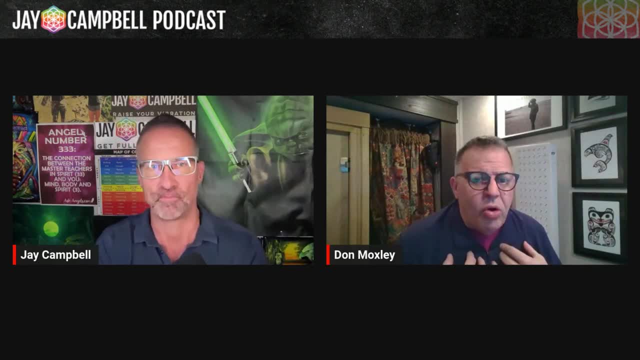 have. when you purchased the product, you got an invitation to have a phone call with me. um, so i wound up speaking directly to probably 500 of our first 700 customers, and asprey at the time was an advisor to aura ring. everyone had a phone call with me. and i had a phone call with him and he said: 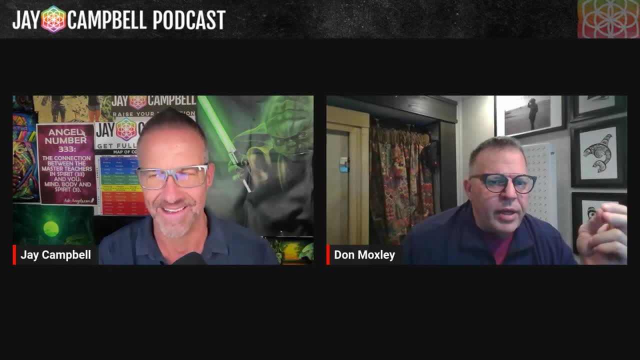 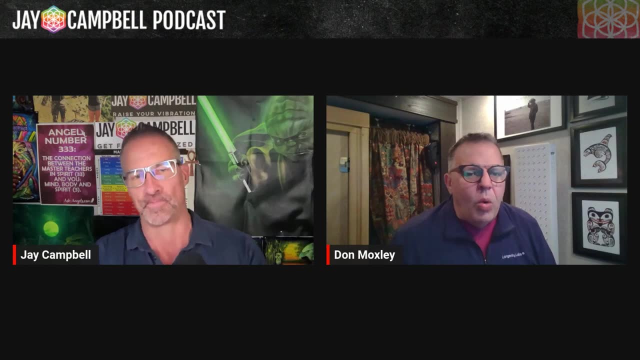 an aura ring. No one knew what the hell to do with it. Um, you know, so we've got this parameter, this HRV parameter, out there that people are starting to pay attention to, but no one knew how to manage it. Um, so they came to me and said: can we make a, can we make a supplement? 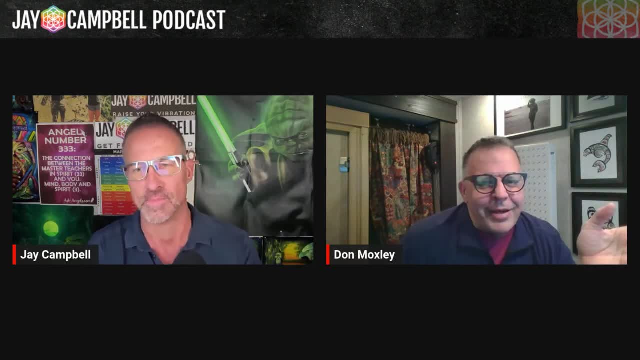 I said I've already made it. You know my apartment in. I was in North Palm beach And when he walked into this little one bedroom apartment I had, my kitchen looked like breaking bat gram scales and beakers and all that I was. I was figuring this stuff out, Um. 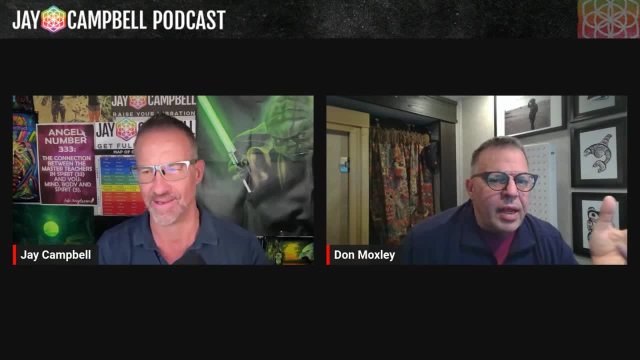 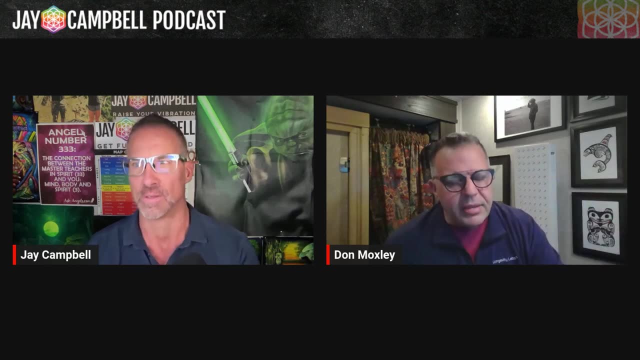 and I developed. I developed a combination, um, and several people were using it And I said I've already got it, So that's where our product is called HRV plus came from. It was that experience of understanding that that drove us into the development of the product. 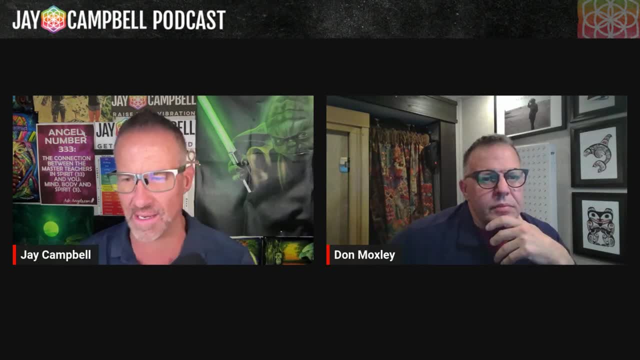 That's awesome. Um, just a couple of things, a couple more talking points. Um, I mean, I kind of know the answer to this, but I'm interested in your answer. Um, who shouldn't be concerned with heart rate variability? 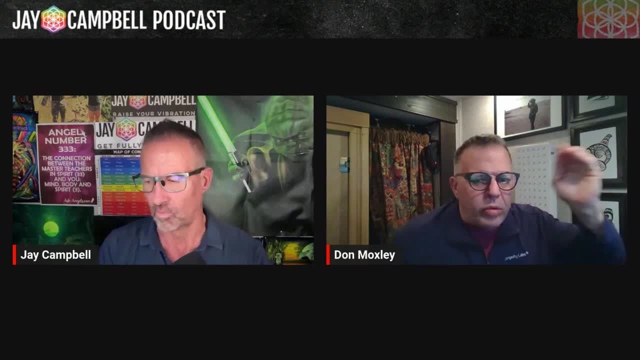 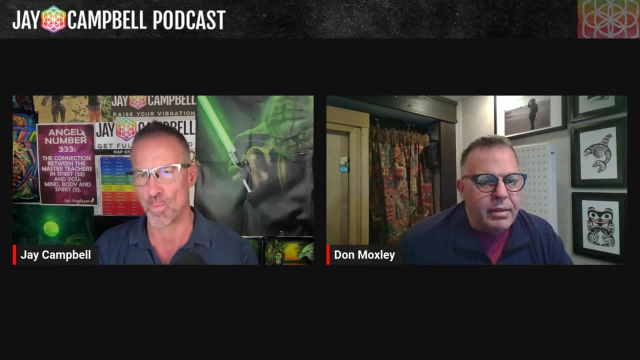 Listen, here's what we know. My Olympic gold medalists have the highest HRV we've ever measured. The minute before you die, your HRV will be zero. So you have a range. You want to move away from zero as much as you can. Okay, Um, because as you're moving towards, 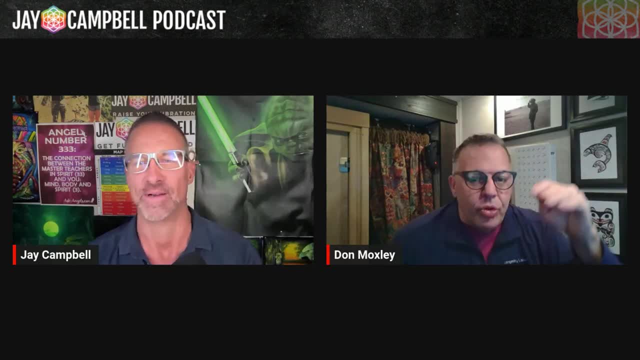 zero, you're moving towards death. Um, and as you move your HRV up, you're recovering better. You have better resilience. You have these. I believe that HRV will become the KPI I. you know it's going to take time. The technology has got to get better. Listen, my daughter just graduated. 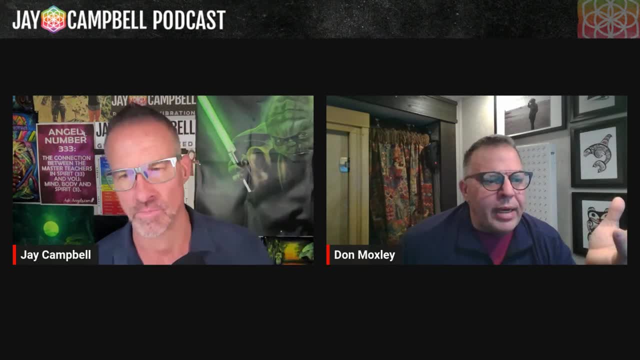 from Ohio state with a degree in um exercise science in 20, 2020.. Yep, They still were not teaching HRV in the exercise phys classes there yet. Okay, And I cannot do exercise prescription and management without having HRV data. It is not. 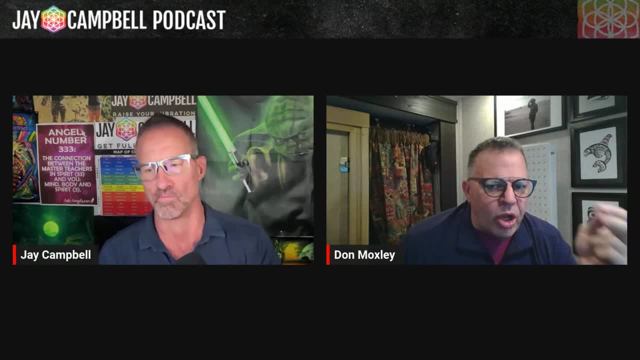 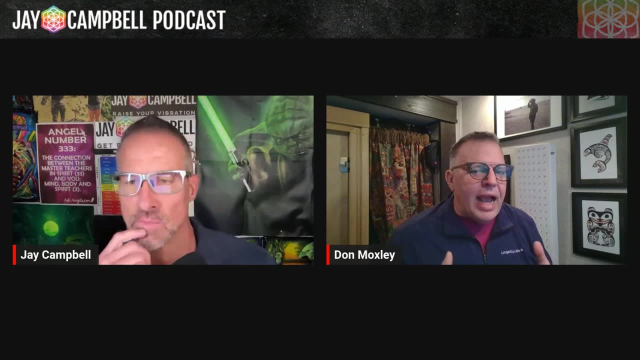 do it You. you do not have valid results if you're not doing that. So so when you start talking about what is the KPI- KPI that I can associate with improved health span, lifespan that I can associate with improved performance- it's, it's HRV, and HRV is more than a single. 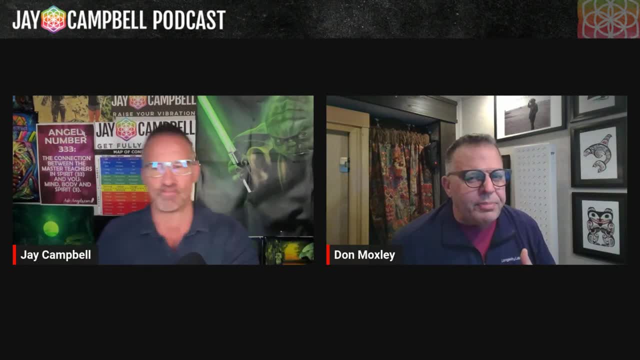 number. When you start to dive into it, it can become a fairly complex concept. Um, I talked to I. I worked with several wearable companies discussing this. you know aura did a great job of popularizing the RMSSD and sleep scores and things like that. There are underlying data. 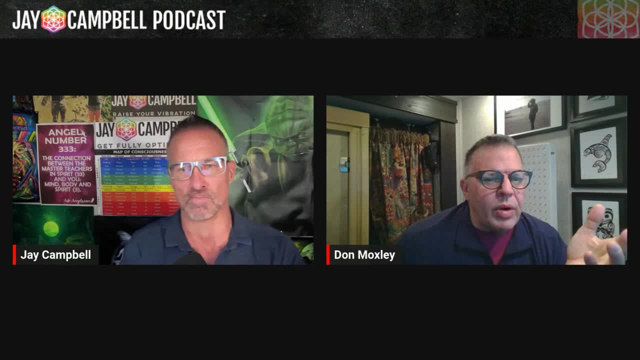 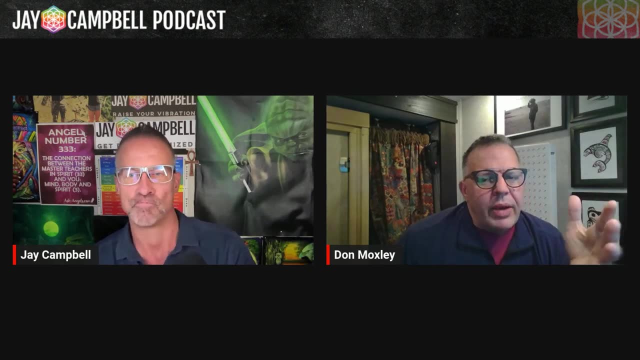 points that I look for that I can't get from aura, So when I start working with someone, I usually bring other technology into play. Um, uh, so I work. there are two measurements that I live on. That's called LFHF- low frequency, high frequency- So 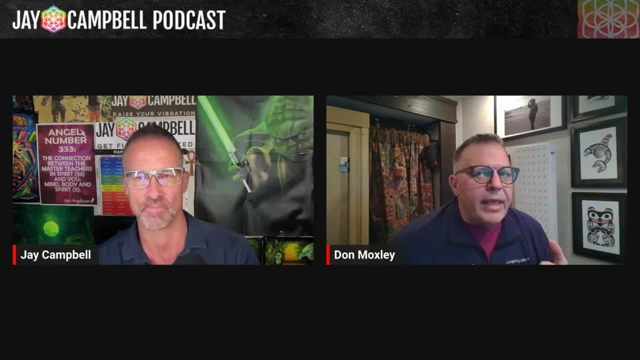 so, so low frequency is your um is your sympathetic drive- Yeah. High frequency is your parasympathetic drive- Yeah. So you want your parasympathetic greater than your sympathetic. Let me put this into perspective. My Olympic gold medalist, Kyle Snyder. 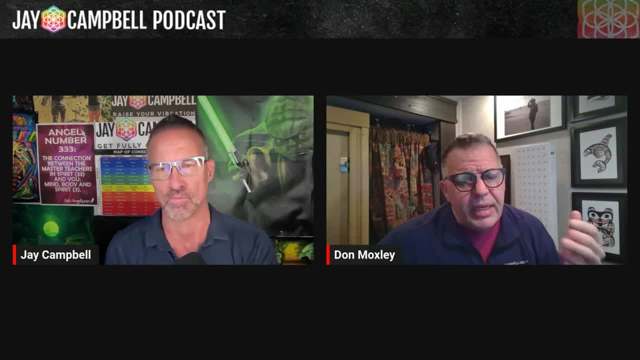 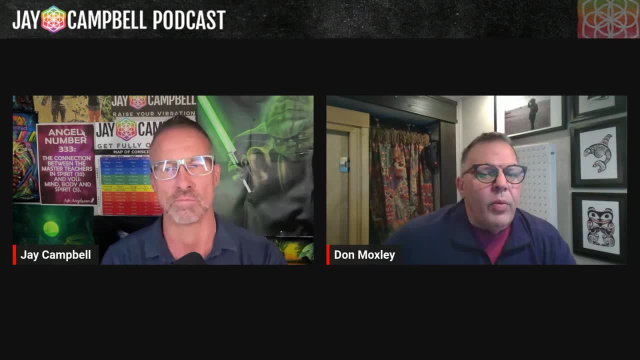 a hundred and twenty-five milliseconds overnight. regularly We go to he's wrestling up at the university of Michigan And the guy from Michigan had red shirted the previous year but he was also a world champion in wrestling, very talented. And this guy cut weight to make two 75. Um. 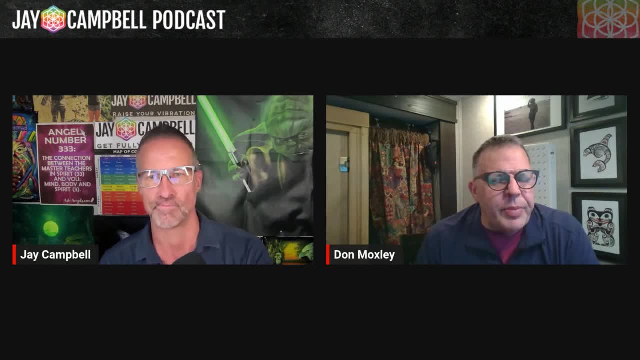 Kyle wrestled 90,, uh 97 kilograms, which means he walked around our room at about two 30. Most days, Um this guy's cutting weight to two 70. So is it So I? I do all my morning measurements with the team up in the Ann Arbor- I get the lowest HRV score. 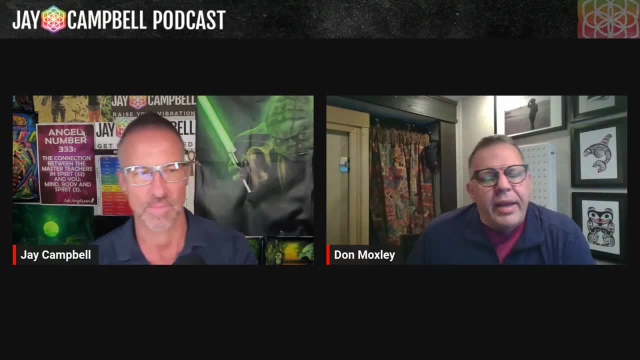 I've ever had with Kyle the entire time, Um. now my language to my guys was: everything looks good, You're ready to go? Good job, Go get them, Okay, Because I couldn't fix anything day out. you know, by that time the, the die, is pretty much cast Um. so if he loses that Domi, um, it's the. 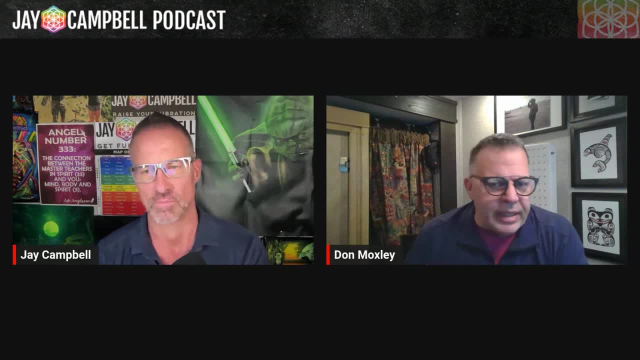 first match he's lost in three years- international NCAA anything. And I get him back to Columbus and I said: Kyle, tell me about what you were feeling in that match. And again I asked the stupidest effing question that day. I said: were you, was there? fear, Never ask a 20 year old Olympic gold. 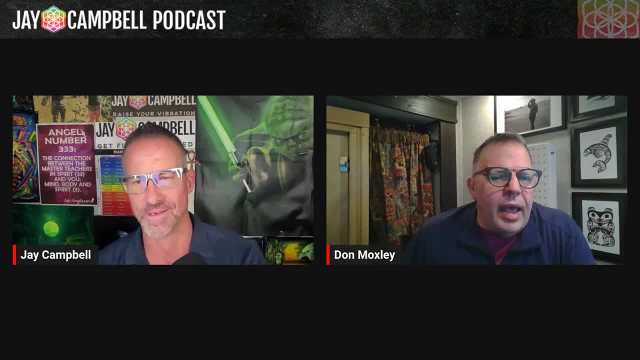 medalist if he's fearful, because the answer will be no, Of course. And um, and so I thought, okay, stupid question. But then I said, well, let me show you what I saw in your data And what I saw. 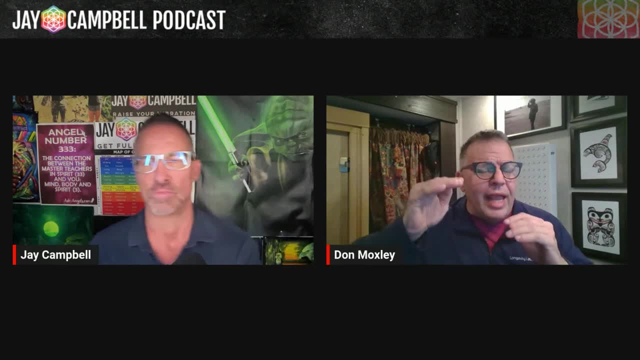 was an LA F, H, F. that was way out of balance, where I like to see that number below one. I want the. I want the dividend greater than the. I want the uh. I want the lower number greater than the um the first. 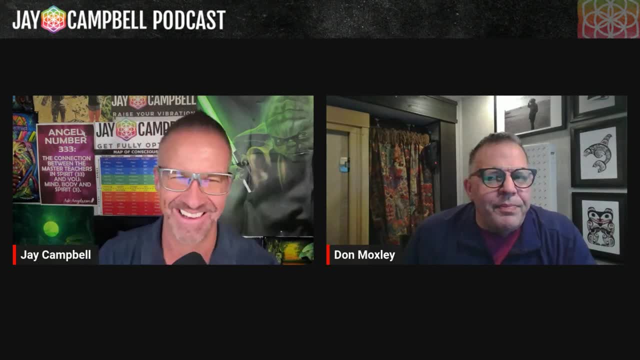 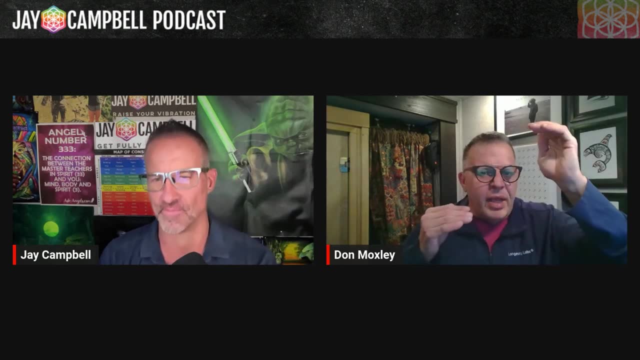 I'm blanking on what those are- Um but um, and and his was 20.. Okay, He had huge sympathetic drive and very poor parasympathetic at the time, So he kind of he goes. what do we do about it? 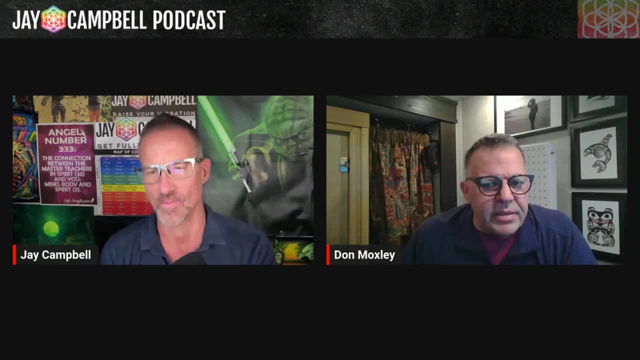 So I hand him a uh uh brain, um, a heart math device, Um, and heart math is a company that you use. It's a, it's a bio. it's a bio feedback meditation tool that gamifies meditation. Yeah, And you give this to a 20 year. 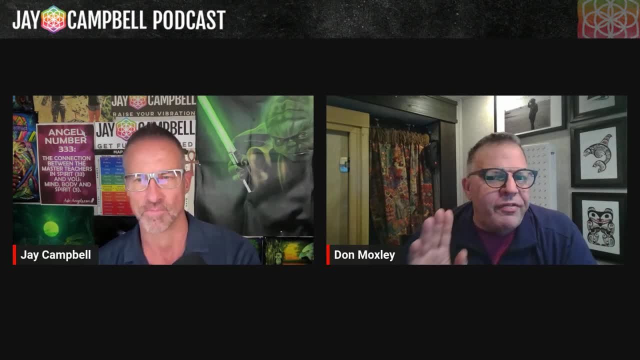 old. and all of a sudden they're gamifying meditation. They go off the edge. He went nuts with it. Um, and all of a sudden his scores man, his drive. So he wrestled, he wrestled this kid. Adam couldn't two more times. big 10 finals, national finals. 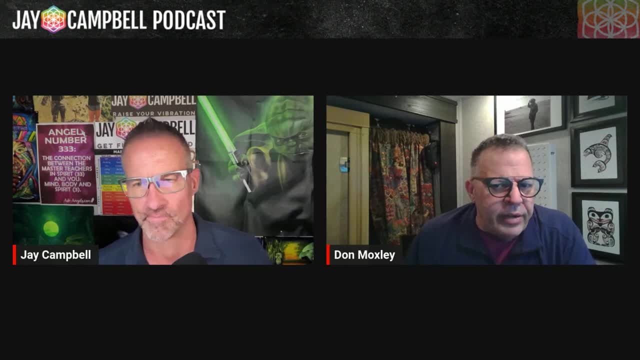 uh, beat him both times. We never went into any of those matches with an LF grade, F, LFHF greater than two. Now, he still had high sympathetic drive, but we were able to boost parasympathetic with that in order to get this kid in balance to getting in And and and. so he had the 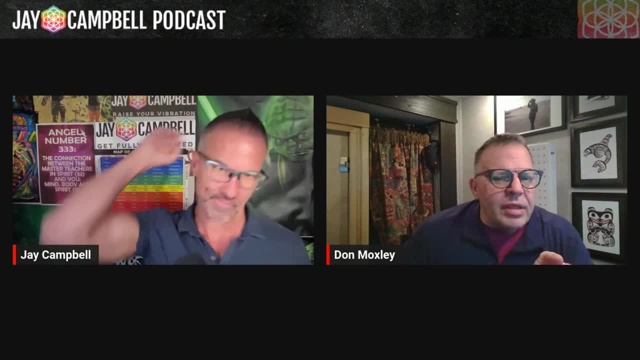 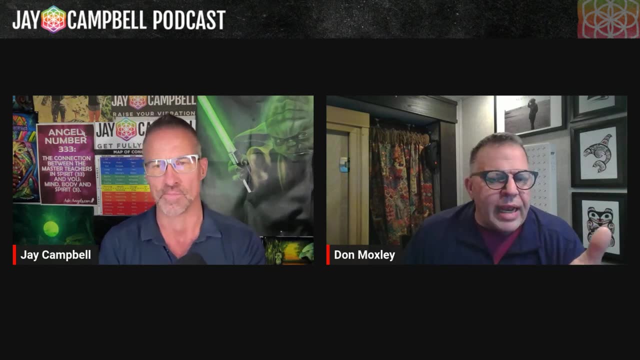 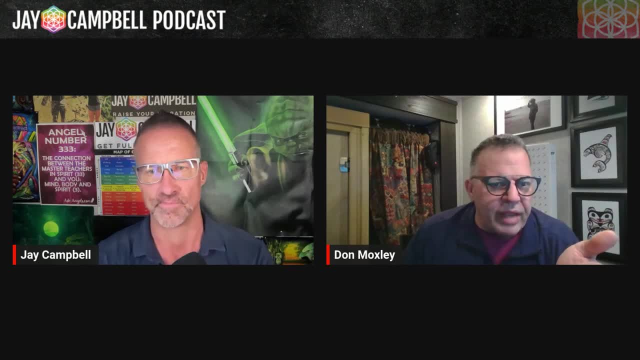 workouts, heart rate files. I see the heart rate graph over your shoulder. I think that's what it is. Um, you know, I want to see the buckets that you're training in. Okay, This is not a heart rate graph, Um, but um. but when we look at that, I want to see. I want to see: are you creating? 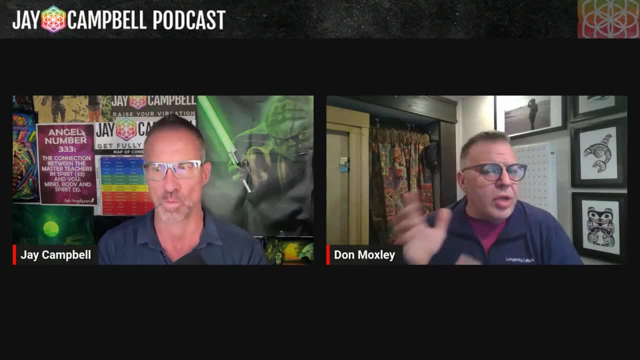 cortisol unnecessarily. Okay Cause cortisol. listen, if you're training and you're leaving puddles of sweat and you're- uh, I'm, you know, listen, I like cry. I have very good friends who CrossFit. I have very good friends who spin both. both systems are a thousand. 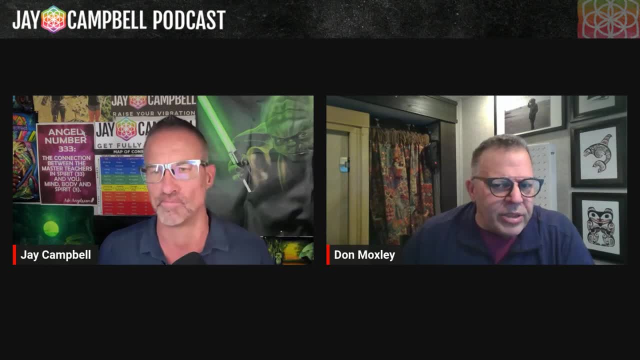 ways to keep you at max Um, which is rarely the best way to train Right Um, but I want to. I want to. I want to train the system to go in and out of max down to recovery with using intervals. So I want to see your heart rate data. I want to see if you're just living up there. 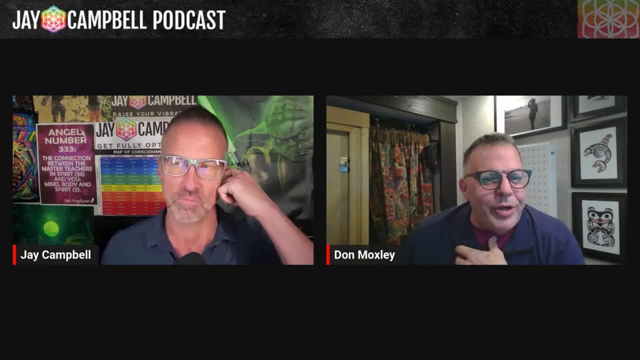 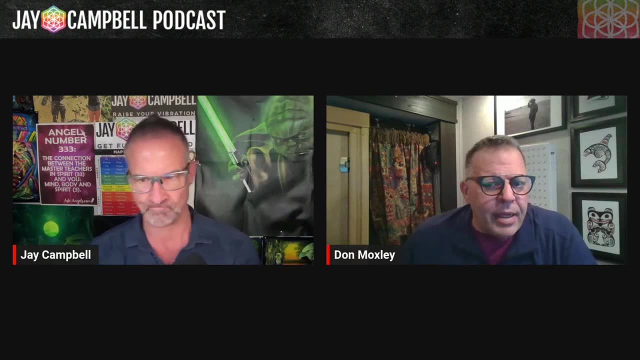 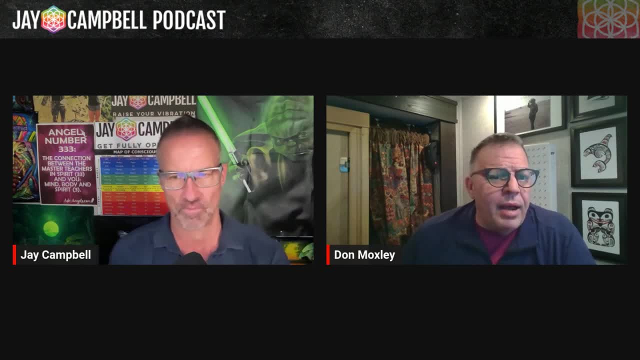 try and make you as happy as you can so you can get away. Um, you know that's, that's the evolutionary aspect of this, but but at the same time, that may not be the best way. You know, when we finish working out, we need to go into recovery. Well, if you finish your workout and 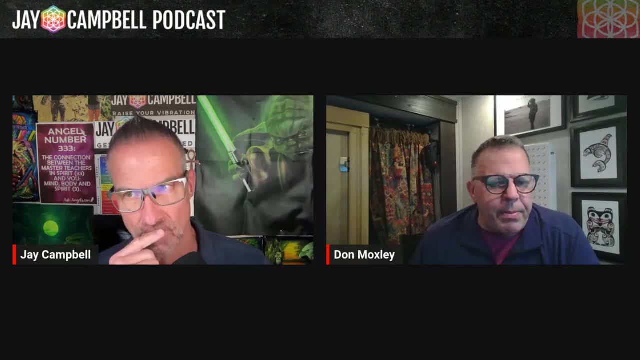 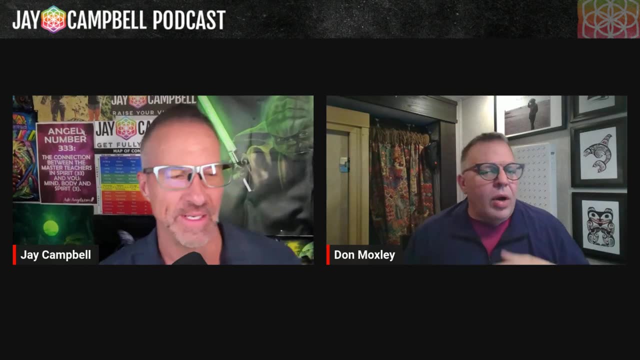 you grab your phone and you're getting agitated by a text you got from your mate or from work or something like that, and you're not able to separate The sympathetic stimulus. or if when you're driving home on Dale Mabry and someone cuts you. 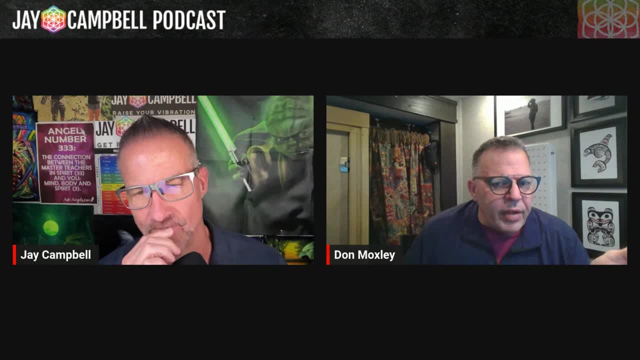 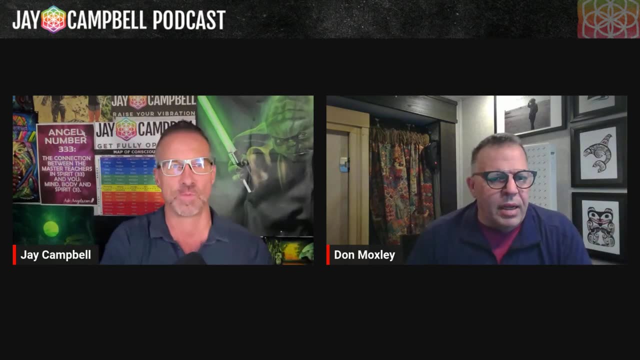 off and you, you go into rage. you've got to learn that, all of a sudden, all that work that you just did, you're, you're continuing to devalue it. Um, you're continuing to devalue it, And that's why. 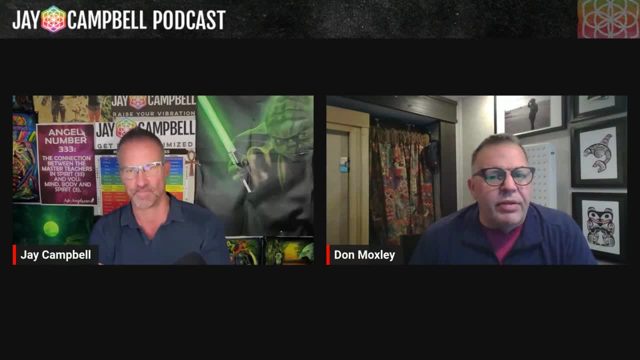 listen, I, I, I don't think you train without a heart rate monitor. I don't think you sleep without an HRV monitor of some kind so that you can see that nighttime resting heart rate. You see that nighttime resting HRV. Um, those are, those are KPIs that I pay close attention. 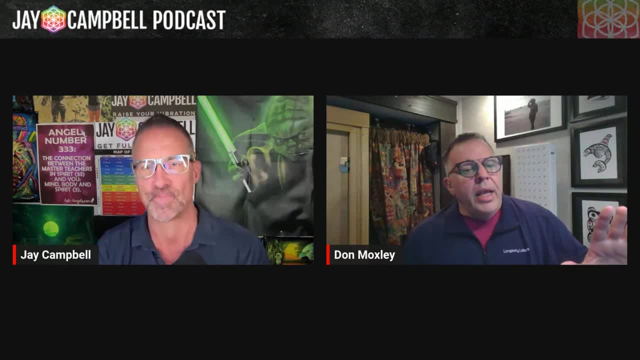 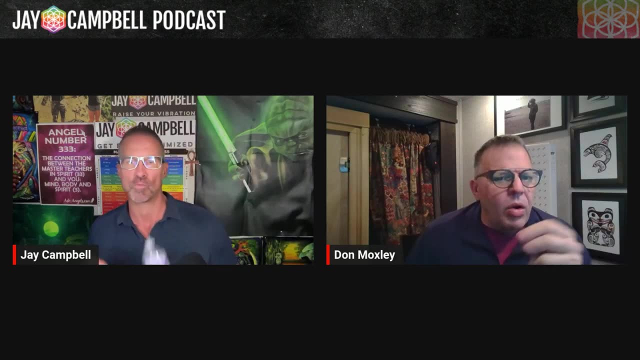 What do you think of the eight sleep mattress? That's what I, that's what we use. Yeah, Listen, I think I think there's tons of there's tons. I think it's on eight sleep or any other manufacturer to be able to demonstrate that their assessment technology. 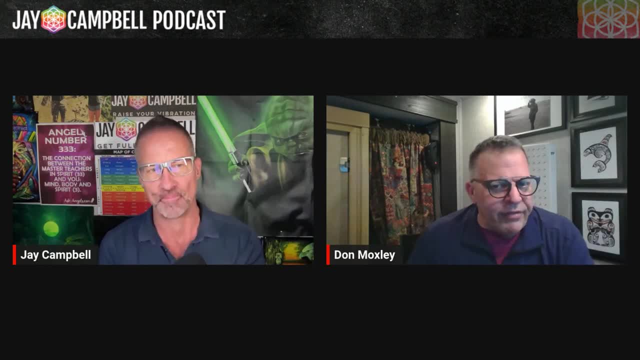 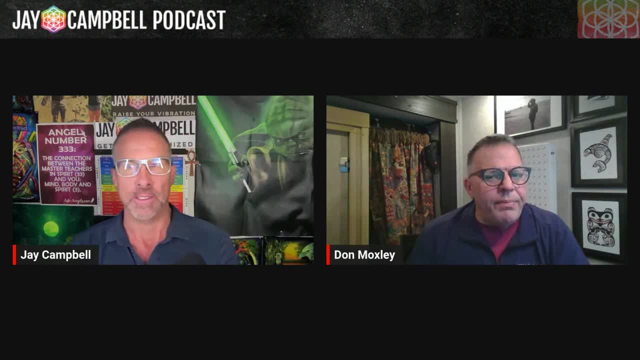 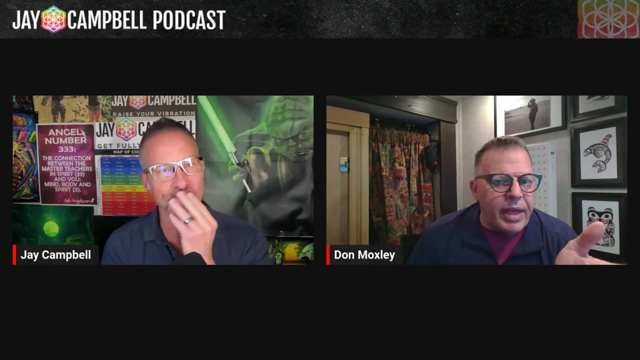 so I don't know. I do have, um, we do have the inflatable mattresses. uh, that that will give me an HRV score. It's not as good as my good wearable device, Um, I good wearable device, And the other problem with it is that there's someone in bed with me, Um, so there's, there's. 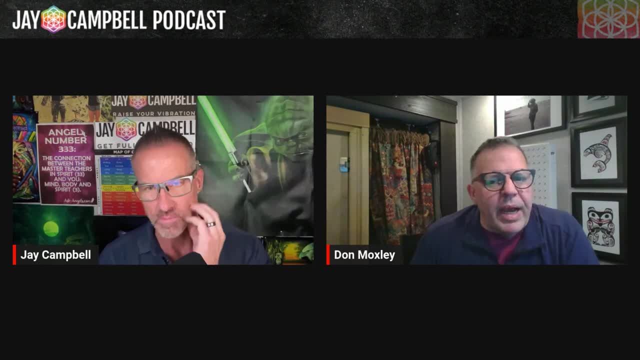 going to be issues there, but, um, but it's on them. but I do absolutely believe in the modality of maintaining a bed temperature that's consistent, And but I don't think. but, as we talked about before we started recording, you know a good friend of mine, Molly McLaughlin, um has a 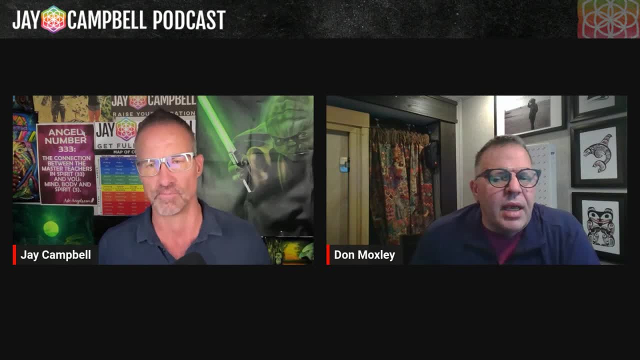 podcast called sleep as a skill, And we have a lot of conversations about this. Um I, personally, my HRV, drops if I'm too cold in bed. Um so I- my bed is typically pretty warm and snuggly to get my best scores. Um so. 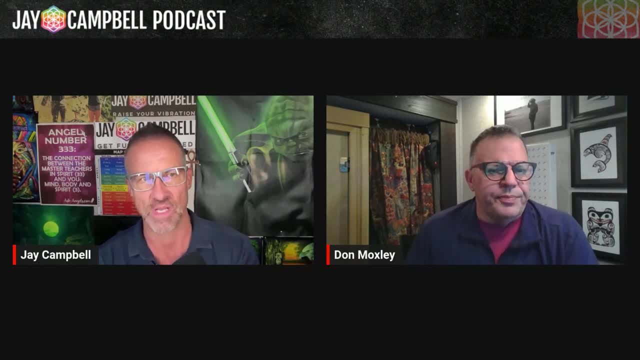 I think. I think it changes from person to person and you got to develop an awareness of this. Yeah, I'm the. I'm different. Uh, my, my HRV is much better when I'm sleeping cold. I sleep more soundly when it's colder. It doesn't have to be like hibernation cold, Right, But you know. 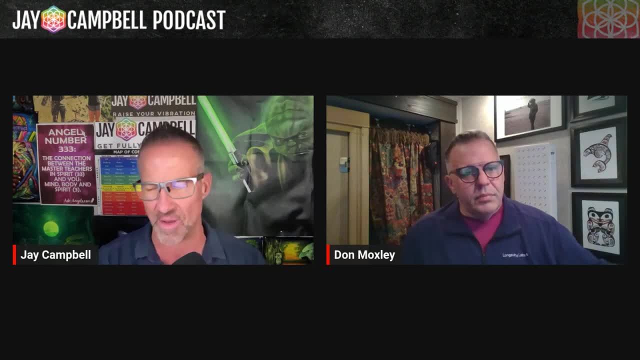 the eight sleep offers both sides. and you know my wife is perimenopausal, Um, and so she, you know is will experience, like you know, warmer. you know not really technically hot flashes, but she definitely sleep warmer. Uh, but it's interesting, Um, just before. 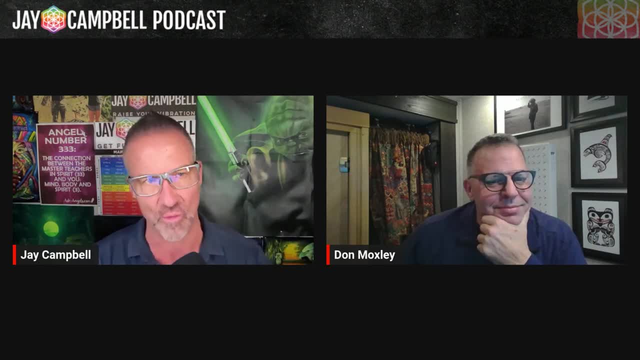 before I let you go, man, just a couple of simple things people can do to obviously improve important performance. You got to measure it. You can't manage anything that you're not measuring right now. Yeah, But, but Mark Twain said no. Einstein said that just because you can't measure. 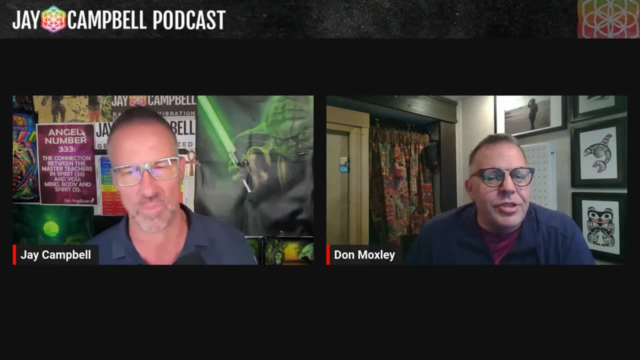 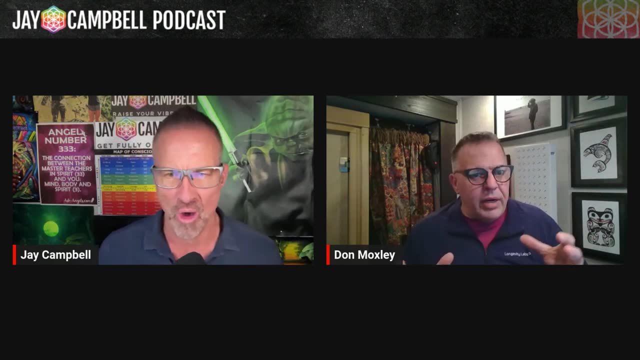 it doesn't make it important. just because you can measure it Doesn't make it important. So you got to make sure you're looking at it. but we're seeing the emergence of this. But if you want to improve performance, you go back to those big rocks. Okay, Movement nutritious. 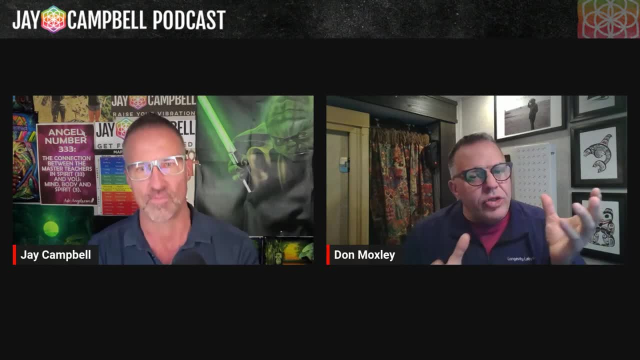 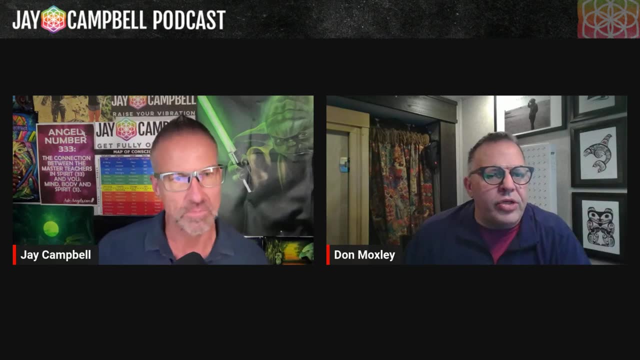 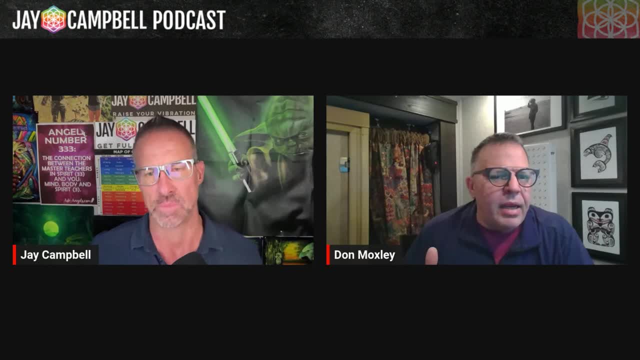 a mistake to wake up every morning, look at your HRV and say, um oh, this is what I'm going to do today. You need a goal out there on the horizon and then you track HRV to make sure you're moving. 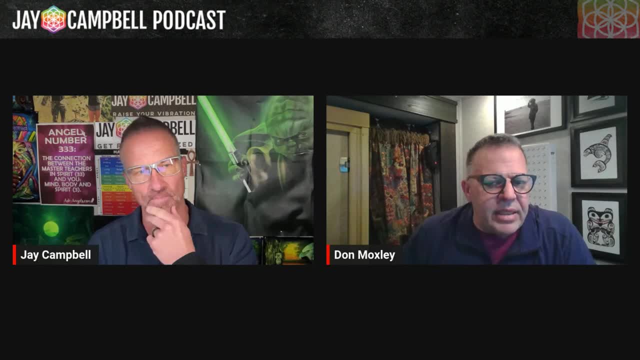 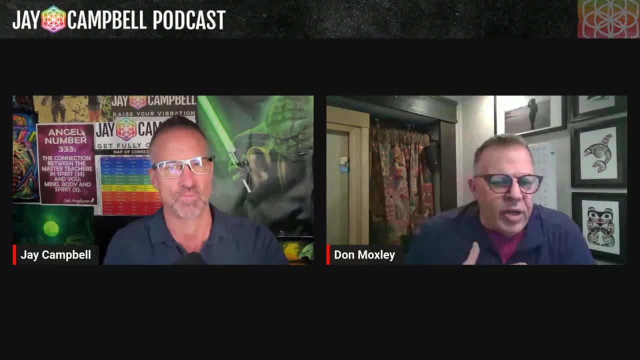 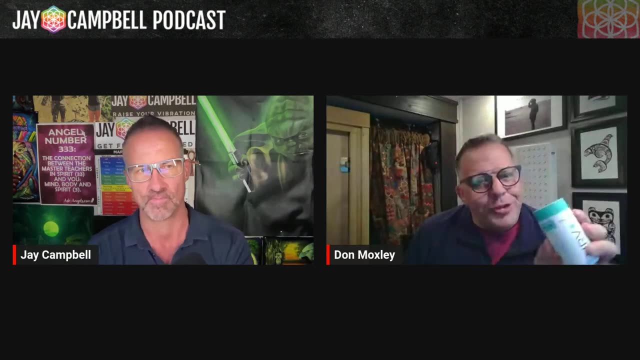 all contribute to this. Don't get caught up. Listen. if you're not sleeping well, HRV plus is not going to do a great job for you, Okay, But if you use HR, the one of the nice things about HRV- 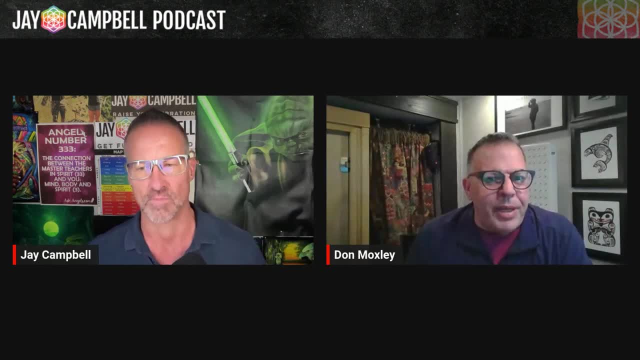 plus is that it's improved the sleep of most of the people that take it. This is what this is. one of the things they talk about is what great sleep they're getting. And again, that endocannabinoid system. part of your nervous system is called the endocannabinoid system. If you don't have the 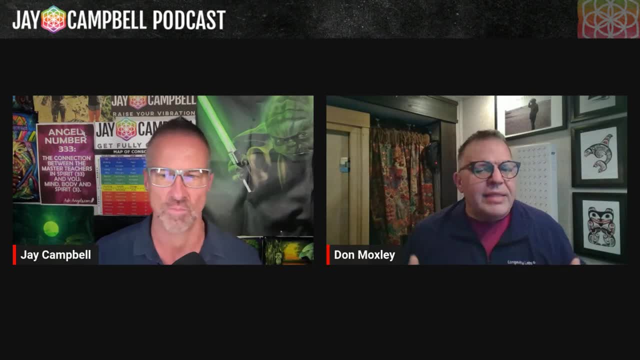 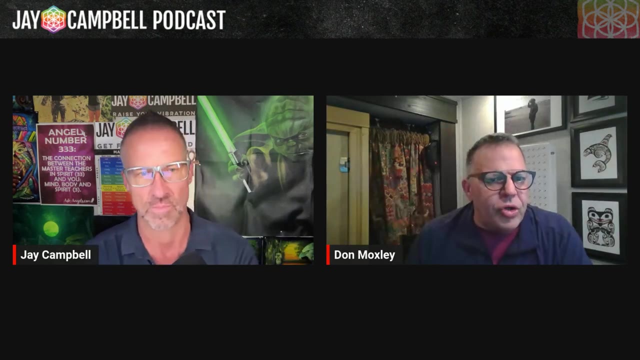 necessary underlying nutrients to support that system. that system's not going to function correctly. That's why we put the CBDA, the beta-caryophyllene, in this. but then we've gone ahead and balanced this, Jay We. it's carried in an omega-3 fish oil, DHA, EPA, fish oil that has 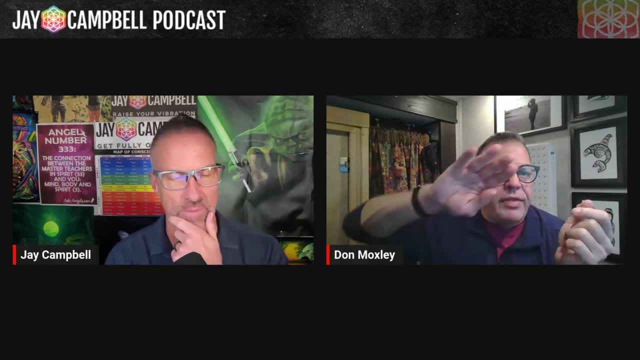 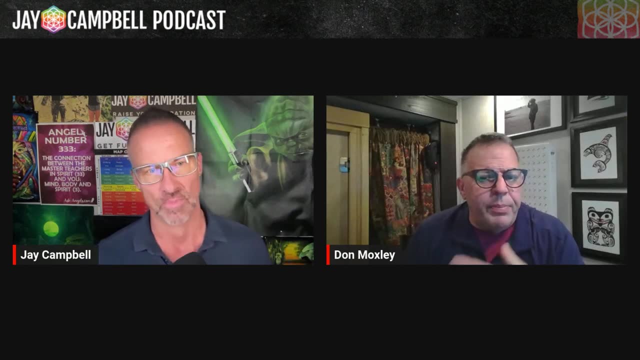 what's called SPM, specialized pro-resolving mediators. These are the final stage of the inflammatory process that clean the cell. But and we found a lab in Spain that we could put these SPM, So they're all in that one combination. So the the second rock nutrient, dense food. you hack with supplements. This is a supplement. This is a supplement that you can use to help balance that, particularly with the omega-3s and the SPMs. But we then we throw the, the CBDA and the beta-caryophyllene in on top of that. 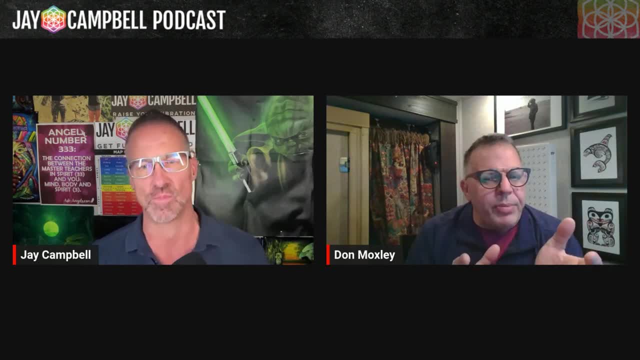 Um, but yeah. so going back to your original question, what can people do? Pay attention to the rocks. Are you moving? Are you hack it with exercise? Are you getting nutrient dense food? Look at all the nutrients Again. spermidine is a nutrient. we didn't know was a nutrient until about. 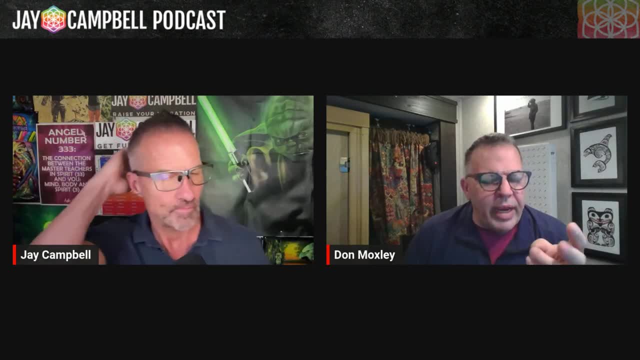 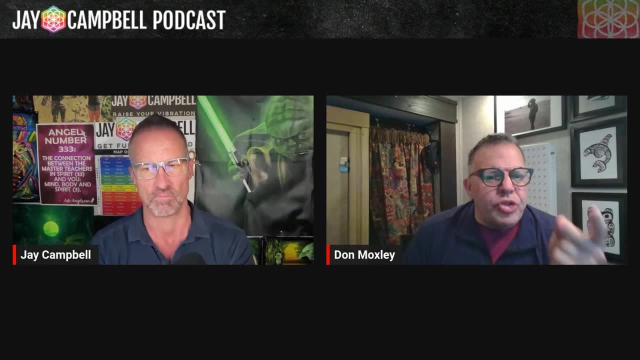 10 years ago and we're just starting to really understand it. So it could be something that you don't understand, that we don't know yet, that you got to pay attention to. Um, you have to sleep. We'd been on the West coast. 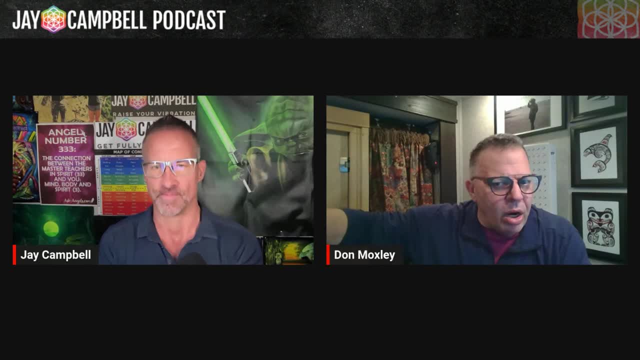 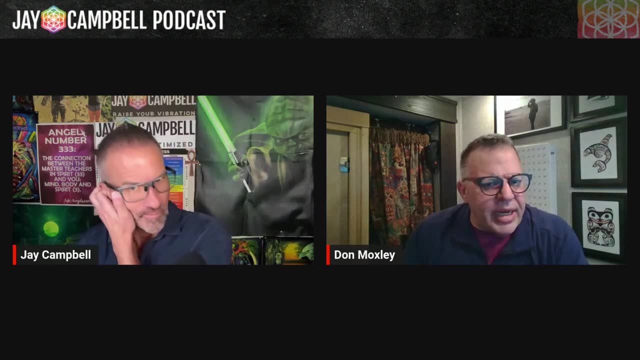 uh, for a year. Okay, So our body clocks are on Pacific time, but we're now in the Eastern time zone And my wife is. she's sleeping till like 10 o'clock and she, she kind of gets upset about it. 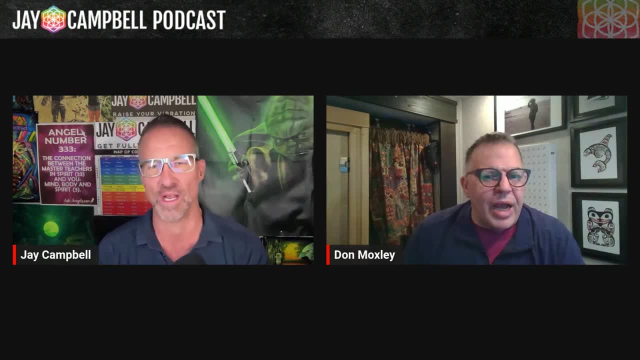 I go: no, no, no, no, just sleep. Okay, Let your body take care of it, It'll adjust. Um, yeah, So pay it And, and, and. this idea that I don't sleep, therefore I'm more effective is bullshit. 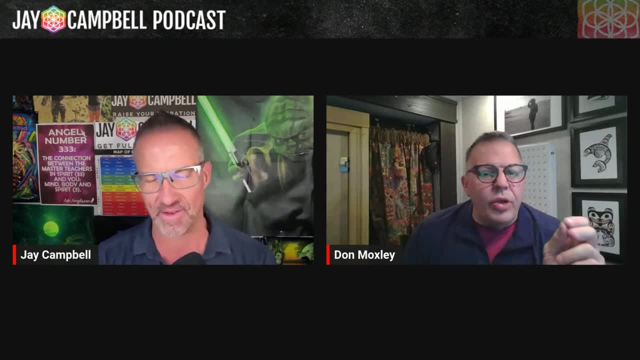 Um, that's complete. You cannot hack sleep Anybody who thinks that you cannot have a sleep environment. you cannot hack sleep Um caffeine. caffeine does not equal sleep. Um and um and then and then finally light.